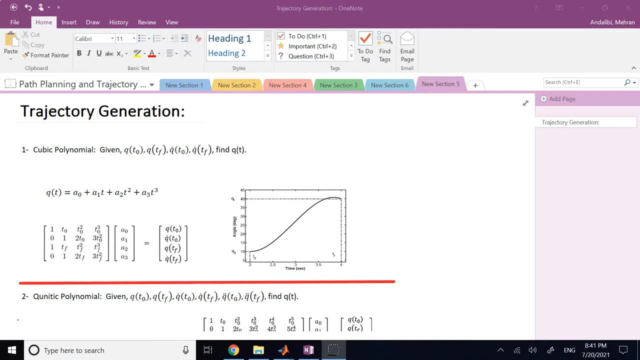 Hello everyone. As you know, the path planning was really a non-parametric identification of the path right. Basically what you did: you determined a bunch of waypoints and you tried to go from one waypoint to another and avoid collision. But you never specified in path planning that when you have Q values correct for each one of the waypoints, you have not specified how the Q, the joint variables, would change as a function of time from one waypoint to another right. 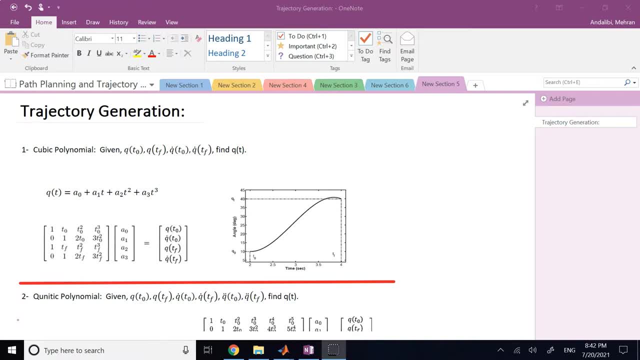 So all you have was the endpoints, just the endpoint Q, Q1 and Q2 or Q3.. Q0 and Q, final. That's all you had. How Q changes versus time, that was not discussed in path planning and that is the topic of trajectory generation. 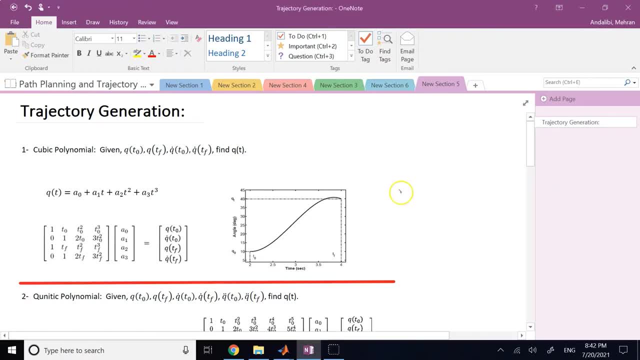 So in trajectory generation I want to find Q as a function of time. What kind of time function I should choose for Q if I only know the endpoints? And you might say why is that any important? Because if I am sure that the reason 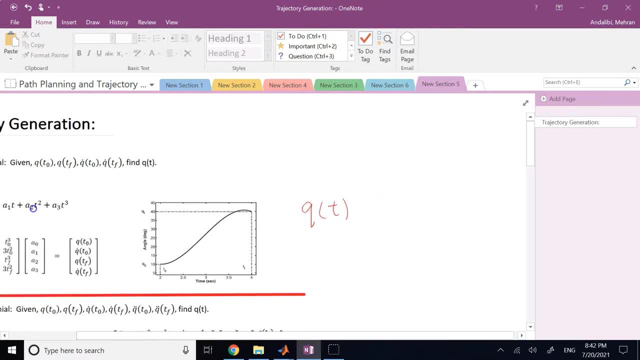 If there is no collision happening. what's the importance of Q? Well, you know, if, for example, Q corresponds to the angle of a joint right- Let's say it's a rotary joint- Then the time derivative of this Q is what Q dot, which is the angular velocity omega. 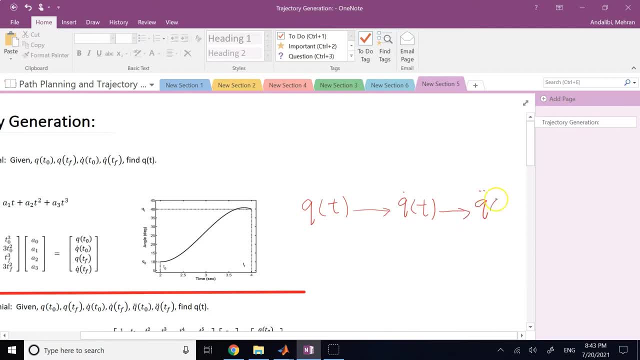 And then what? The time derivative of that is Q double dot, which is the angular acceleration or alpha, correct? And this angular acceleration Does depend on what, On the torque, correct? For example, you know, if it's theta double dot, theta double dot or alpha is equal to what? 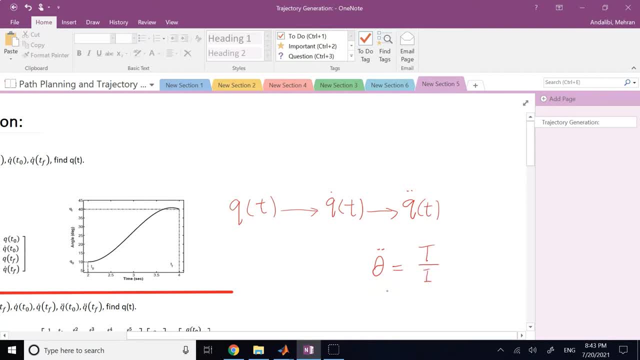 The torque divided by the mass moment of inertia, I right? Or if it's like the, It's a prismatic joint, then D double dot is equal to the force applied to the joint divided by the mass, correct, And you know. 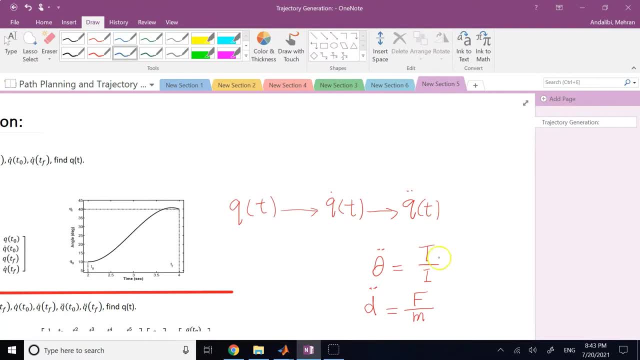 You have physical limitations on the amount of the torque that a motor can generate or the force that a linear actuator can generate. right, They have limitations, and so when you divide them by these numbers- I or M, your D or your theta double dots- they have some max values, correct? 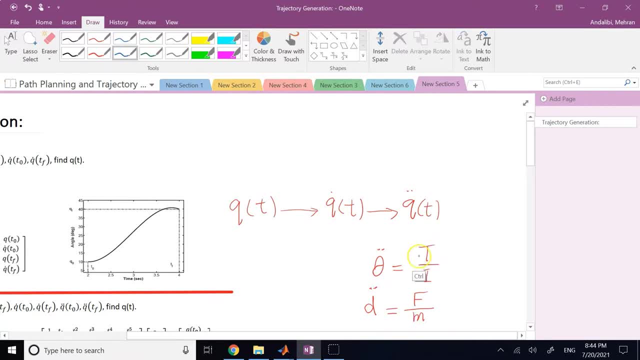 Alright. so if I write it like this, You have some maximum. This is like A, correct, This is like A and this is like alpha. There is some maximum acceleration and maximum what Linear or angular acceleration you can have, and also: 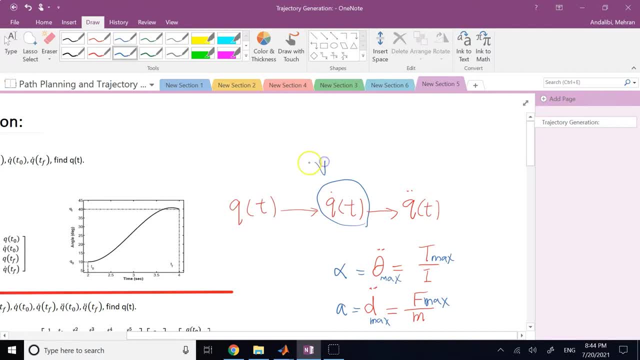 When you integrate those, this guy can be either linear velocity or what Angular velocity. This guy will only also have some maximum correct. You cannot expect from A motor to give you any RPM that you want and any torque that you want. 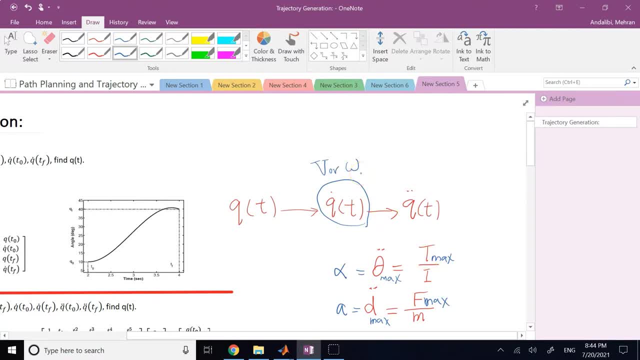 And you also know that the omega and torque, for example for a motor, they do depend on each other. right As the RPM goes up, the torque drops and vice versa. So you have limitations, physical limitations, on the driving force or the driving torque behind your joint. 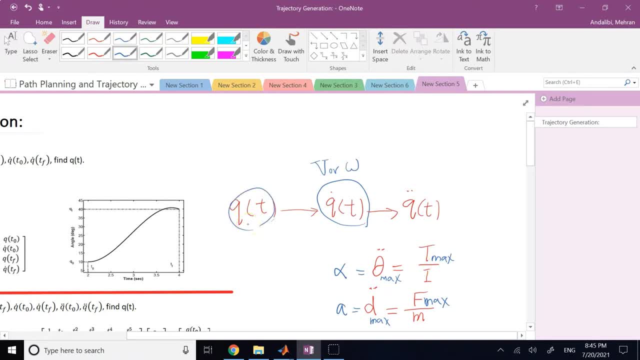 And that's why this function of Q does matter, Because if you choose this Q of T such that your angular acceleration, or linear acceleration, exceeds what the motor can give you, then your robot cannot achieve the task right The way that you want. 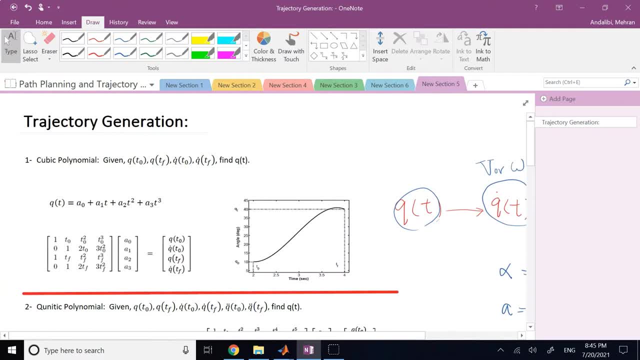 For example, let's say I want to go from my initial Q value and let's say T naught is zero or whatever, and TF is two seconds, And I want to go from initial Q of zero radians to final Q of, let's say, 400 radians. 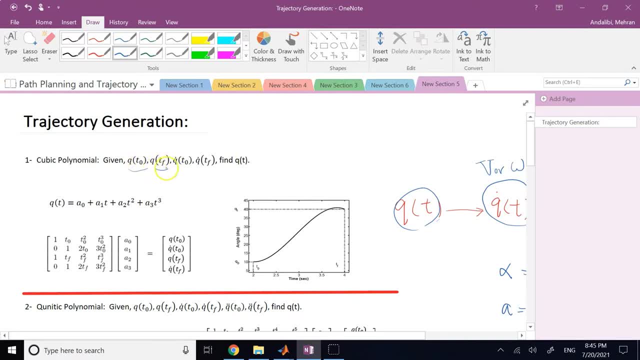 And the timing I have is from zero to two seconds. So in two seconds your joint has to rotate 400 radians, which is on average 200 radians per second. And if you multiply that by By By 60, over 2 pi, correct. 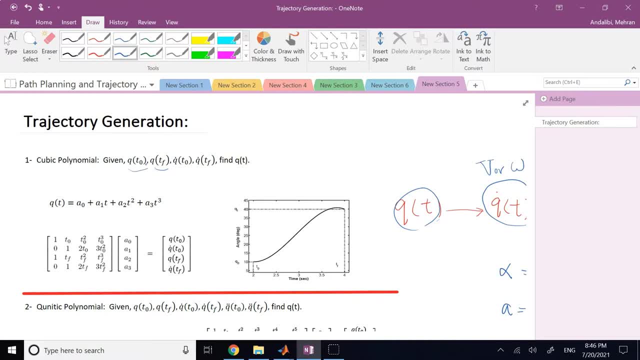 You can convert it into RPM 60 over 2 pi is roughly 10.. So 200 RPM means what? 200 radians per second means 2,000 RPM. Now, can your motor give you such RPM? Maybe, maybe not. 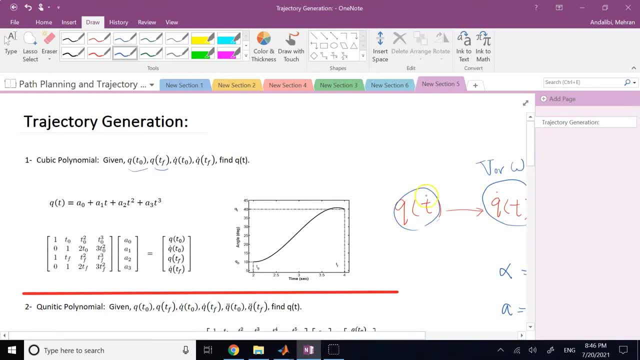 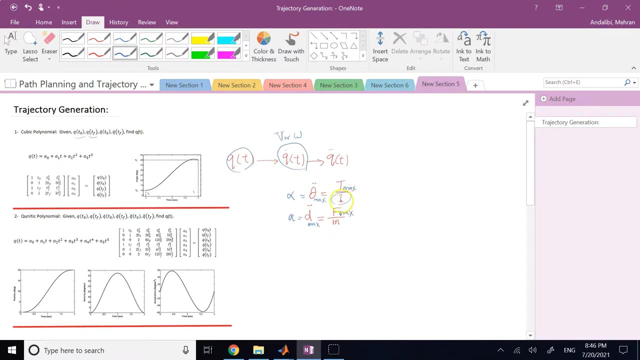 And also, when you calculate your acceleration, I'll show you angular acceleration. Maybe it shows that your maximum angular acceleration, based on the inertia of the motor, is going to be- and the load, of course, right. This is the inertia equivalent. 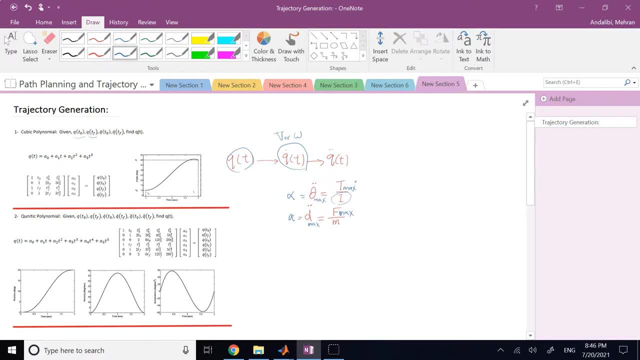 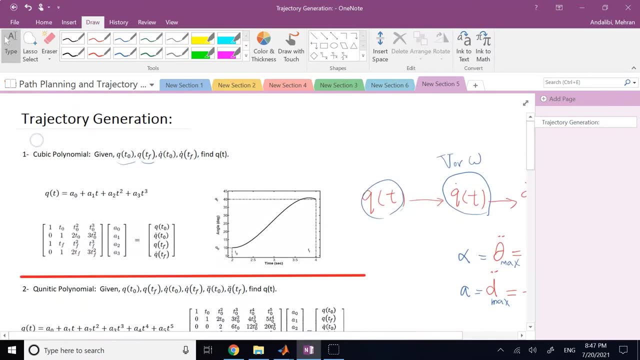 This torque is going to be, let's say, 100 newton meters. Does your motor have that torque? Maybe, maybe not. So you have to know how these joint variables are changing versus time. Good, So now that we know the importance of it, how do we determine that? 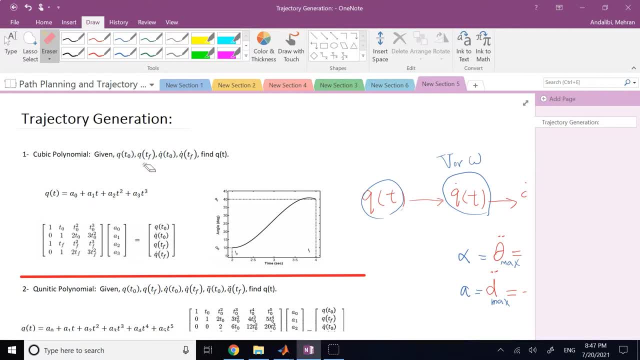 So there are different ways depending on what. What is it that you want to control and what is it that you have, What pieces of information you have? Then there are different methods. What are the limitations, and so on. There are different methods for generating trajectories. 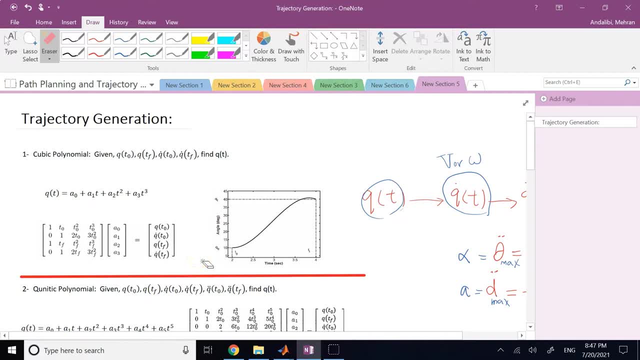 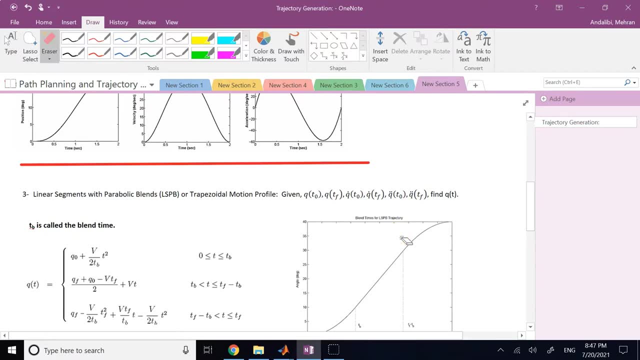 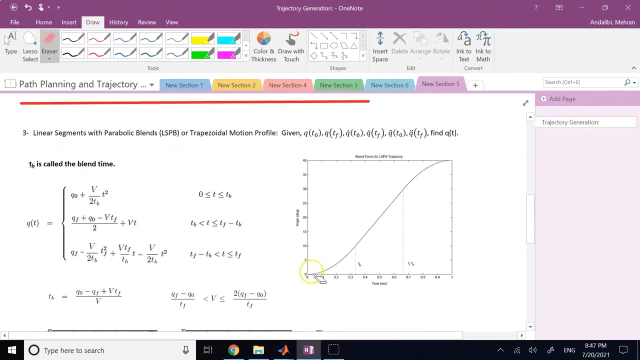 Here we discussed two of them that are polynomial, cubic and quintic. And then there is one that is very common in a robotics application: trapezoidal motion profile, Or you might also call it trapezoidal motion profile, Or you might also call it linear segment with parabolic blend. okay, 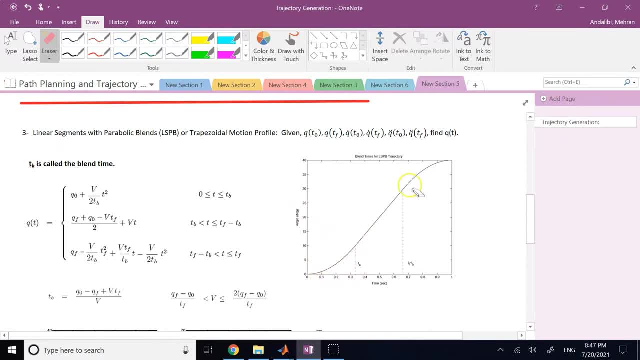 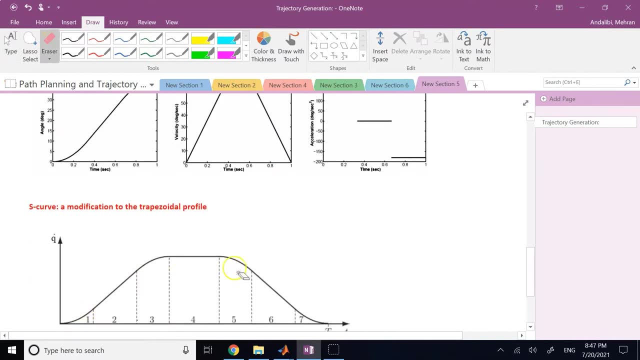 So, in terms of joint angle, it's parabola, line, Parabola in terms of velocity, it's a trapezoidal, okay. And then, finally, we look at the S-curve, which is a trapezoidal, but it is smooth. 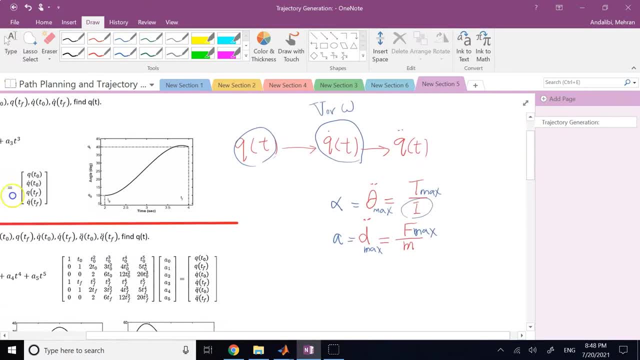 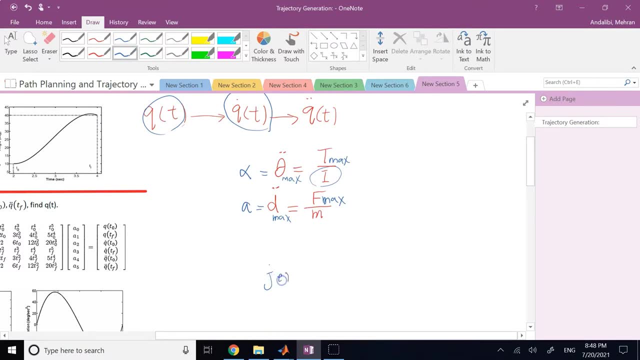 So here we need to look at a bunch of things. The last thing I want to talk about before we start is the notion of jerk. okay, This jerk Is a physical quantity and it is defined as time derivative of the acceleration. okay, 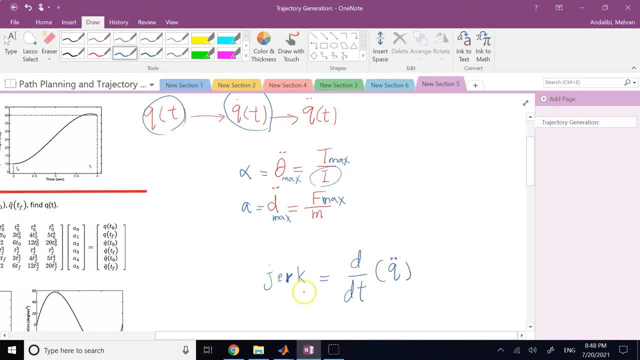 So, for example, if it's theta double dot, jerk is like the time derivative of theta double dot. If it's A, it's like the derivative of A. So the rate of change of acceleration, the rate of change of acceleration, whether it's linear or angular, doesn't matter. 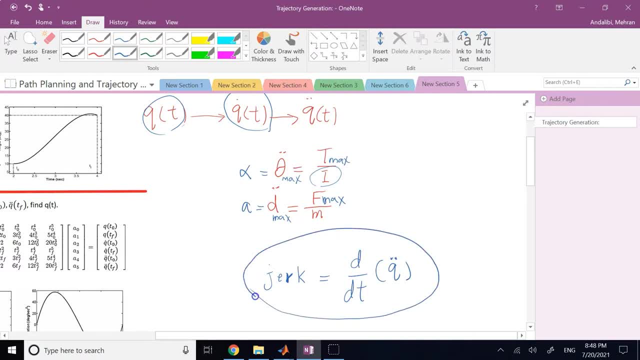 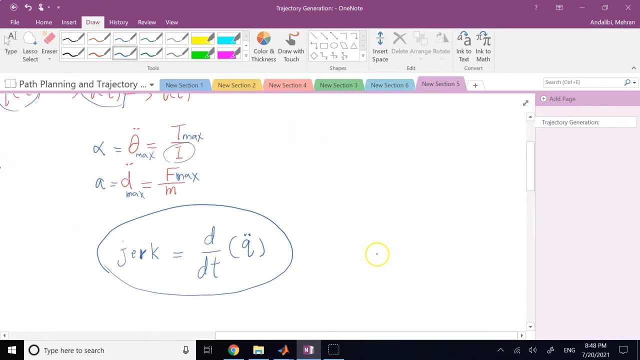 The rate of change. of that. we call it jerk. And what does this one show really physically? As the name says, it's the jerk in the motion. So if you ride, for example, in a taxi, and the taxi, what does have sudden stops, slams on the brake. 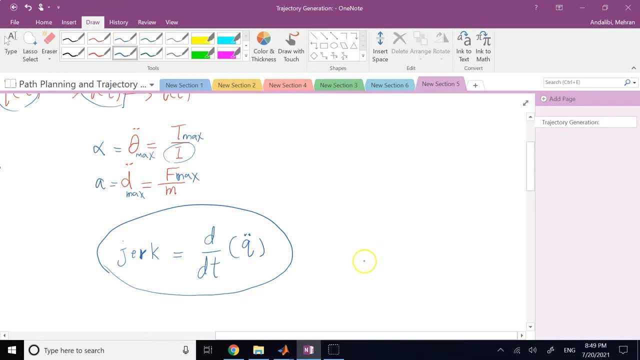 and then when he starts moving he slams on the accelerator right. So if you look at the acceleration lot versus time right, Let's say first the taxi is cruising, so acceleration is zero, Then he boom, slams on the brake and in a very short time he goes to a very big negative acceleration right. 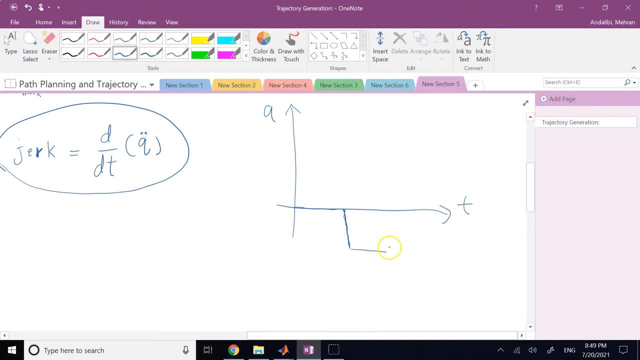 And then what? He goes to zero speed and then stays there stationary for some time. Then, when he wants to stop Start moving again, boom, slams on the accelerator and goes to a huge acceleration again. right, So if you look at this type of motion when you are sitting in the car, you feel all of these changes in acceleration. 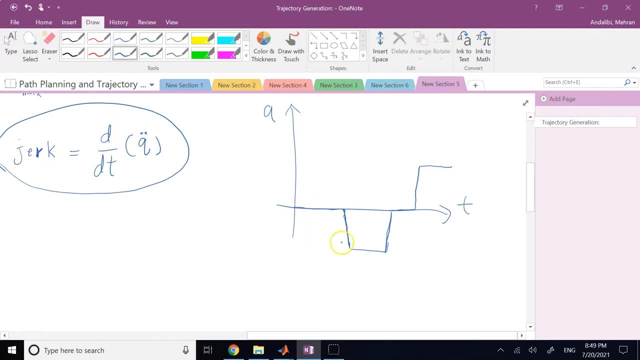 which is basically the changes in the forces applied to your body. And if the forces that are applied to your body from the seats of the taxi, you're not going to feel any comfortable, right? You see, one time the seat is pushing you. 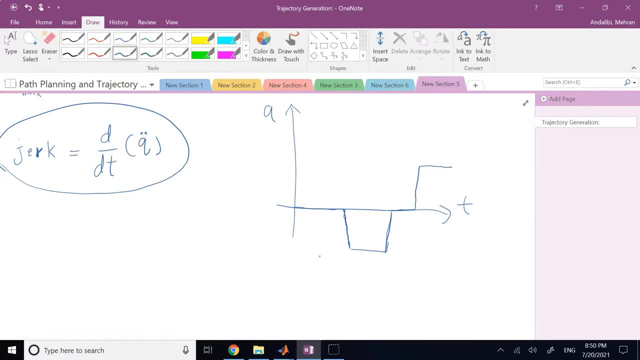 The other time you are going to the windshield and so on and so forth. right, So that's what you felt. Or like when you go to these different rides in a theme park, you see when the merry-go-round or anything like that is rotating this way. 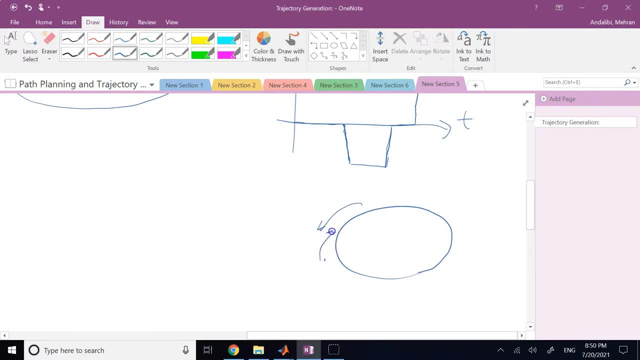 and all of a sudden they what, They stop and they switch the direction of rotation. Or it goes right, Some of these rides, if you have seen when they are also rotating, they also go what Up and Down and those changes in acceleration or the changes in the force will cause the jerk in the motion. okay, 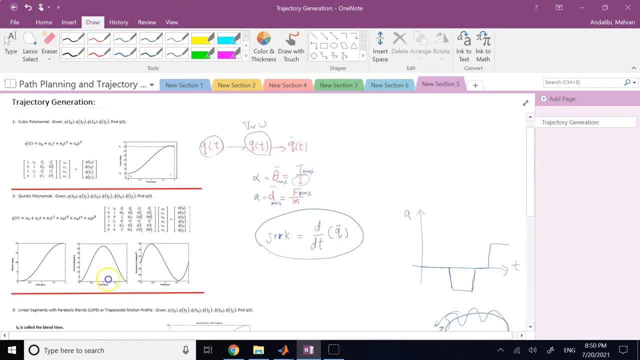 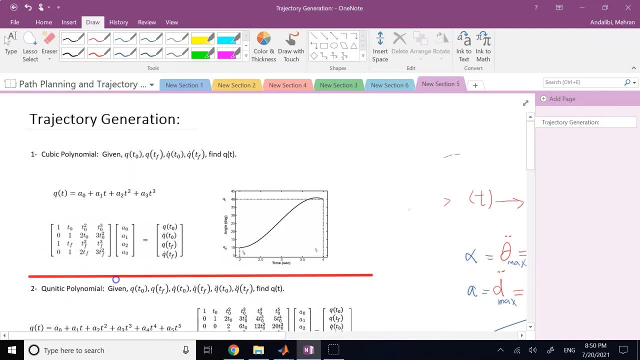 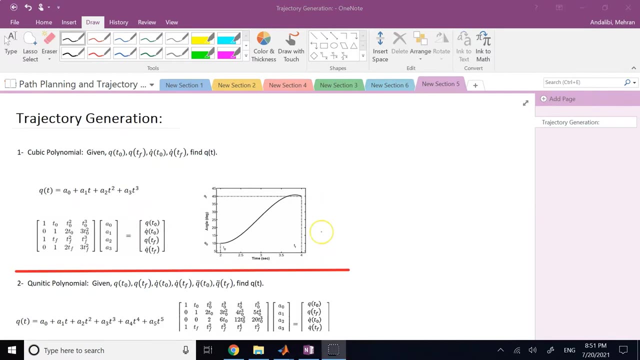 So this idea of jerk, just wanted you to know about it because that is important to us. So now let's talk about the polynomial functions for the trajectory right: Cubic and quintic. So when is it that cubic polynomial is a good function to choose? 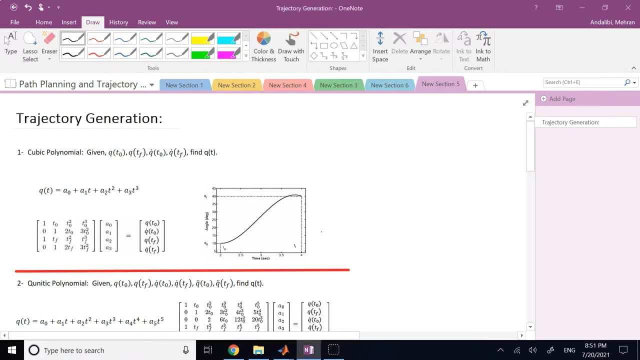 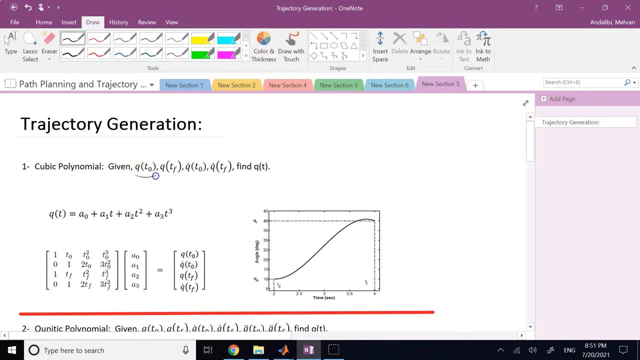 When you only have four values that you necessarily want to achieve. What are they? It's the joint variable at the beginning time, It's the joint variable at the final time, and then the joint velocity at the beginning and the final time, right. 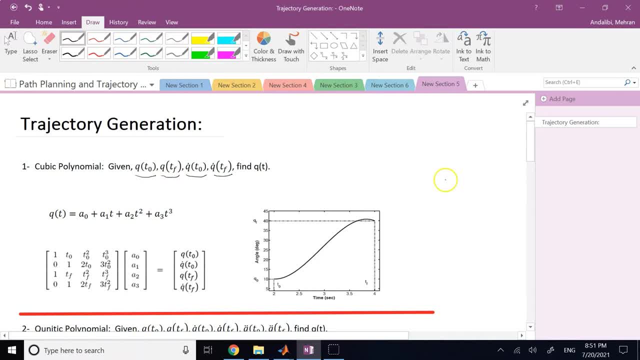 So all you know are the joint values at the beginning, at the end, and the joint velocities at the beginning and at the end, And here we are just focusing on one variable. So here, q It's not a vector, It's just one variable. 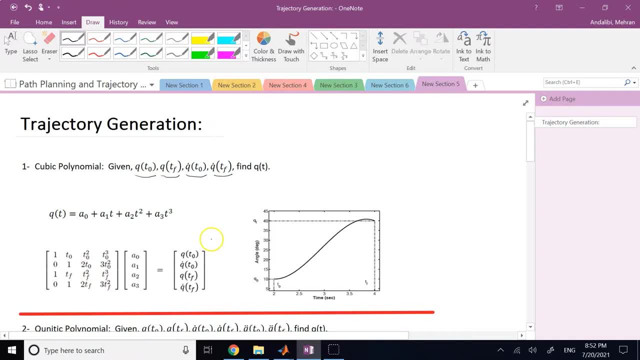 But you can do this operation. You can do this basically curve fitting right to each and every one of the joint variables, right. So if you have four joints and you call them q1,, q2,, 3, and 4,, for each one of those q's you can apply a cubic polynomial like this: 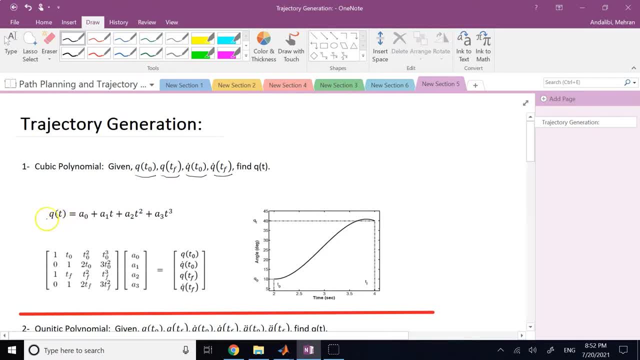 So I say now, this specific q is going to be a cubic polynomial, So it has four coefficients, It has four conditions unknown: a0,, a1, a2, and a3.. And this guy is going to satisfy these four conditions for me. 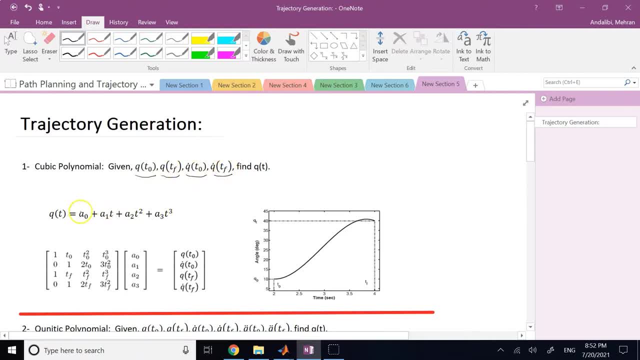 Why? Because it has four unknowns, correct. So we set it equal to this. and then we apply these conditions. So for t, we apply t0 and set it equal to q at t0.. Then for t, again we apply tf and it is going to be q at tf. 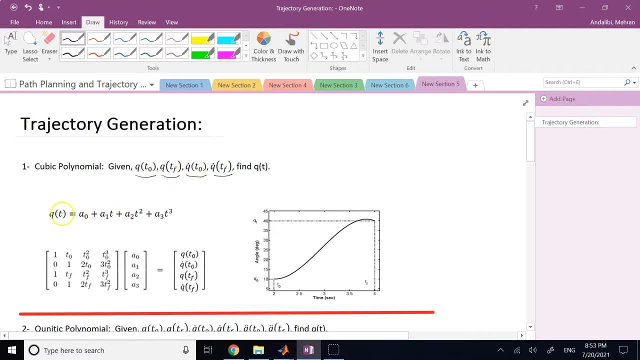 Then we take a time derivative from this And in that time derivative q dot, which is what Clearly you know. q dot is going to be a1 plus 2a2, t plus 3a3 t. squared In that one again you plug in t0 and t final and the values for them. you call them q dot at t0 and q dot at tf. 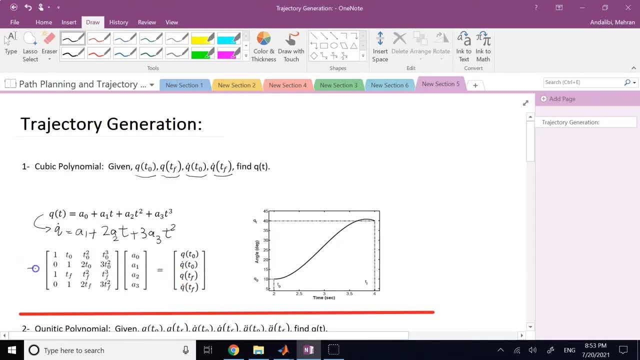 And you will get four equations. Here are these four equations, arranged in a matrix format, where here is matrix on the left-hand side. This a matrix is a matrix with known values. Everything depends on time. This is your unknown vector x, which are the unknown coefficients. 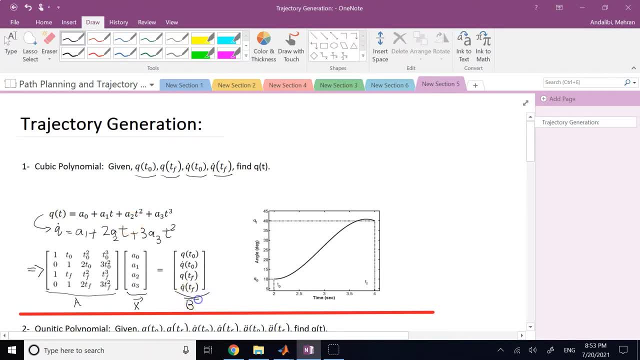 And the right-hand side is also a known vector based on the four given values. So clearly, from here your unknown vector x. This is going to be what A inverse times b, And once you have that, you plug them back here. 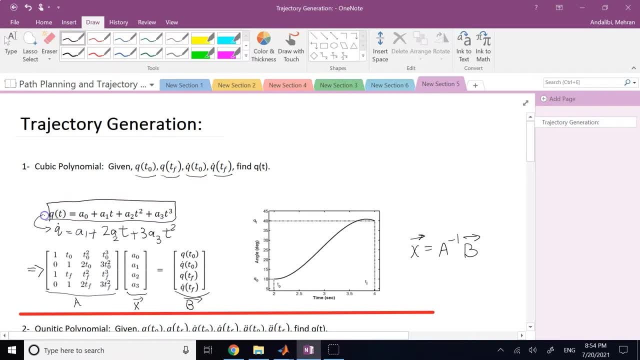 You have now your q as a function of time, So you made your q values parametric. What is the parameter? It is time, Okay, And if you look at the way that the function is so at time t0,, it is q0.. 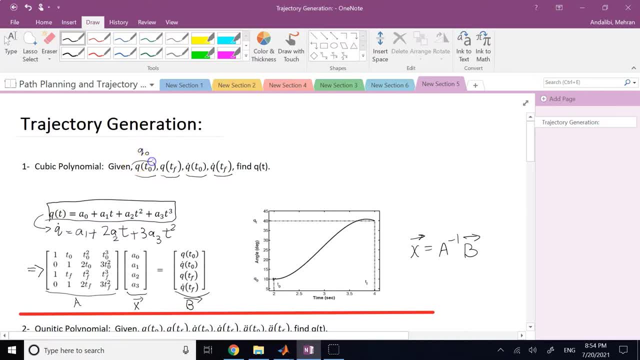 q0 is this guy, This is called q0.. And t final, It is q final. And also the slopes at the beginning, this initial slope here, This initial slope, If you call this angle, for example, alpha, Let's see if I can. 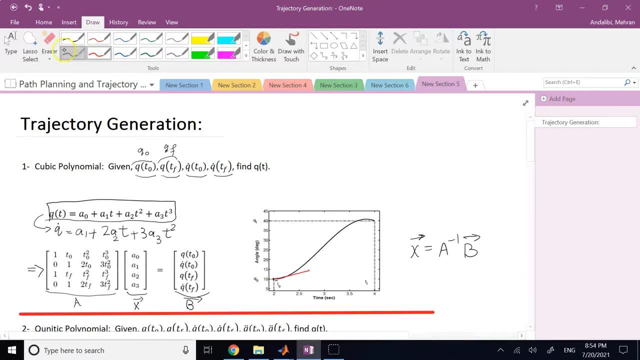 So here this initial slope And this angle is alpha. Clearly alpha is tangent inverse of q, dot at t0.. And then you also have some final slope like this, And again the angle of that with respect to the positive horizontal axis beta. 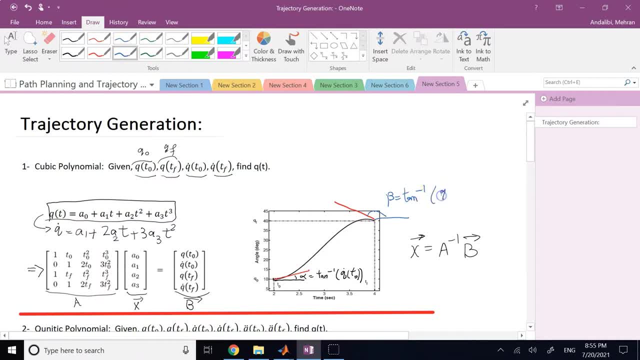 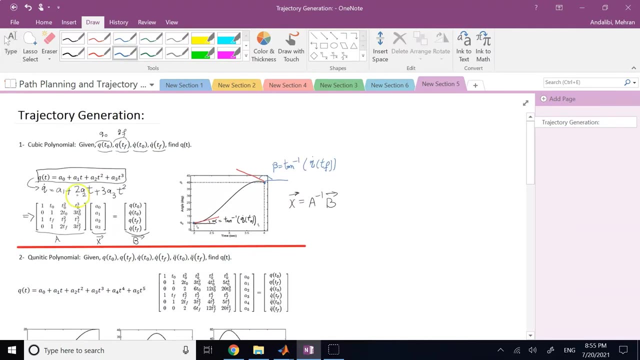 This is equal to tangent inverse of q dot at t final. Okay, So you have the initial and final slope and initial and final value, And it passes a cubic polynomial. This is what you see And then, as I said, you can plot your q dot, which is like this, with the coefficients that you determined. 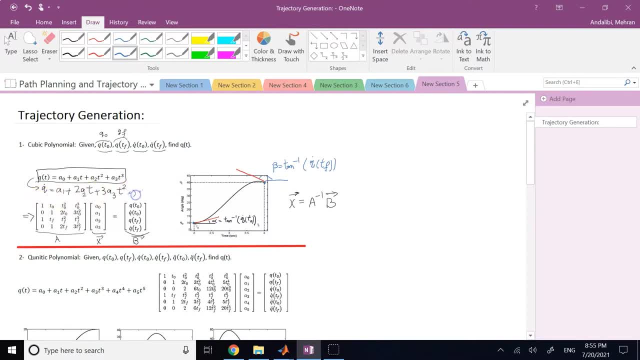 And you can also determine your what Q double dots, E acceleration terms, which is going to be 2a2 plus 6a3 times t. Okay, And so here I'm going to show you that in a MATLAB demo. 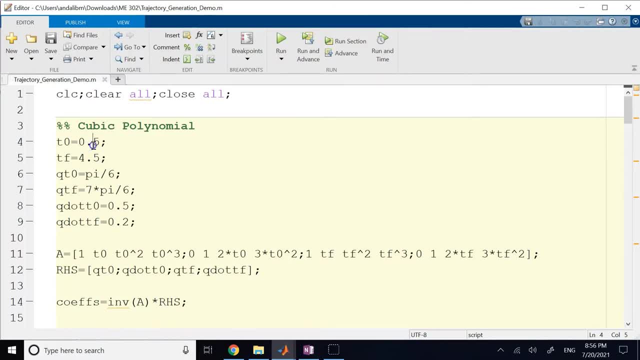 So these values I've chosen is my initial time I chose it to be 0.5.. Final time, 4.5.. I go from pi over 6 to 4 pi over 6.. So all I'm rotating is about 180 degrees. 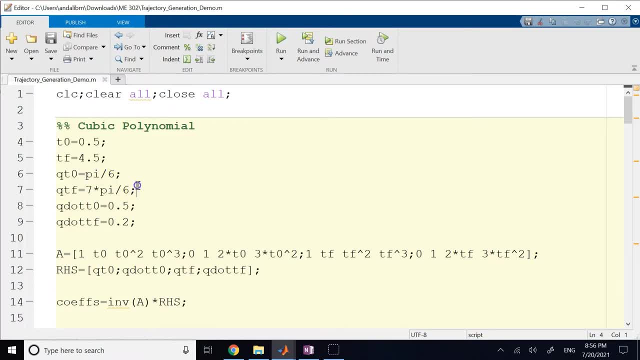 I'm rotating 180 degrees in 4 seconds. It's not such a big deal, And my initial and final slopes are given as 0.5 and 0.2.. I calculate my a and right-hand side here is the same as b matrix. 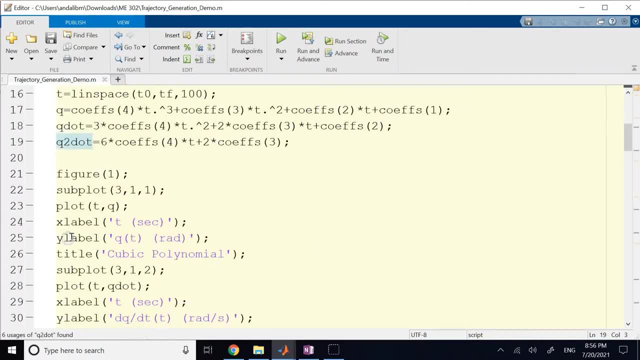 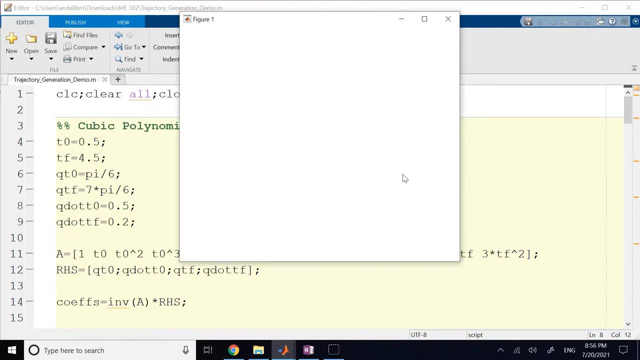 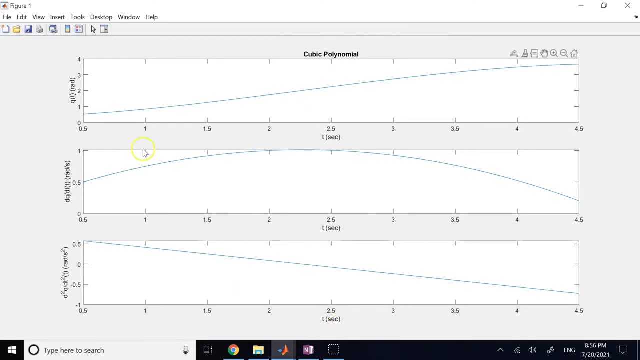 Get my coefficients, Get my q q dot, q double dot, And all I'm doing is plotting it right. So here we go. You can see q q dot and q double dot, all of them as a function of time. 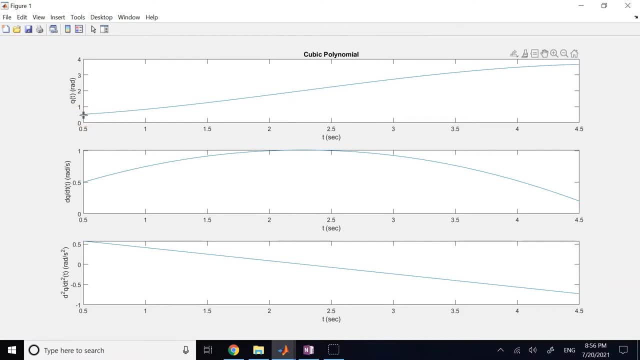 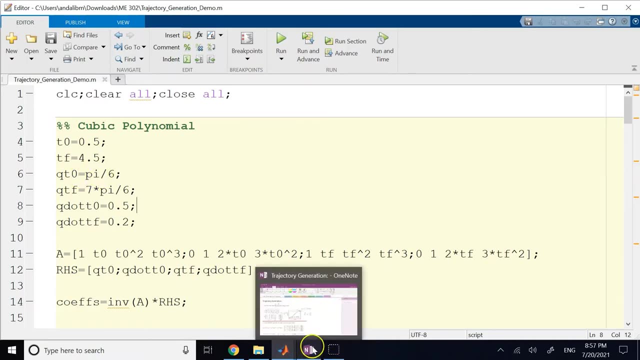 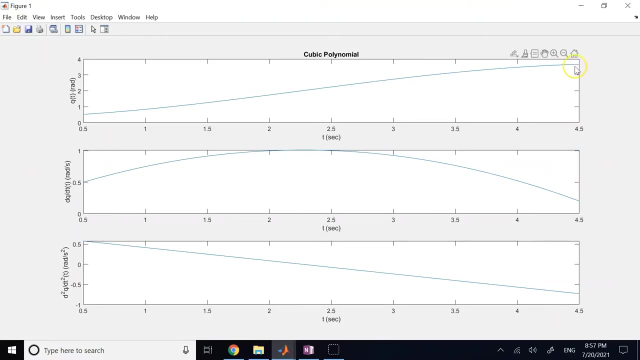 Clearly, you see, your q starts at pi over 6, right, at 30 degrees, And goes to, Goes to 7 pi over 6, right, which is 210.. So you can see, that's 210 radians, of course. 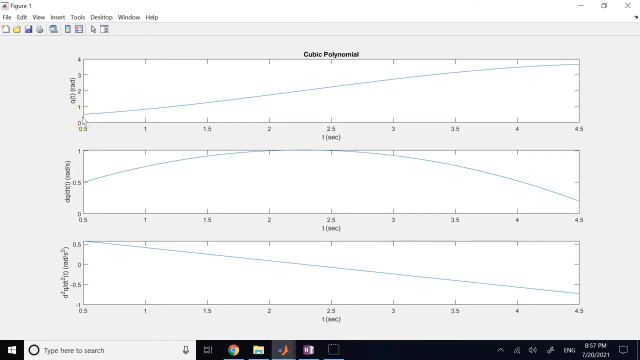 This is 30 degrees of pi over 6.. You know pi is a little bit more bigger than 3, so over 6 means more than half And clearly you see, this number here is a little bit more than half And you have some initial slope of 0.5, and you have some final slope of 0.2. 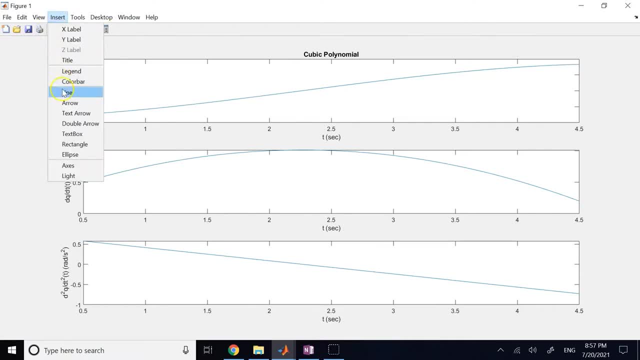 There is a positive slope Both in the beginning And at the end, correct, You can easily draw a tangent line like this And one like that And look at in the beginning and at the end there are some slopes- Not a big slope, but there is definitely one involved. 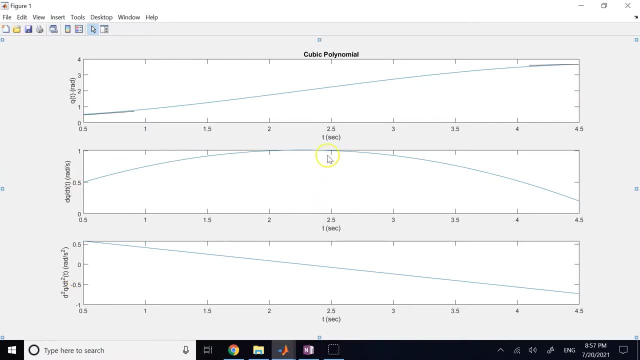 And now if you look at q dot and q double dot, you see your maximum q dot is what One radians per second And your maximum q double dot in magnitude It is here, which is somewhere like 0.72, 0.73 or so. 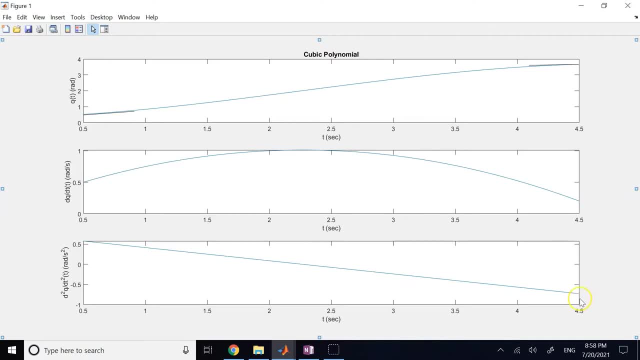 Okay, so now can you have this much of angular acceleration or linear acceleration? Well, it depends on your motor, right, Whether your motor can do that or not. Now to show you the effect of what can change to the maximum: q dot and q double dot. 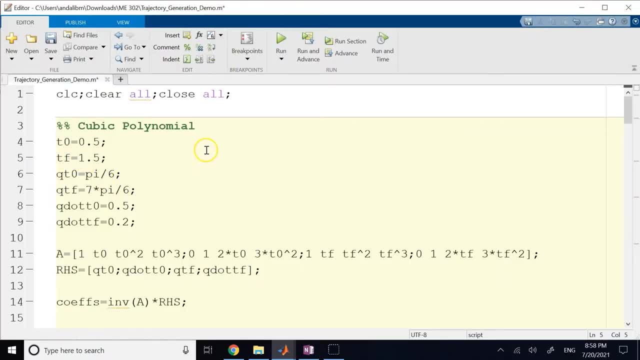 I'll try to make it a little bit faster. I say: in only one second, try to go 180 degrees, Or maybe you know what. Let's make it 360 degrees, So go. one full rotation is in about one second. 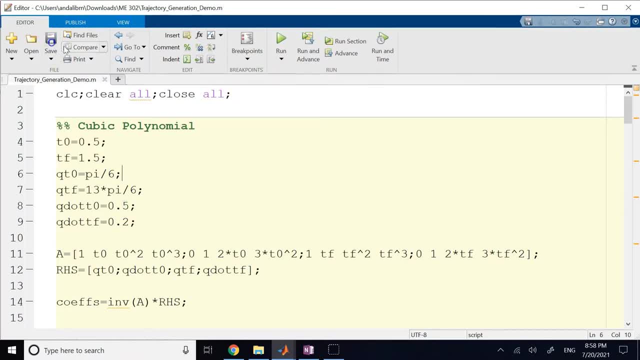 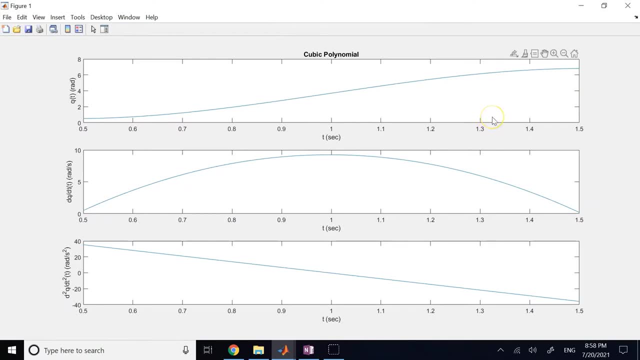 And the initial slope, final slope, are good. So let me run it one more time Now. look So all I did: instead of four seconds, I made it one second And I made the amount of rotation two times larger. Now you clearly see again: you are going from pi over six. 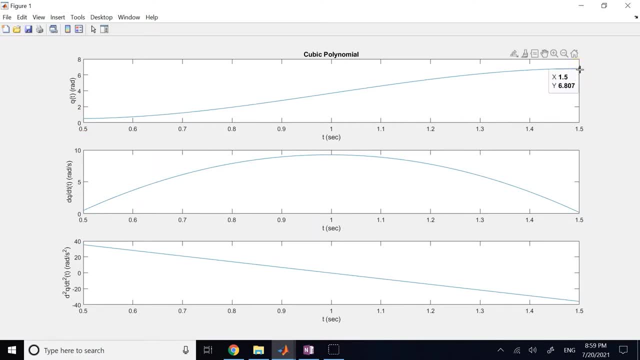 To three to 13 pi over six, which is 390 degrees. But now look at your max value of theta dot, the max angular velocity. Now it is 9.25 radians per second. If you multiply it by 10, it is about 92, 93 RPMs. 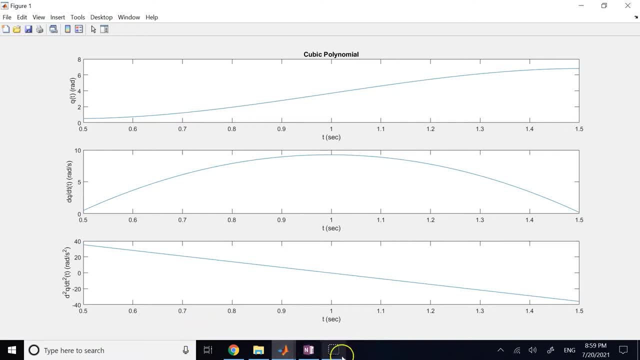 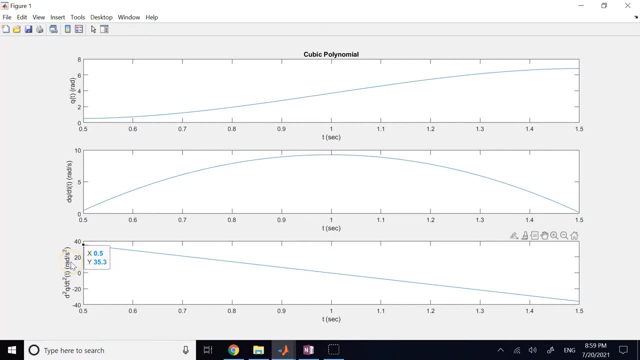 It is 35.3 radians per second squared. If you multiply that by the inertia equivalent of the motor can the motor torque will provide such amount of angular acceleration Maybe, Okay, So we can look at one simple motor here with some specs. 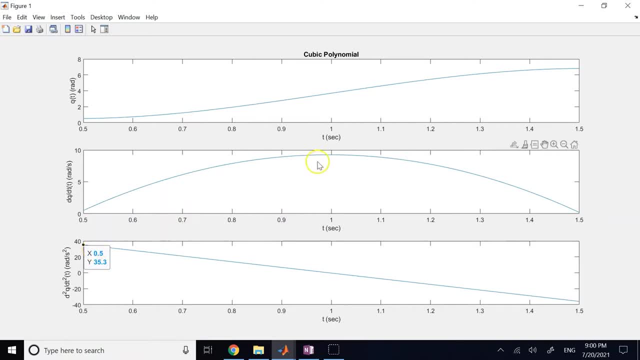 Right, Let's see what is the T max And what is I for it, and what is theta dot correct. And, as I said, this omega and this guy times I, which is torque, these two are not just independent from each other. 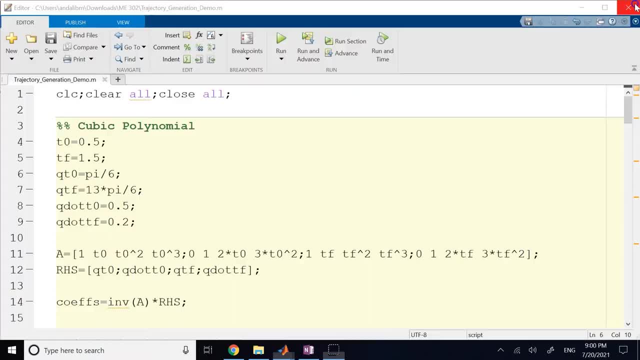 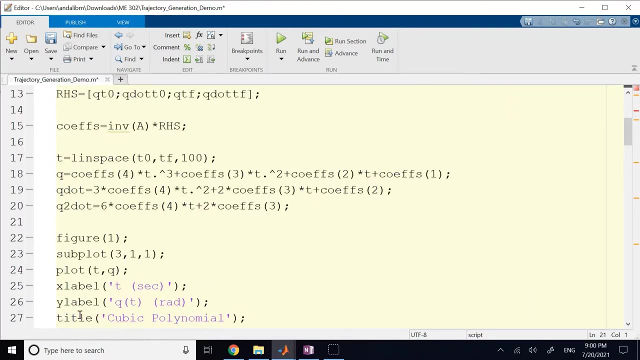 If you want, you can have a fourth plot really and you can consider some I equivalent right. So we come up with a number. Then we multiply our Q2 dot by some I and call it torque. So torque is I equivalent times Q2 dot. 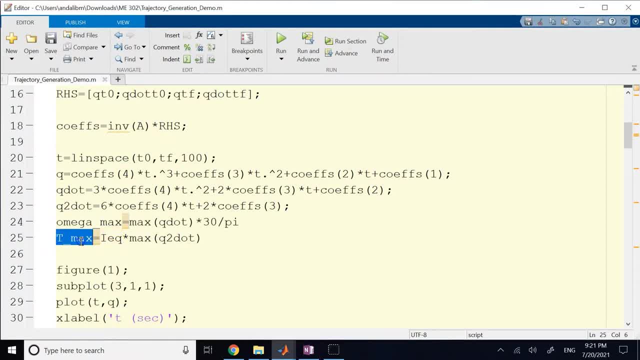 Now here, since I'm interested in the maximum torque that the motion needs, I'm going to get the maximum angular acceleration and multiply it by the I equivalent and call it maximum torque. Okay, Okay, So what I'm going to do in my plan window, I would also convert my maximum omega into 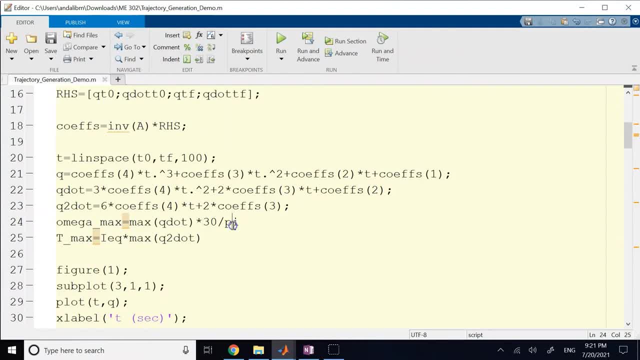 RPM. so multiply it by 60 divided by two pi. and 60 divided by two is 30.. So multiply by 30, divide by pi. So this is max omega in RPM and this is max torque in Newton meters. And if you know from motors, if you have a gearbox after the motor with a T you can have. 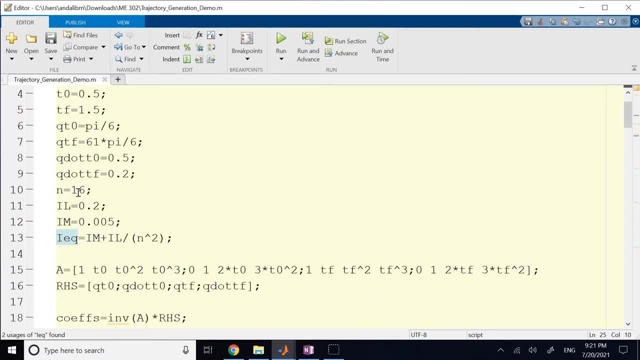 a good torque. Okay, with a speed reduction with factor n, let's say here the factor is 16.. so the gearbox reduces the rpm by 16 times and if you have the eye of the shaft of the motor to be very small number typically, and then i have the load- then the equivalent is going to be the eye of the motor. 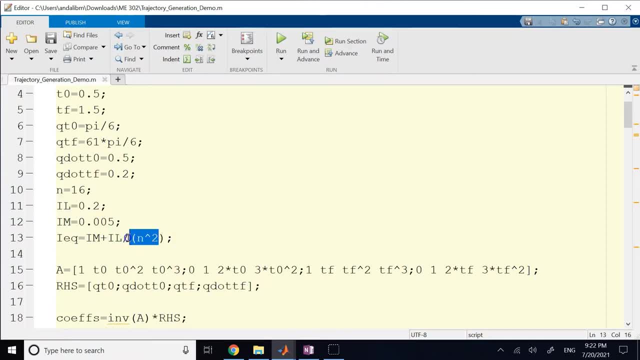 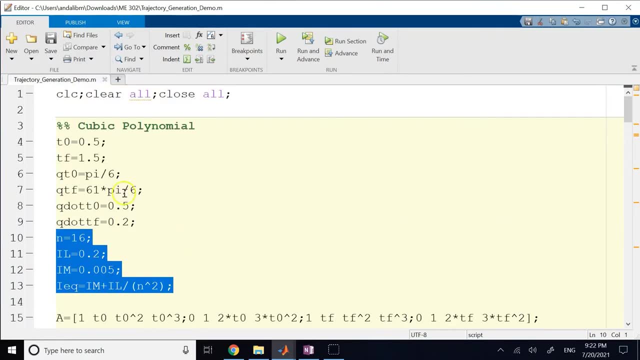 plus the eye of the load divided by the reduction factor squared. so here i calculate that and then i plot this. here i also made my um final angle to be quite bigger. so instead of going one full round now, it is going five full rounds. okay, and five is basically 61 divided by 12, because in 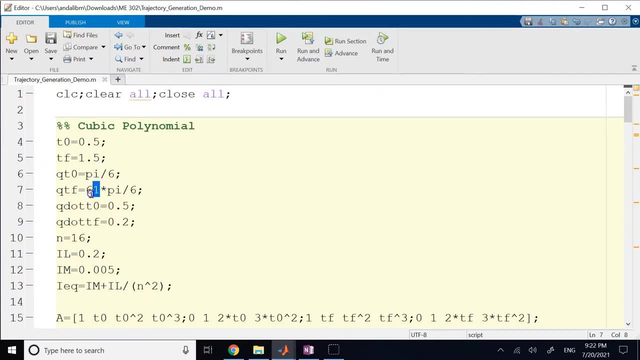 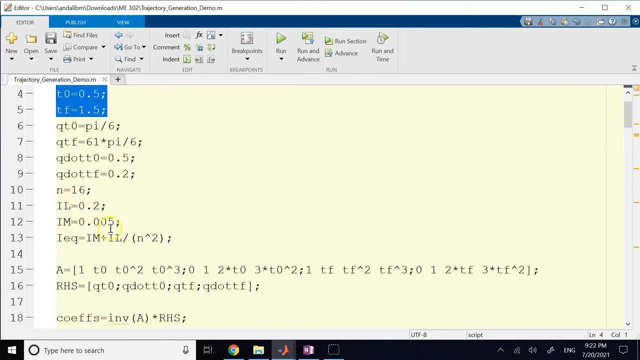 each full round you have 12, 30 degrees and this is 61 times that and the first one is one times that. so the difference is 60 times 30 degrees, which is five times 360.. so it is doing five full revolutions in one second with these numbers. for 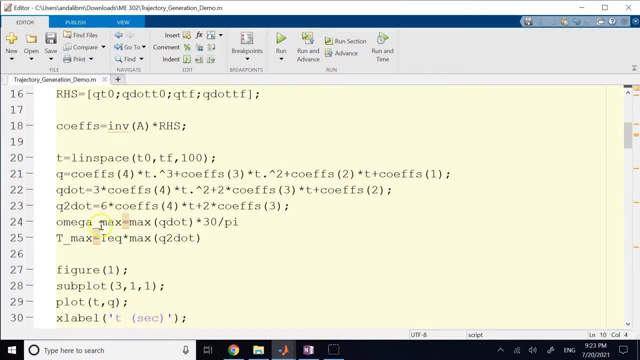 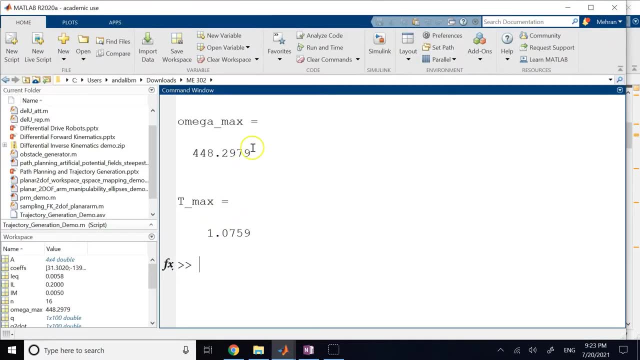 the inertia of the shaft, the load, the gear reduction and everything. and if i run this to get my plots, now, if i go and look at the values for maximum rpm, it is 448 rpm and max torque is 1.07 newton meters. right now, if i go, for example, and search a 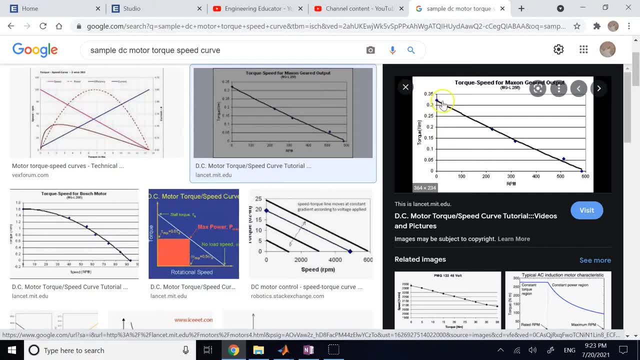 specific dc motor. right then, uh, i get this kind of curve, as i said, the rpm increases, the torque drops, and vice versa. and now, if i look at the maximum torque, which we call the stall torque, for this, uh, let's say dc motor, it is something like 0.32.33 newtons meter, while here you can see 1.07. 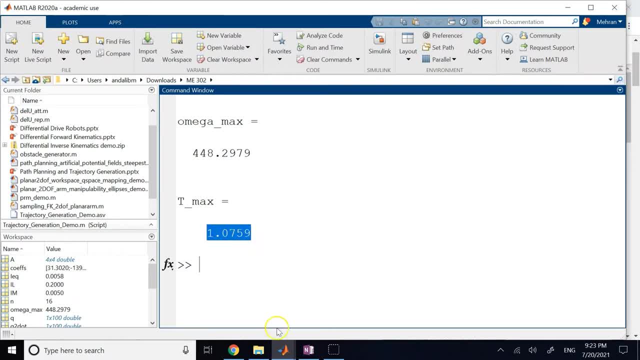 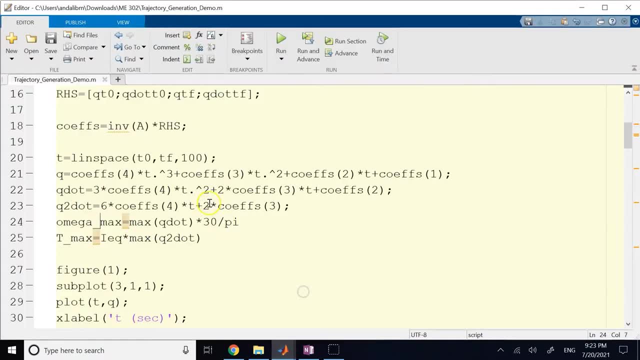 which is like three times bigger or more. so, definitely, if i want to achieve this motion, it's not going to be possible, right? it is not going to be possible. so i have to change this q as a function of time, right? or i have to choose a different uh motor that is more powerful, or bump. 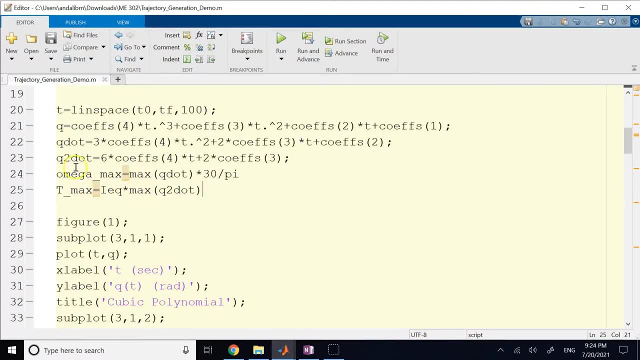 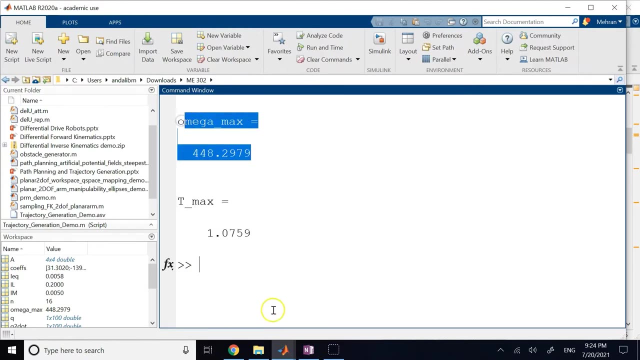 up the voltage of the motor. so clearly you see this function of time, q, as a function of time, determines q. double dots, when multiplied by i equivalent, determines torque max and torque max determines whether you can go with the motor that you have or you have to change it. so the 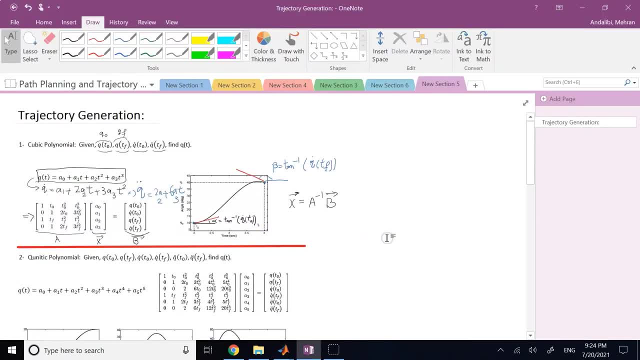 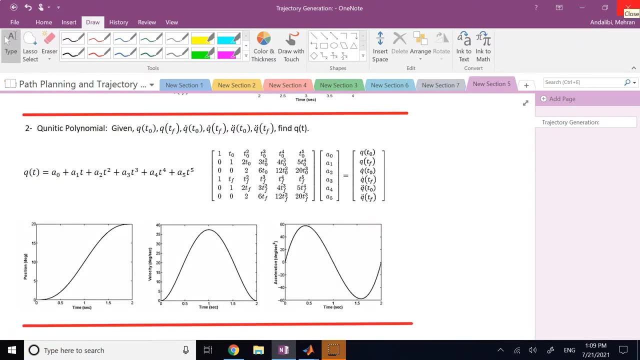 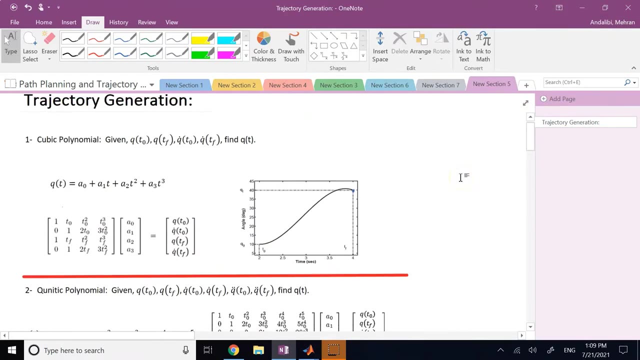 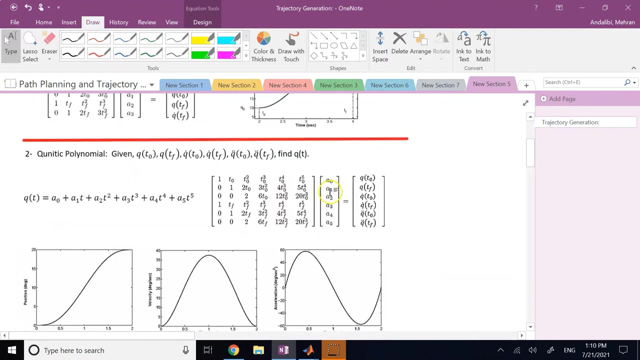 choice of the time function in this trajectory generation is very, very important. okay, now it is time to look at quintic or fifth order polynomials. so last time we saw that we chose cubic with four unknown coefficients because we were given four numbers that our polynomial had to satisfy: the initial and final joint values and the initial and final speed values. 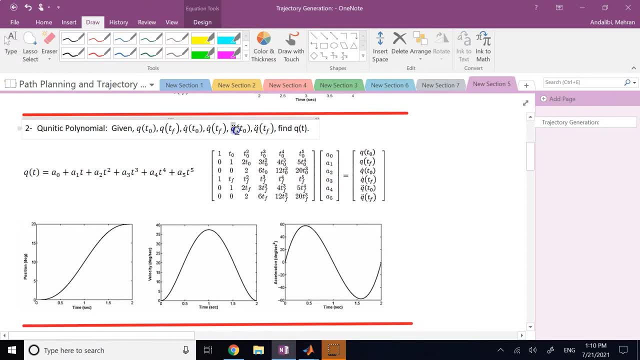 now, if we also have to satisfy the initial and the final acceleration values, q double dots, then we definitely need six coefficients, and that comes from the fifth order, polynomial. like this and again the unknowns from a naught to a5 can easily be found using a matrix format. 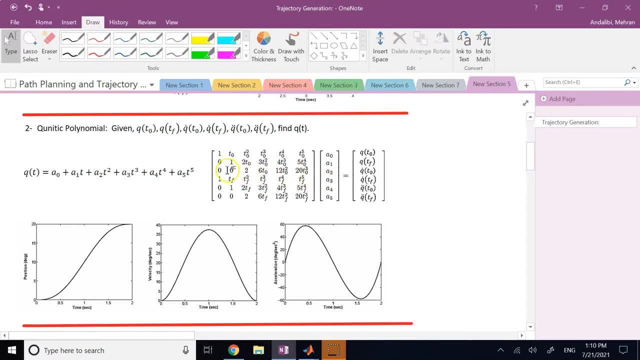 right where here you have a coefficient of known values, the coefficient matrix here, which is all based on the time, t naught and t final. so this is the known matrix. a right hand side is also the given numbers, and so by inverting this matrix multiplying by the right hand side, you can get your. 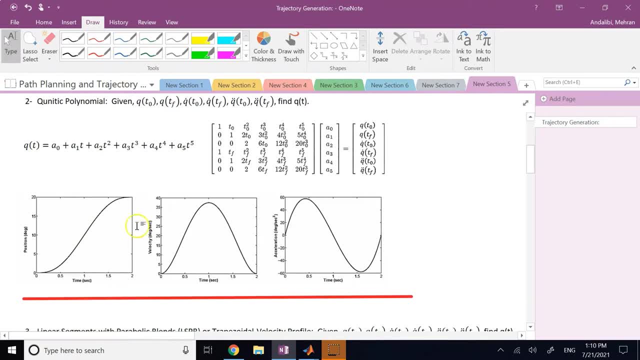 coefficients. and now if you look at, for example, position for a specific set of numbers, you see it is a fifth order. now it might look like a cubic. it might, yes, depending on your um, initial and final q and initial and final time. and then you have the velocity, which has some max velocity, and you have some acceleration, which has some 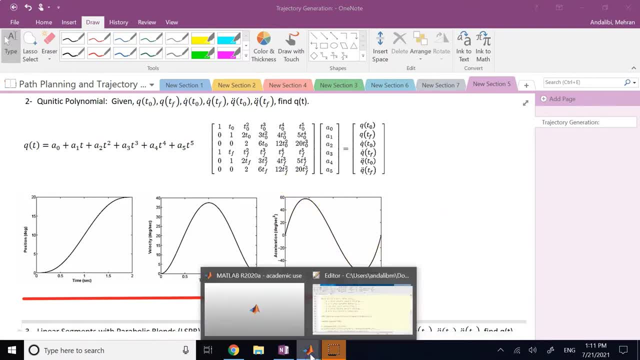 again max and mean values. so here i'll show you a demo of that, and i use the same numbers i used last time for cubic. so i'm going to show you a demo of that and i use the same numbers i used last time for cubic. so 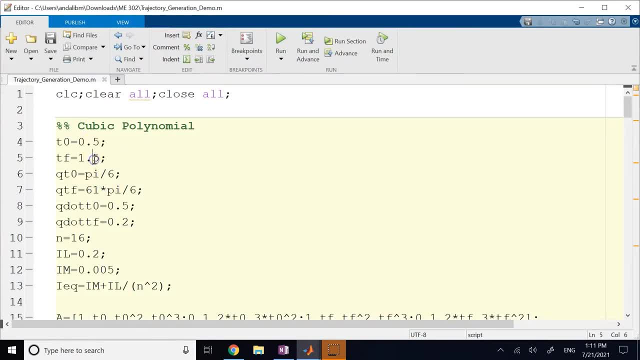 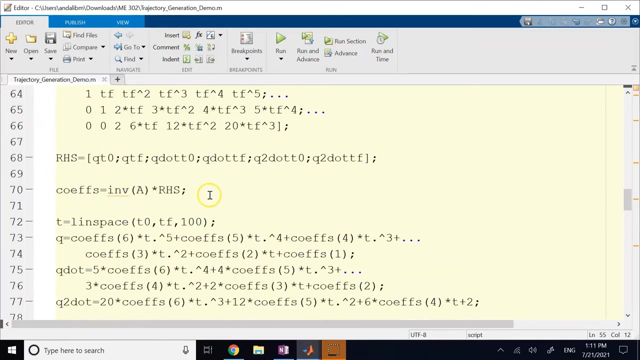 i go for five full rounds in one second. and last time we have to satisfy the two initial and final speeds. this time we also have to satisfy the initial and the final accelerations, zero and point one, and uh, i also again calculate the maximum torque and the maximum speed and uh, show them with f, print f. so uh, if you remember. 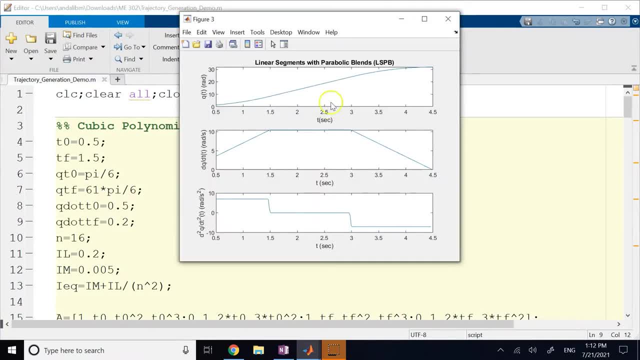 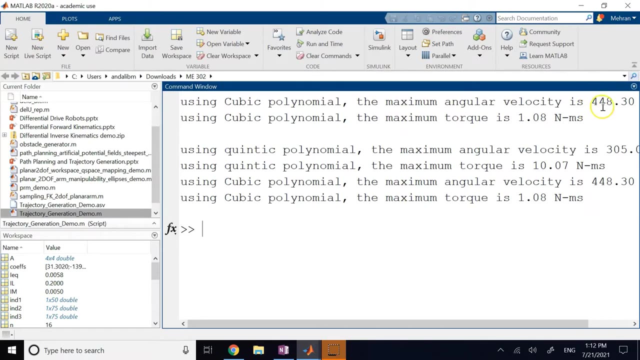 when we did the cubic with these numbers, right? uh, i guess i ran the whole thing when we did cubic. this is the chart that we got and the numbers that we got were also here. i guess, if you can see them right, let me clean up everything and do it one more time. 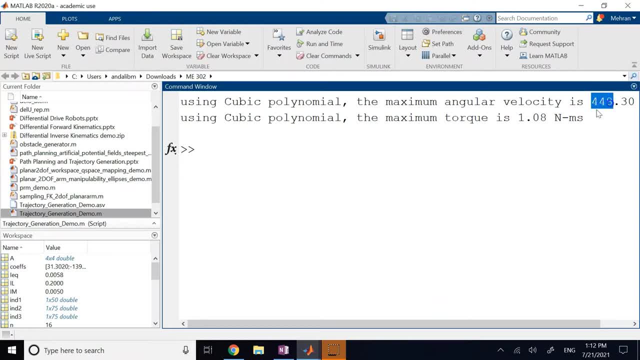 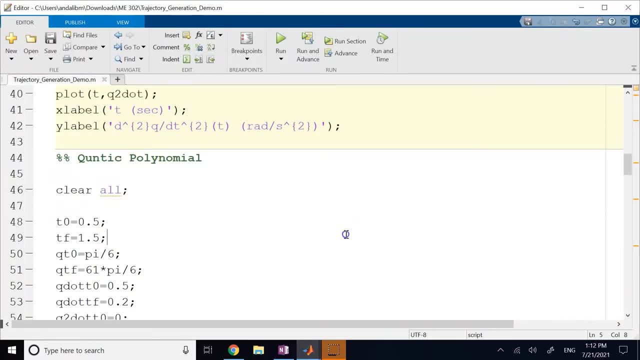 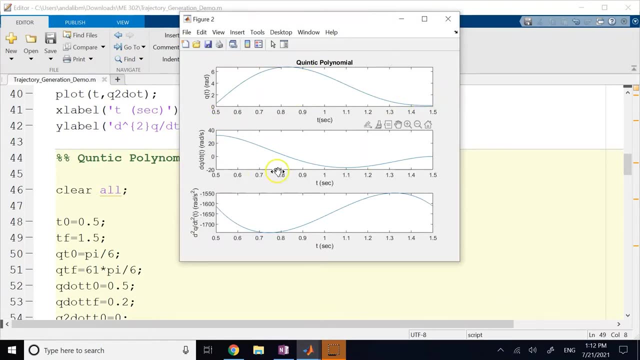 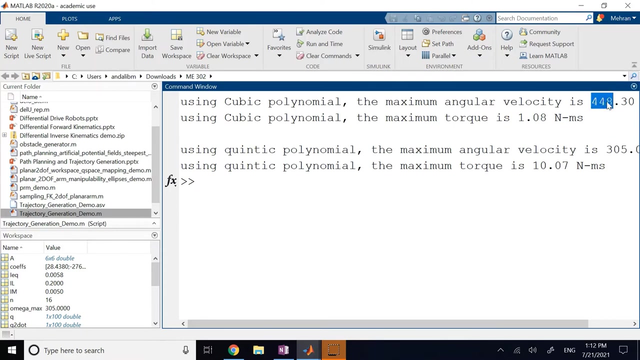 so the max rpm was 448 and the max torque was 1.08 newton meters. now here i'm gonna do the quintic one, and this is how the plot would look like for the setup numbers that i provided. and now, if you look, your maximum rpm is even less than the cubic one, but if you look, your maximum torque is: 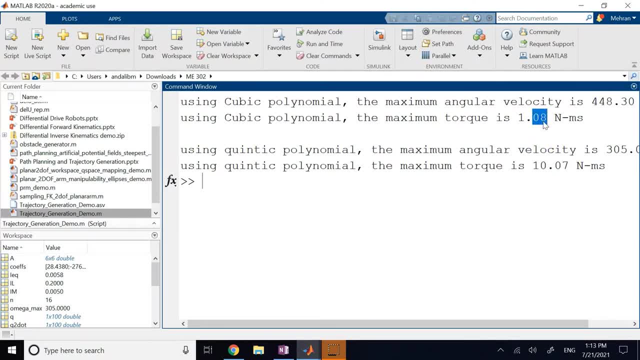 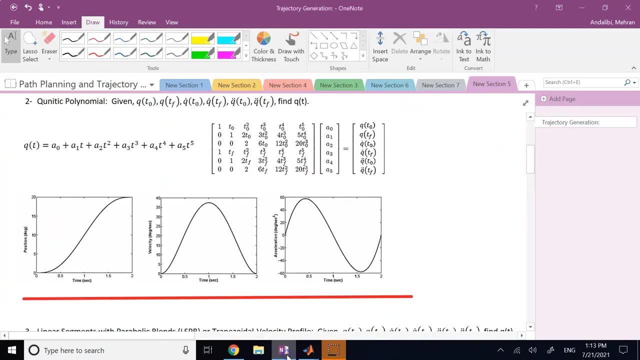 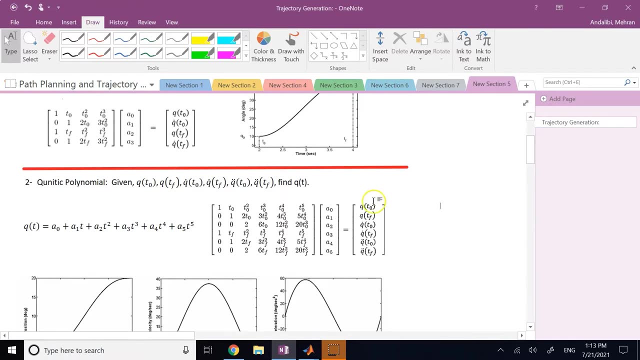 way larger. okay, so that's another thing that you have to consider. that, uh, the order of the polynomial. of course it does depend on how many conditions you have to satisfy, but in general it's not really a good idea to add to the orders of the polynomials when you do curve fitting. 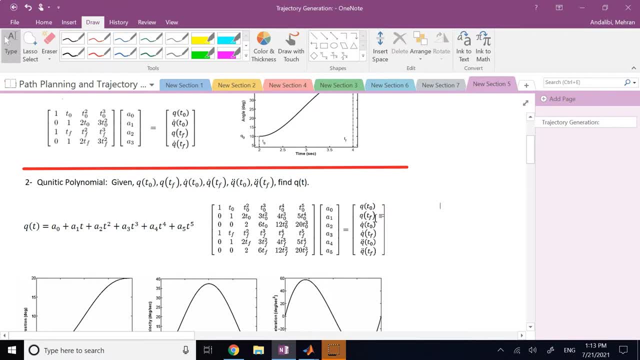 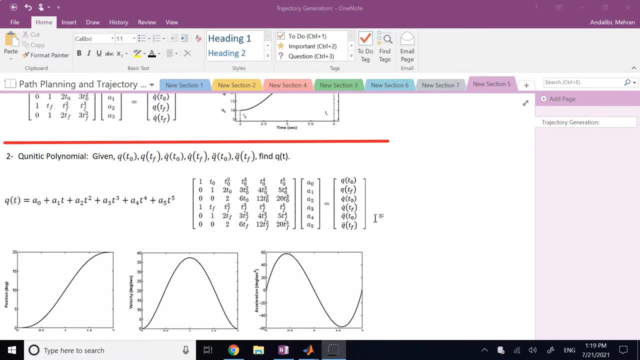 and you know the problem. there is called the uh overfitting problem, which will be discussed in a later video. but i guess if you go to my channel under the playlist engineering mathematics and look at the curve fitting video where i talked about list of squares, curve fitting, you see over there when i talk about polynomials, i explain the problem of. 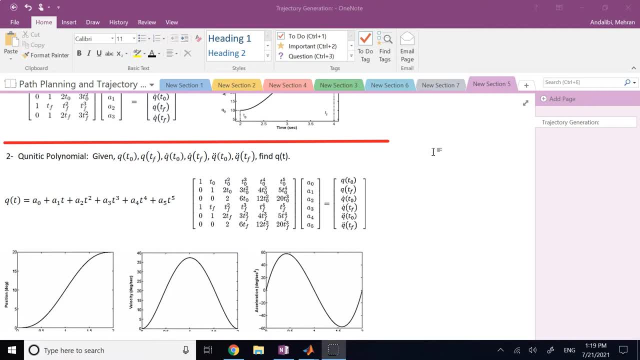 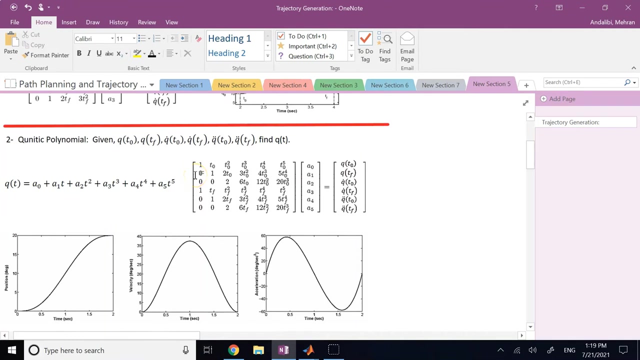 over the issue of overfitting. okay, so, uh, you can refer to that. in general, we try to use as small as parameters that we can, minimal number of coefficients we can to satisfy all the conditions. okay, so these are the two polynomials that we typically use, but there are other types of 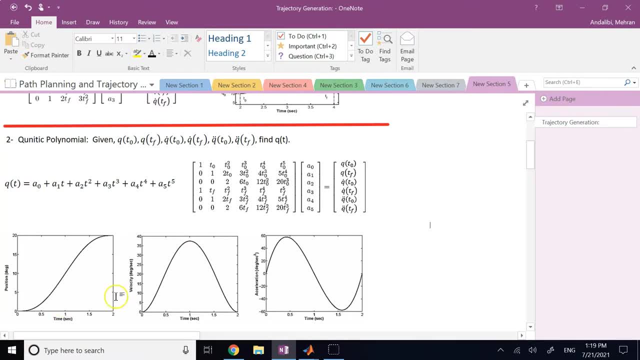 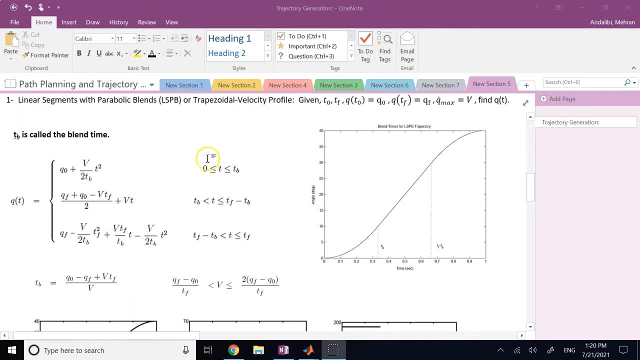 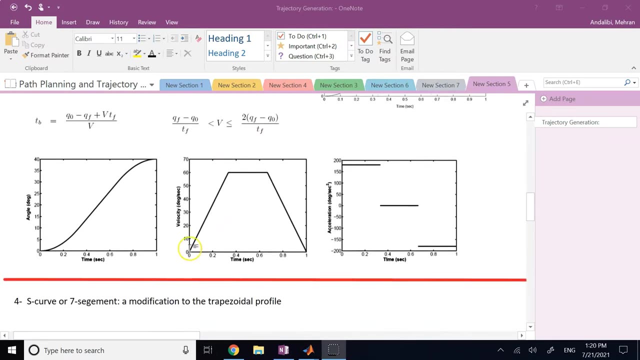 profiles, trajectory profiles that we can use, and one of them is called linear segments with parabolic profiles, and then the other one is called linear segments with parabolic profiles, blends, or lspb, sometimes also called the trapezoidal velocity profile. so what it is is- uh, i'm given the initial time and the final time, the initial joint value and the final joint. 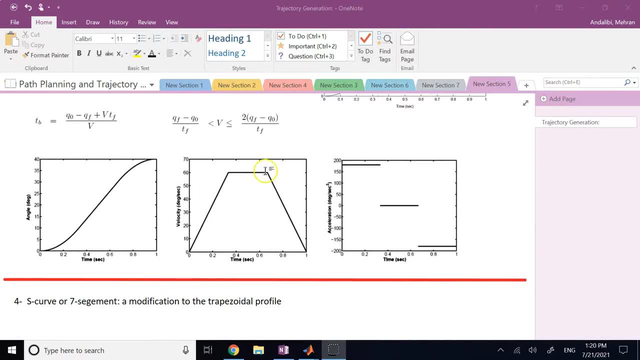 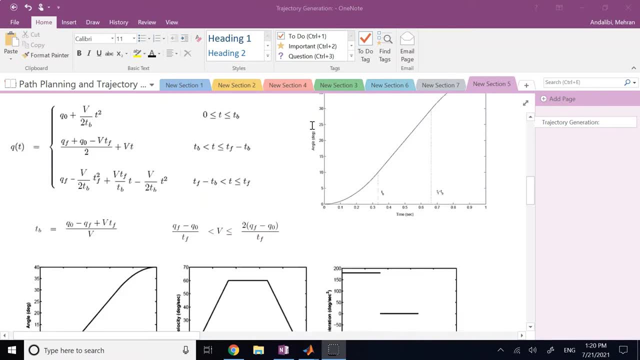 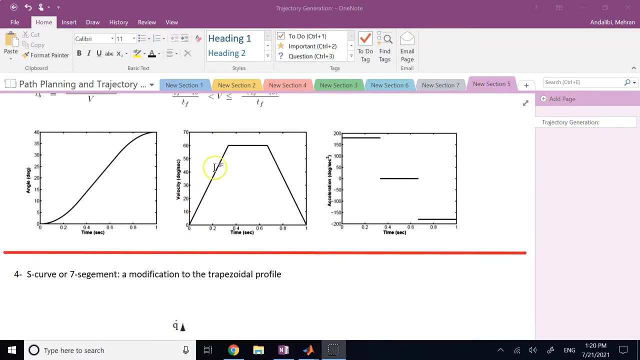 value and the maximum speed that i want to achieve. okay, or i can achieve. so i'm given these five parameters and what i want to do is to go from my initial speed of zero to some max speed, then, uh, go at constant speed and then decelerate and go back to zero speed. okay, 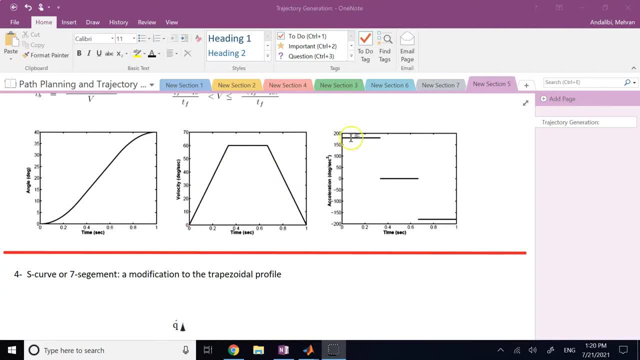 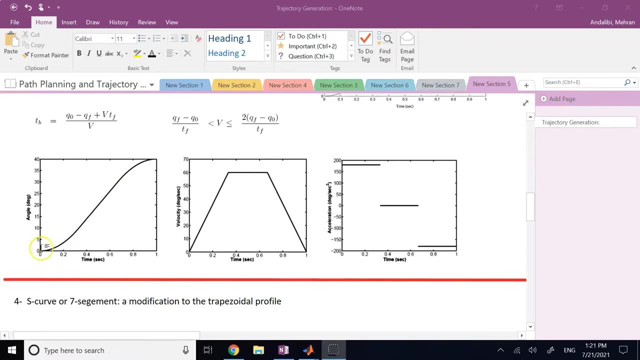 so the velocity profile is going to be a bunch of lines, the acceleration is going to be positive, zero, negative, and, of course, when you integrate the velocity, so the joint angle is going to be a parabola, a line and another parabola. that's why you call it the linear speed. 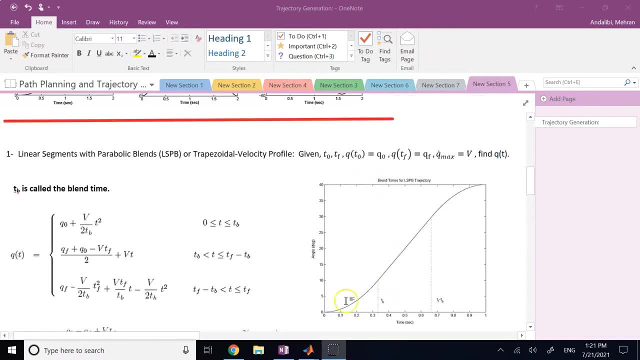 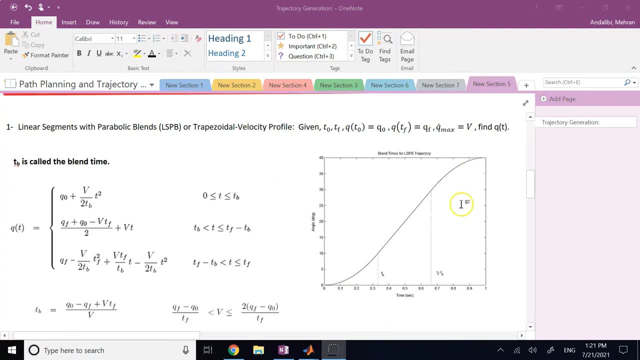 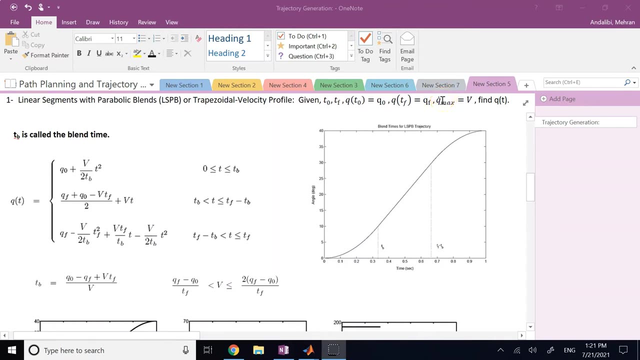 segment, which what you can see here, and with two parabolas that will blend to it and create the whole profile. so, as i said, here i'm given four, five parameters: t- naught, tf, q naught, qf and v, which is q dot max, and i need to find q as a function of time. okay, so clearly, as i said, we 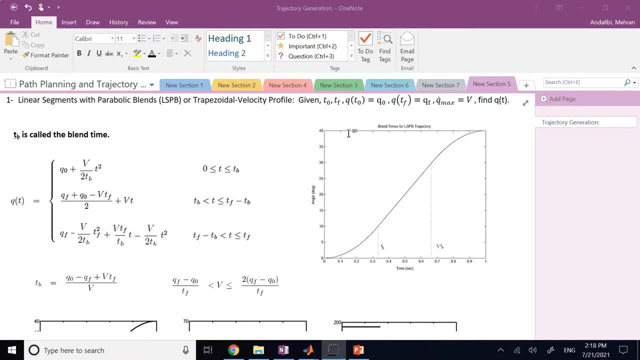 have eight coefficients, three for each one of the parabolas and two for the line, and i have five given parameters. i'm not going to be able to calculate all of the unknown coefficients, so we need some extra conditions, and two of the conditions that we have here is 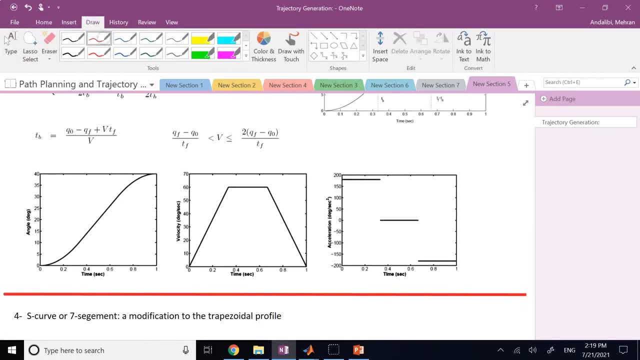 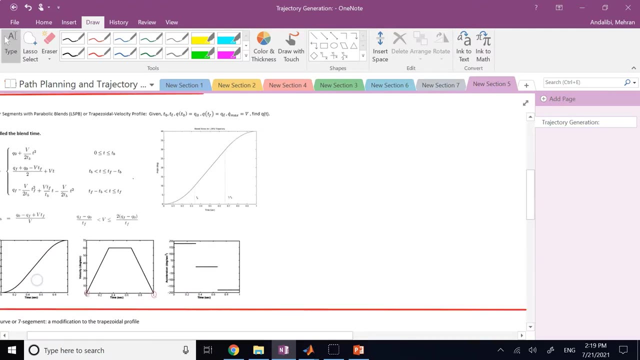 we start from zero initial velocity and we go to zero final velocity. okay, so these are two extra conditions and we have two extra conditions and we have two extra conditions and we have two conditions right which are very important. so if i want to write this problem, the conditions that i have in general are that q at t naught is equal to q naught. 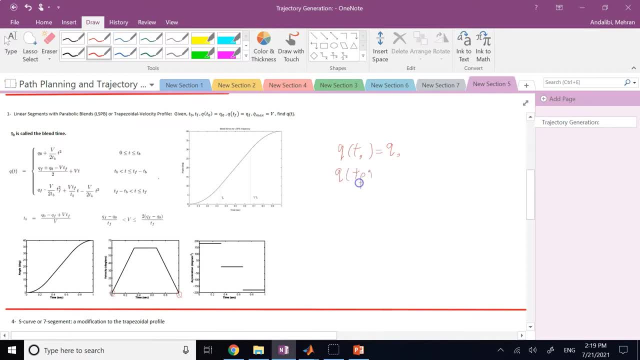 q at t final is equal to qf. these are two equations: q, qf. q dot at t naught is equal to zero. q dot at t final is equal to zero. this is four. then we have continuity conditions, which is basically at this time where you go from. 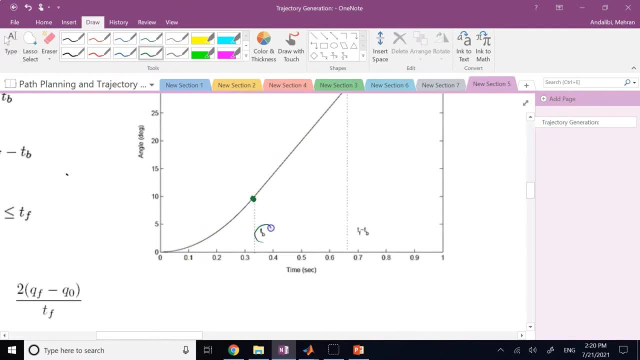 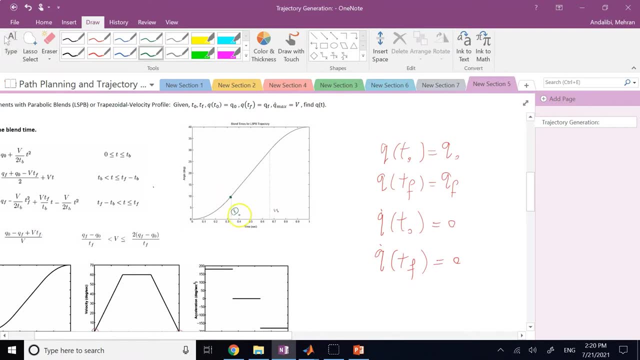 parabola to the line and we call it tb or blend time, which i mentioned for you here. at the blend time, which is an unknown, and we have to determine that at this t blend, what you have is the value of q from the first function should be the same as the second function. so if i call this portion, 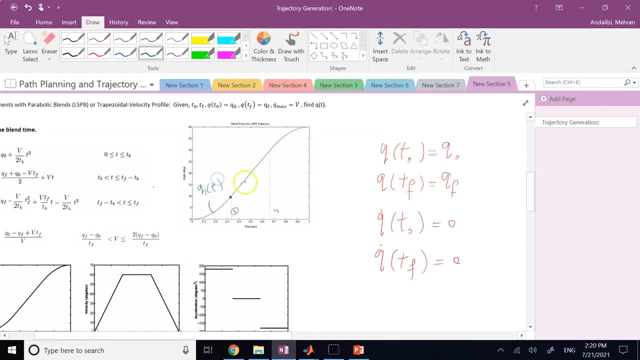 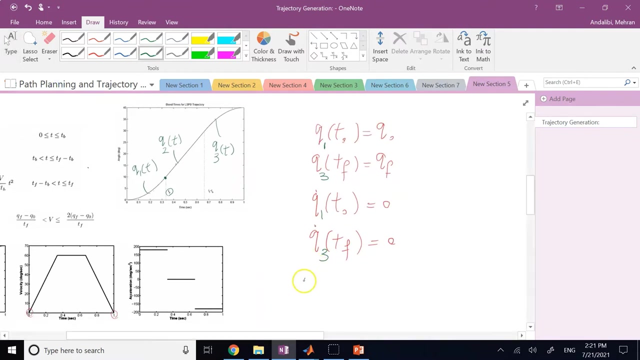 q one of t, i call this portion q two of t and i call this last portion q three of t. right then what you have is: this is q one, this is q3, this is q1, this is q3. okay, and then continuity conditions will give. 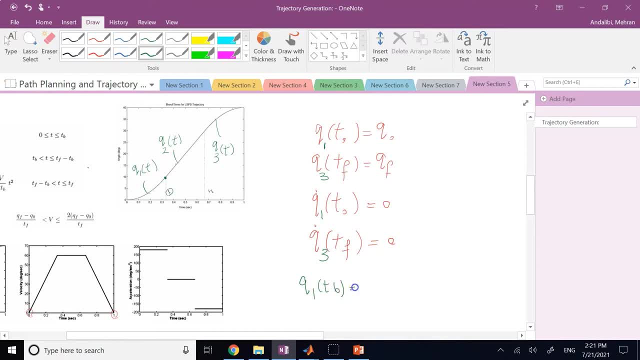 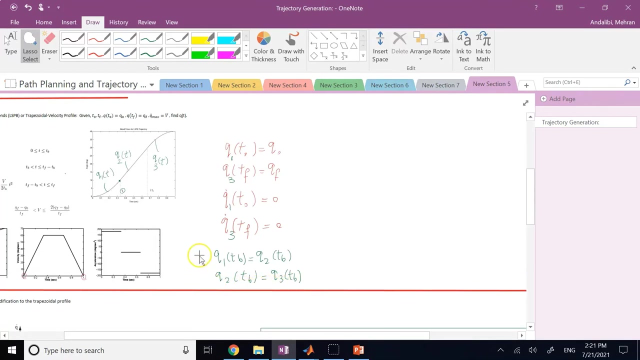 me, q1 at T blend is equal to q2 at T blend. so that's one more condition. and then q2 at T blend is the same as q3 at T blend. so these are the continuity conditions. and also q2 dot at any time should be equal to this V. remember I said the? 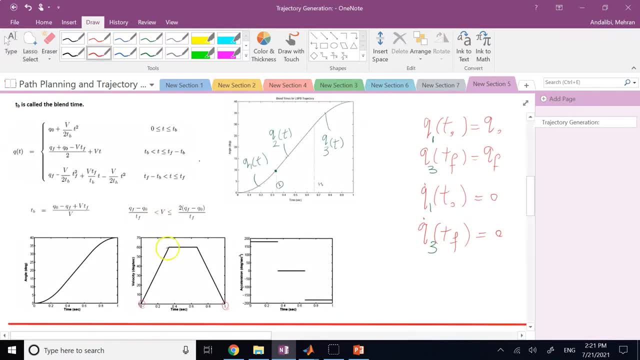 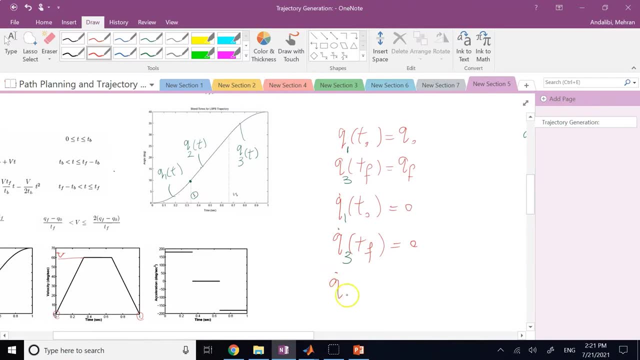 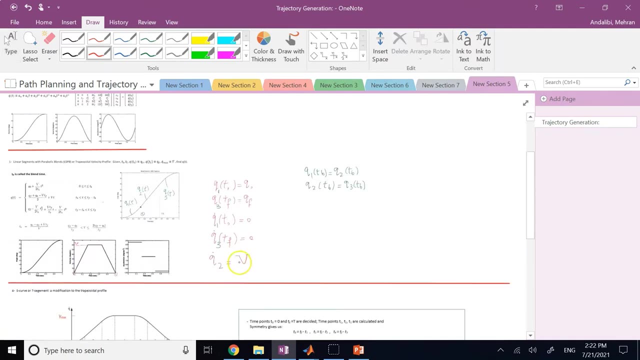 maximum velocity we have is called V and that is this point here. so this point here is V. so I can say dot in general should be equal to what V, correct? so that gives me the slope of the line right, that's V. these two, as I said, are continuity conditions and then 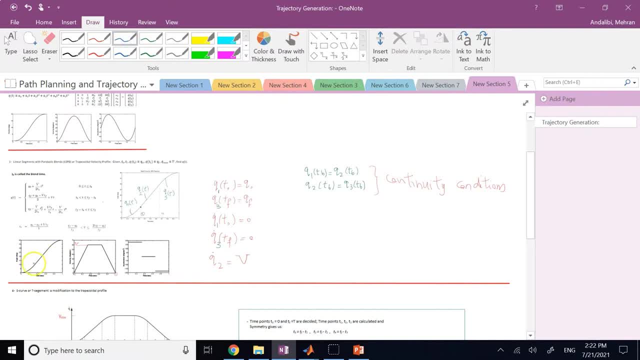 I have smoothness conditions, which is basically the slope of the first function, q1 at the T blend should be the same as the slope of the second function at T blend. so q1 dot at T blend should be the same as q2 dot at T blend and 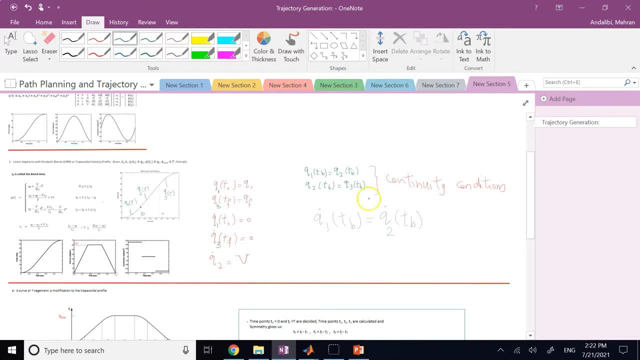 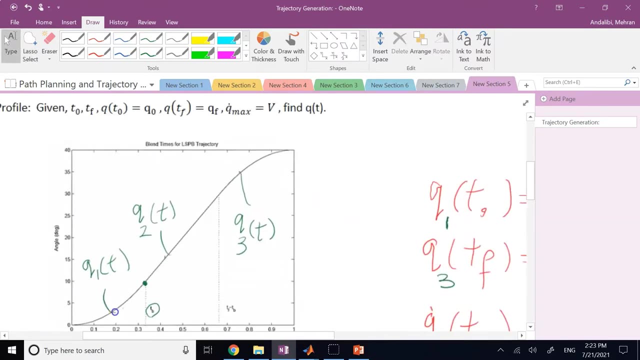 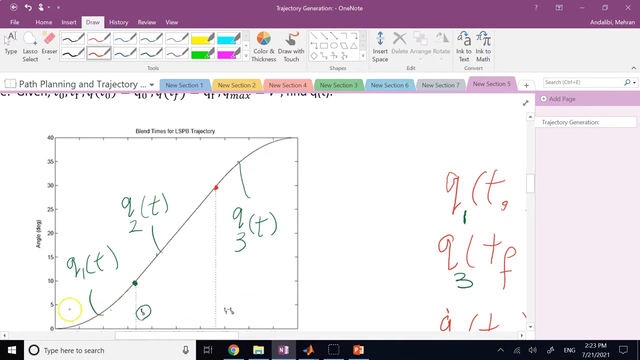 then, by the way, one correction here. the correction is the next time point that the blending is happening here. this point, this is not T blend, this is T minus T blend. and because the whole thing is symmetric, okay, so if the left hand side is T blend, the right hand side also, this distance should be T blend. so 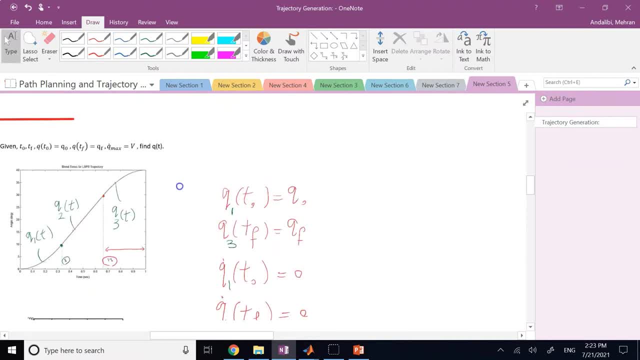 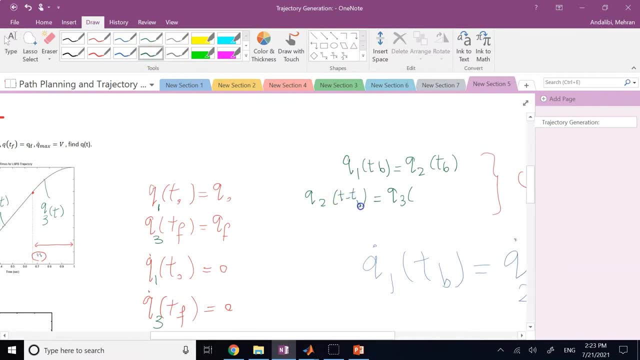 they should be equal to the slope of the first function, q1 at the T blend. so But the time point is T final minus T blend. So you have to say Q2 at T minus T blend is the same as Q3 at T minus T blend. 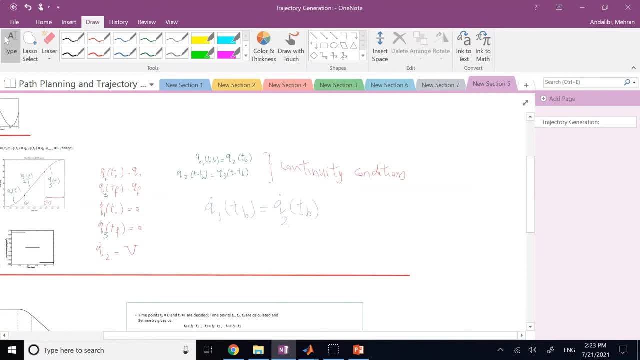 Okay, you need that. And then I have, as I said, Q1 dot at T blend is the same as Q2 dot at T blend, And Q2 dot at T minus T blend is the same as Q3 dot at T minus T blend. 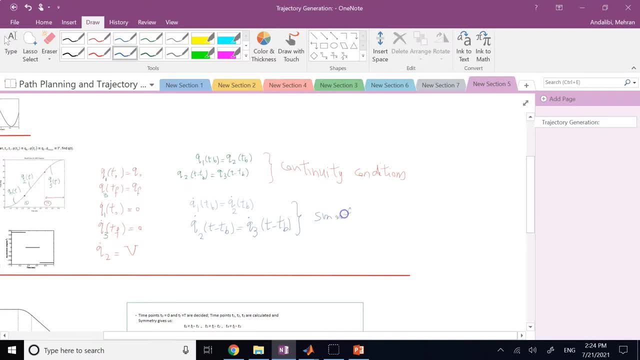 These two I call smoothness conditions. So so far, So so far, So so far. So, if you have seen, I have eight, nine equations, right, Nine equations. What are my unknowns? There are eight unknowns: the coefficients of Q1,, Q2, and Q3, and the T blend, correct? 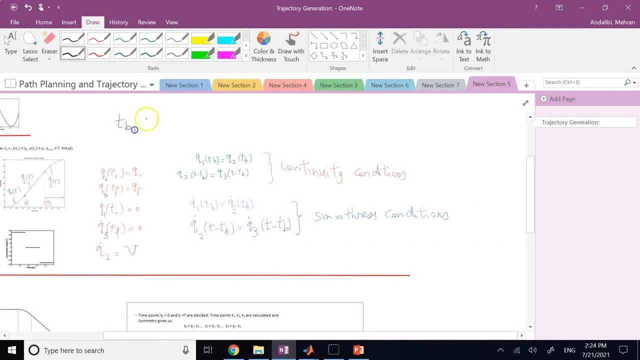 So I have T blend as well as my Q1 of T. if you write it as A1 plus B1T plus C1T squared and Q2 of T, you write it as, let's say, D plus E times T. 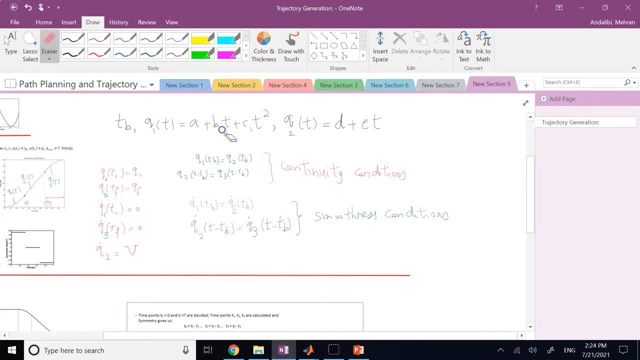 And let me get rid of these ones for here, because I don't need them really- And your Q3 is like F plus G times T plus H times T squared. So you see I have. I have nine unknowns. This is one, three here, two here and three here. 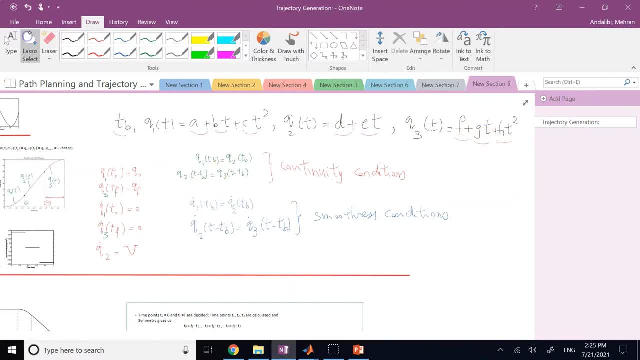 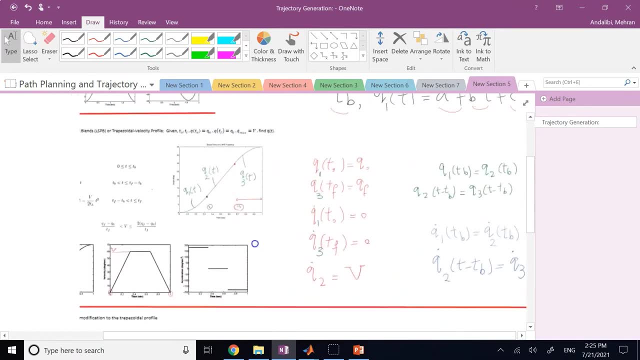 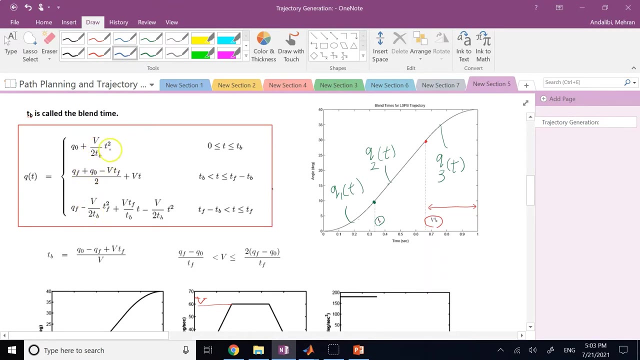 Nine unknowns and then I have nine equations, as you can see, And I should be able to solve the nine equations with nine unknowns, which, if I do, I will get this criteria for Q1, Q2, and Q3, correct. 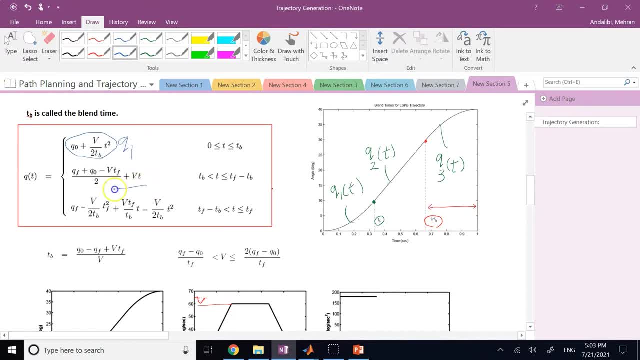 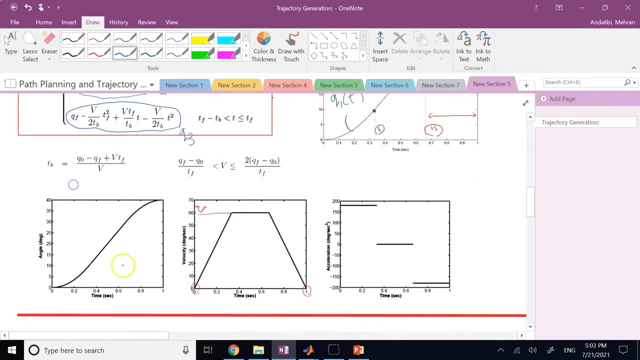 So this is your Q1.. This is your Q2.. Q3. And this is your Q3,, where each one of them is only valid for a specific time period. First one, between zero to time blend, As you can see. the next one is between time blend to T minus time blend. 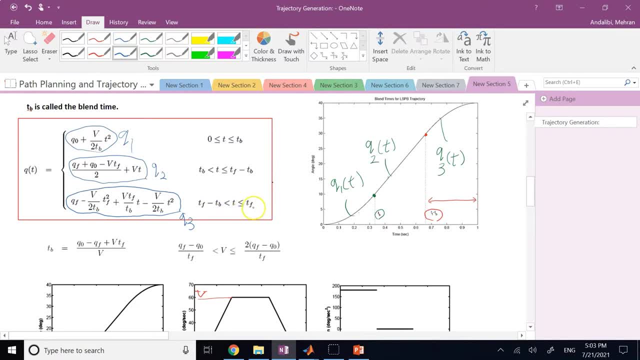 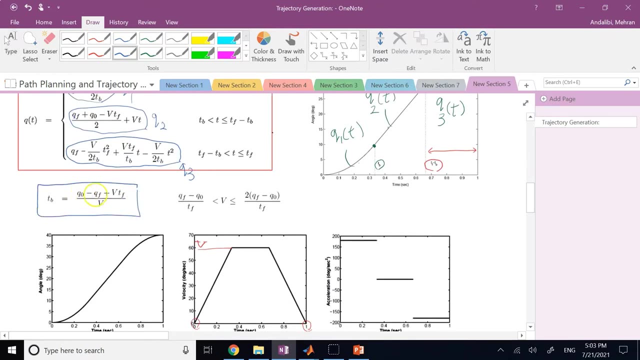 and the last one between T final minus T blend and T final. Okay, Now, not only you get all of these eight coefficients- as I said, T blend is one of your unknowns- and you can also solve for T blend, which is going to be Q initial minus Q final plus VT final divided by V. 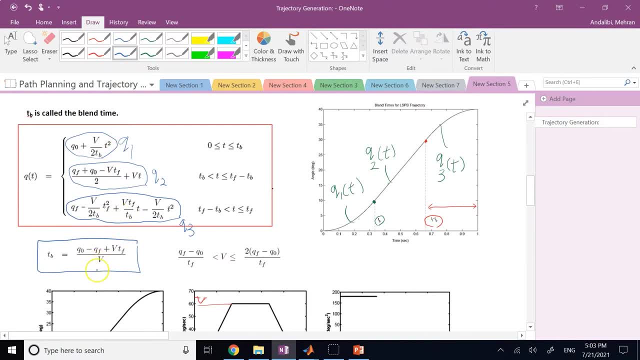 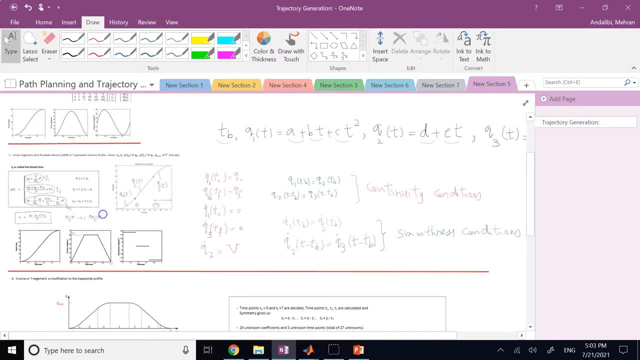 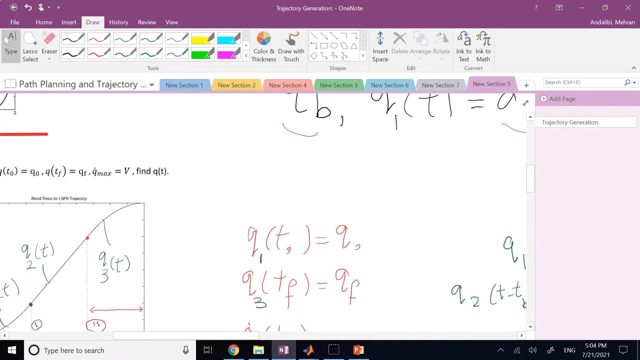 So here are the solution to the nine equations and nine unknowns. And if you check them you see clearly all of those nine conditions are satisfied, correct, Like for example at: T of zero equals zero. here your T naught is equal to zero. okay. 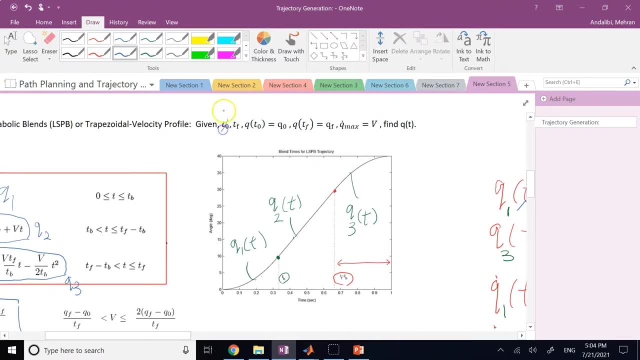 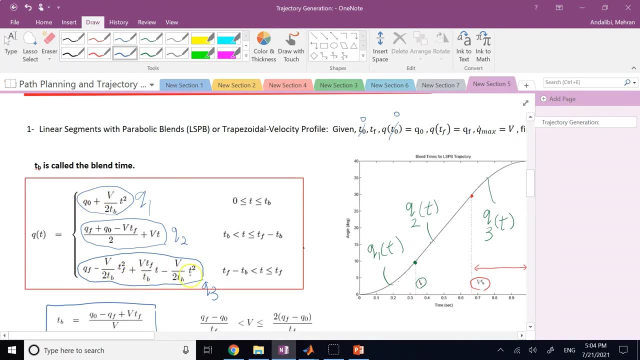 At T naught equals zero, You have the value to be equal to Q zero. if you plug in T F here in this last one, correct and simplify, then these two negative one-half terms with this one positive full term would go away. 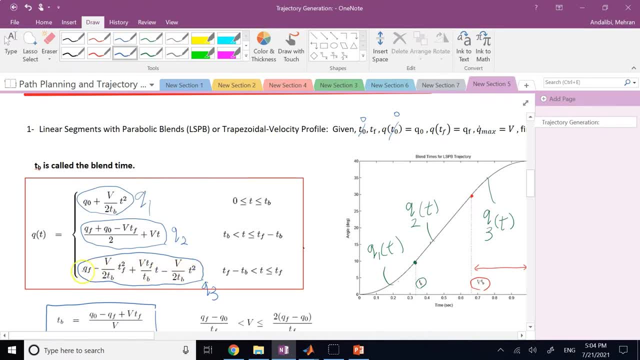 So all of the three terms would vanish. simplify together, you'll get your Q F. If you look at the slope Q dot at time T- zero, clearly it is going to be zero. If you look at the slope Q dot at time T F, again you can easily show. 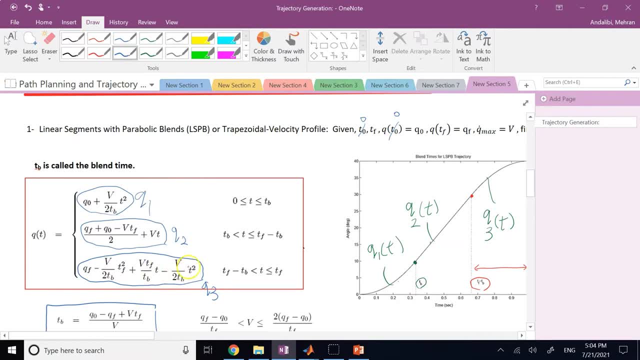 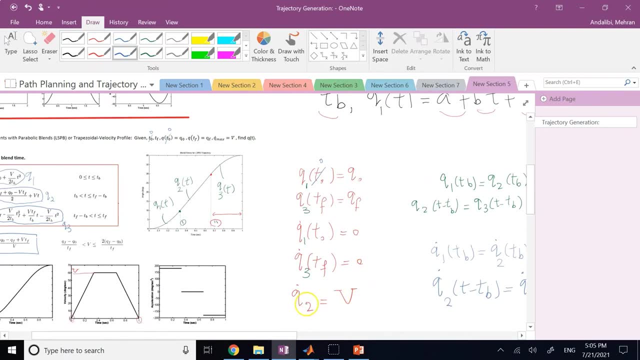 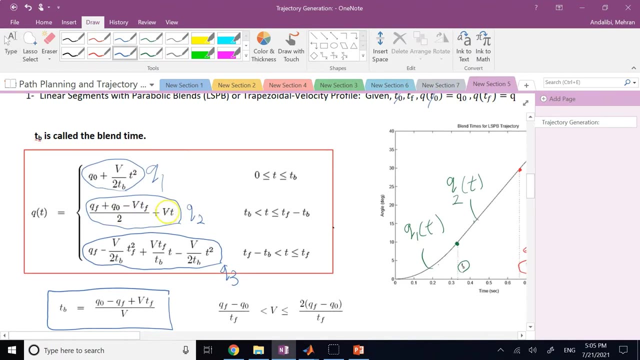 that it's just these two terms that have time derivative. Again, it is going to be zero. So all of these four conditions are satisfied. If you look at the middle function, Q two, the derivative of that is V. Clearly you see, it's a linear function and the slope is V times T. so V is the derivative. 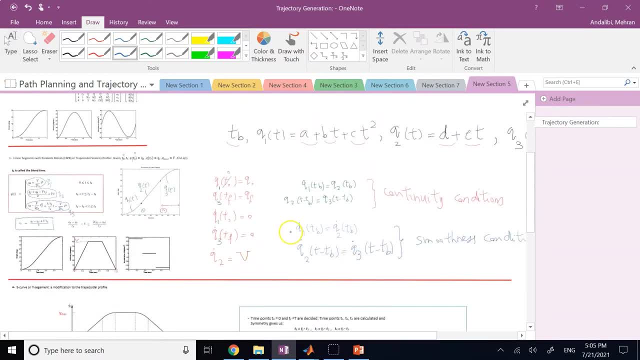 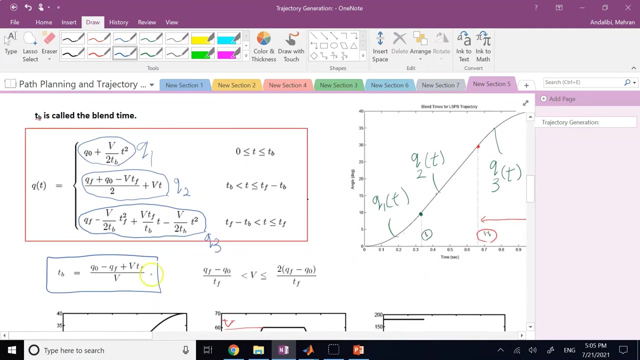 So the fifth condition is satisfied, and then, clearly, when you plot these functions, you have the smoothness and the continuity conditions. okay, So everything is basically taken care of, right. So this is the solution. This last one gives you a value for T blend. so when you want to start using this, 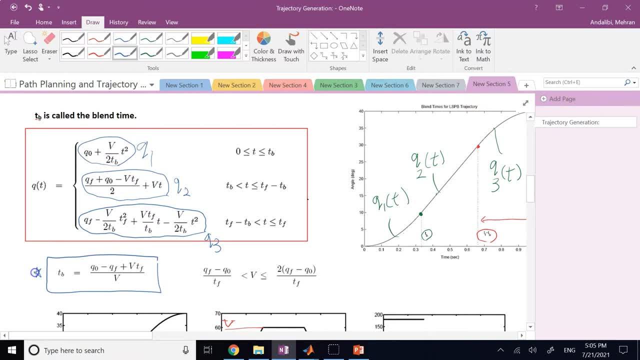 the first thing you do is you do this. Okay, The first thing you have to calculate is actually T blend. Once you have that, then you can plug it into the first one and the last one. So before you can calculate these coefficients in this Q one, Q two, Q three, 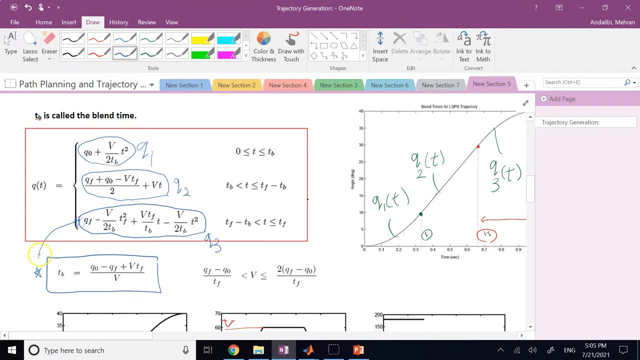 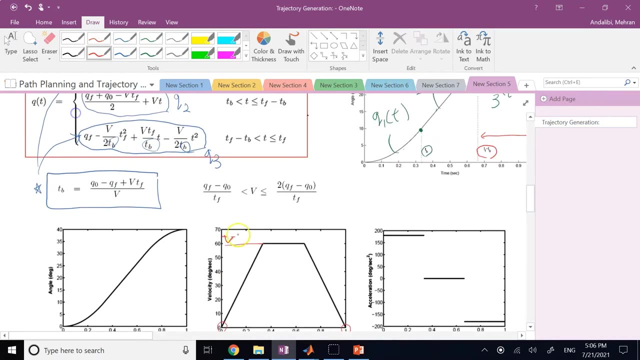 first you have to calculate T blend, because you need it in Q one and Q three, as you can see here Right Now, here there is also a limitation On this V max. okay, This V that you have, V max, it has some limitation. 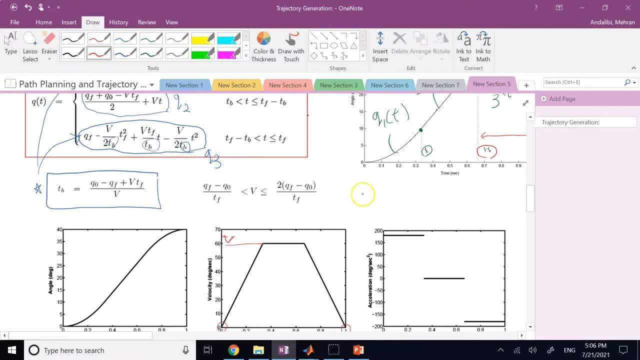 You cannot just choose it to be anything, Because your T blend is bigger than or equal zero and it is less than or equal T final divided by two or less than actually in general. if you make it equal to, it means there is no period of constant V. 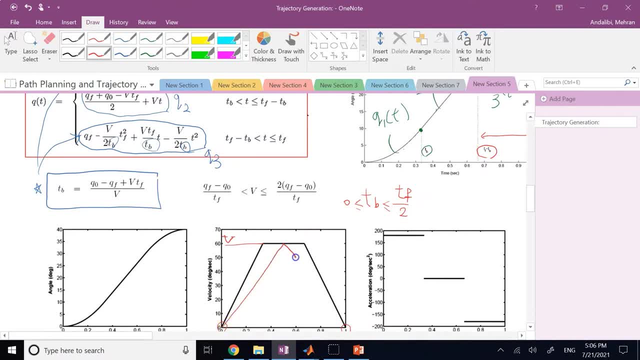 You directly go up like this and you directly go down like this. okay, There is no time during which V is constant. when T blend is equal to half of T. final, When you make it zero, it means literally you are going straight up and then the whole motion is constant. 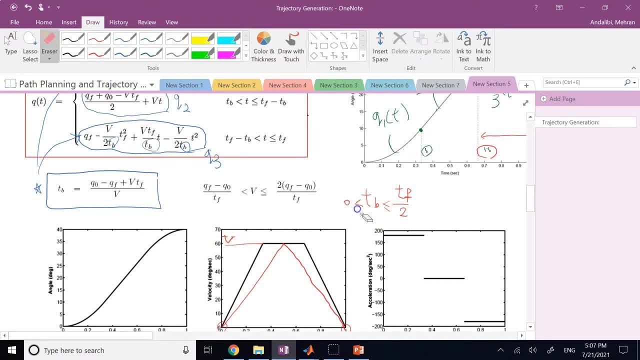 So really, if you want to be realistic, the equalities here are not really appropriate. It has to be less than that and bigger than zero. And so if you now set this to be equal to bigger than zero and then less than Tf, right. 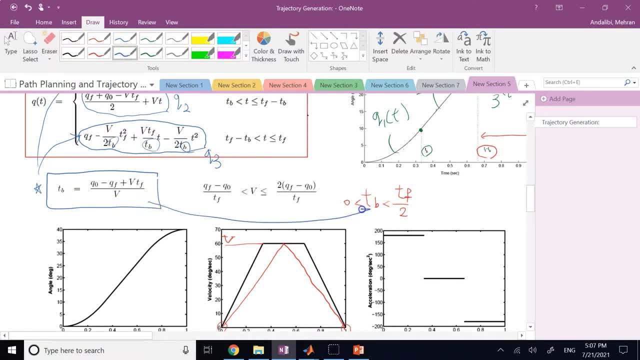 So that formula for Tb, if you plug it up here then it leads to this inequality that you would see here, That your V cannot be anything that you desire. Your V has to be bigger than the delta in Q, Q final minus Q unit. 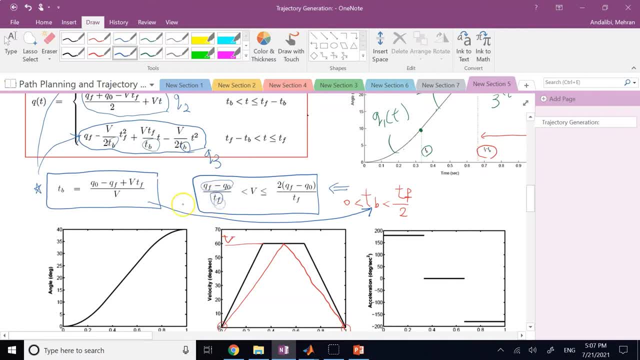 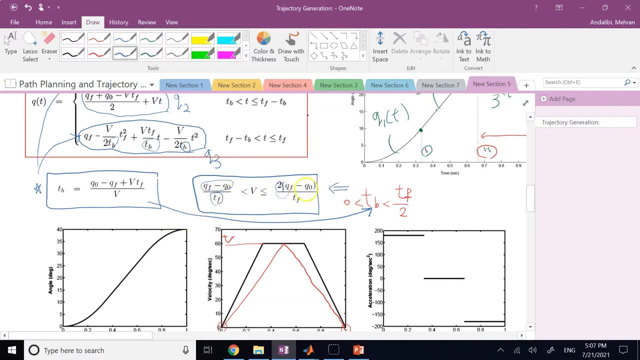 Okay, Okay, Okay, Okay. And it's less than or equal to times that quantity. So this delta Q over delta T, One times that and two times that, anywhere between one and two. it should be what Your V. it cannot go like to be three times that or 0.5 times that. 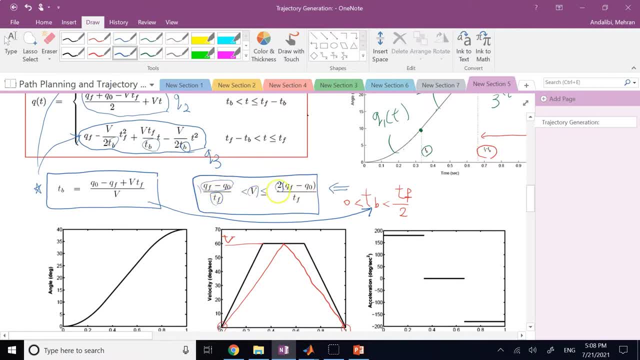 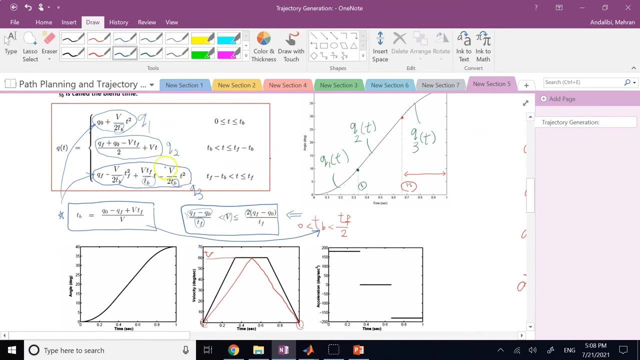 It has to be between one time this delta Q over delta T and two times delta Q over delta I t, and so that gives you a choice for v because v. you clearly also see that you have limitations on v, and this v is used in all of the formulas. so before you do that as well, you have to go through. 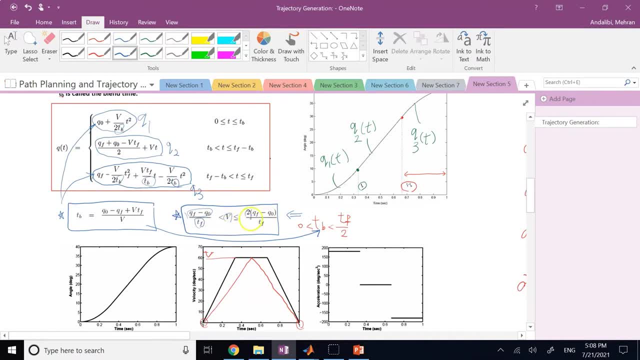 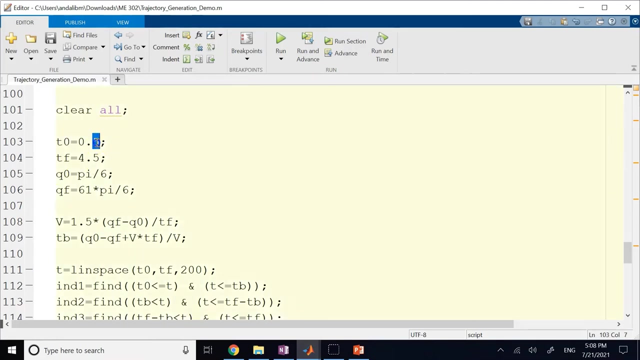 this one as well. you have to choose a value for v based on the q, not q f and t f. then once you have these guys, you can go and determine your criteria right. and here i wrote a math lab code based on these formulas. if you can see, here i have some initial time. you can choose it to be zero if 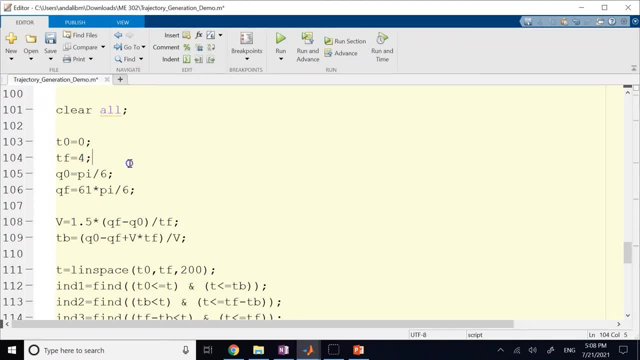 you want, i have some final time. i have some initial q, some final q. here you see my v. i have chosen it between one and two. i chose it to be one and a half times delta q over delta t. t of b is calculated based on the formula. 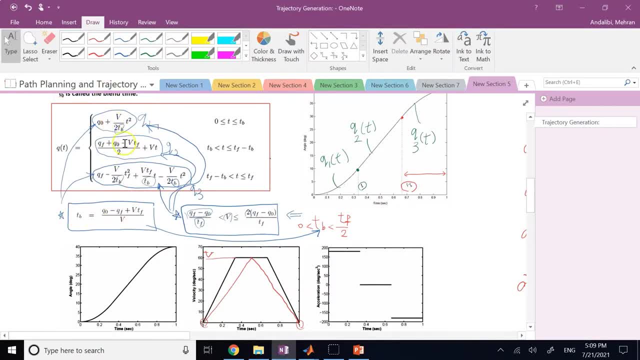 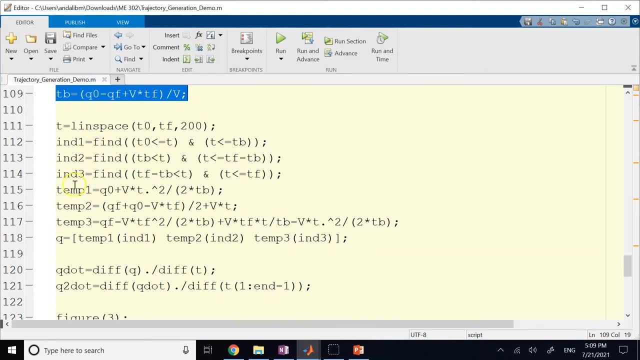 you just saw here, and then, based on that, i created my q1, q2 and q3, which here i called actually temp 1, temp 2 and temp 3, and then the combination of them i called what q. okay, so if i want to, instead of temp 1 i can call it q1, right, so it's not a big deal. or i can call this one q2 and i can. 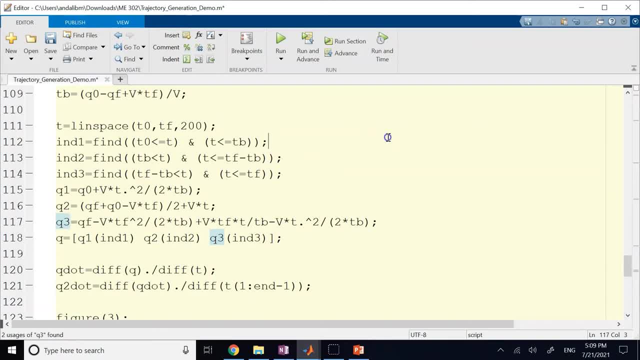 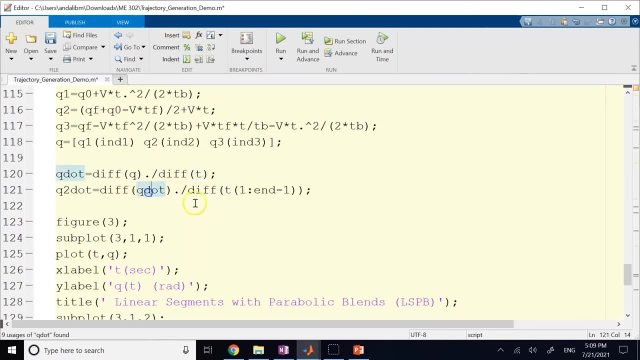 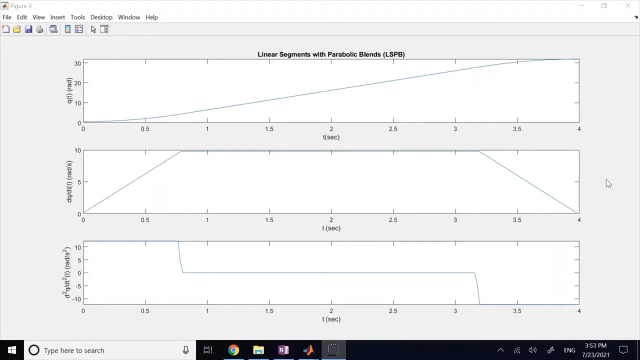 call this one what q3. so i form my total q, i calculate my q dot and q double dot using numerical differentiation, and then what? i can plot it for you. okay, here is the result. as you can see, the joint variable is basically a parabola, as you can see, then followed by a line and then another. 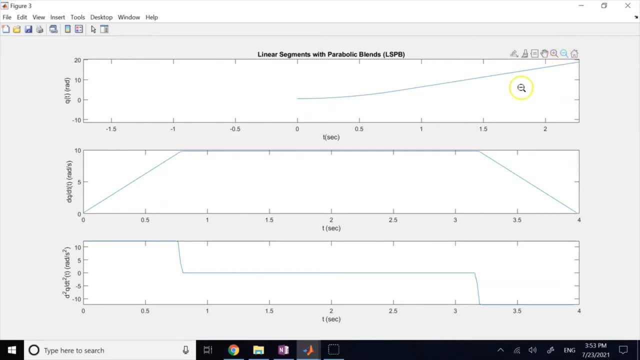 parabola, right, so it is a linear segment in the middle with two parabolas on the ends. it's blended with them, so we call it lspb. or if you look at the velocity profile, you clearly see it is a trapezoid. and also if you look at the acceleration, you see the step type. 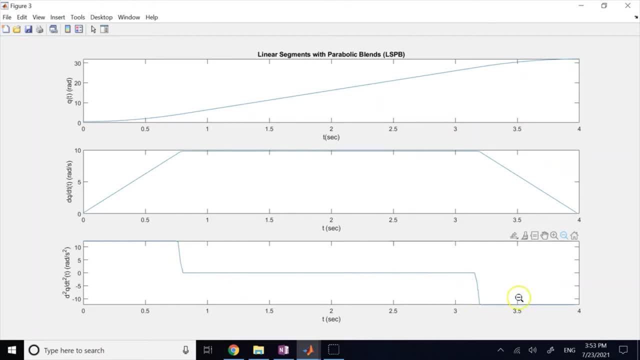 behavior. it jumps from a positive number to zero to negative. okay, so this is our lspb, or trapezoidal motion that you can see, and the main problem with this type of motion is this: jump in the acceleration. when you have a step type, jump in the acceleration. 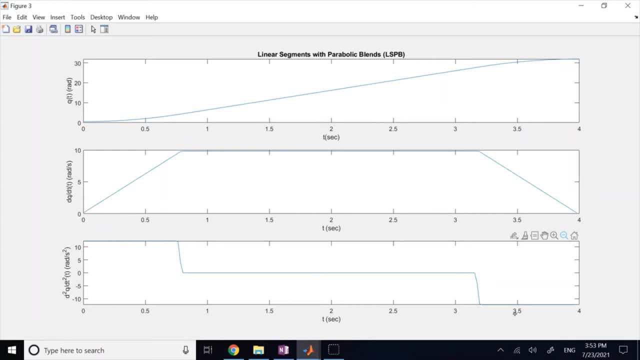 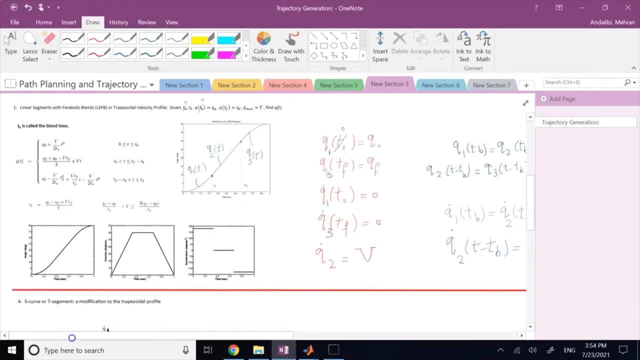 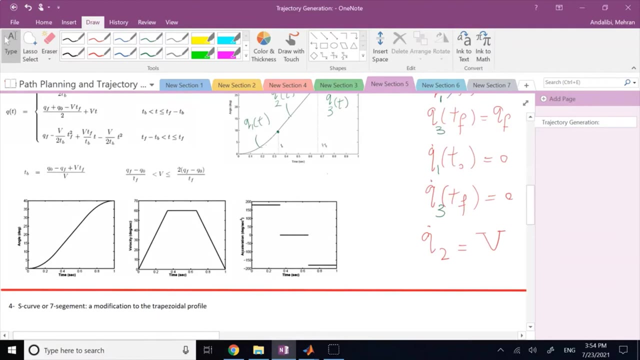 the derivative of the acceleration that, if you remember, we call jerk and it shows the uh, sudden changes in the forces, right, it shows it's an identification of impact, basically in your system, if you have that and calculate it. so jerk is equal to d of q, double dots. 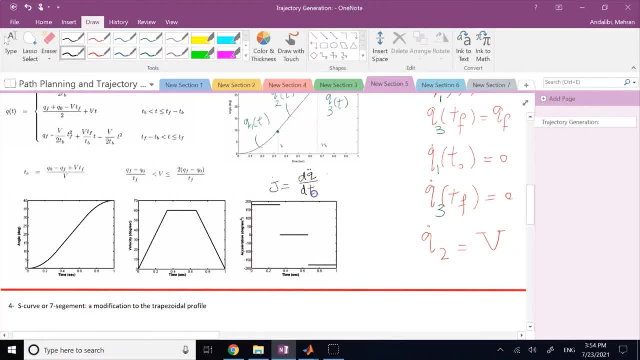 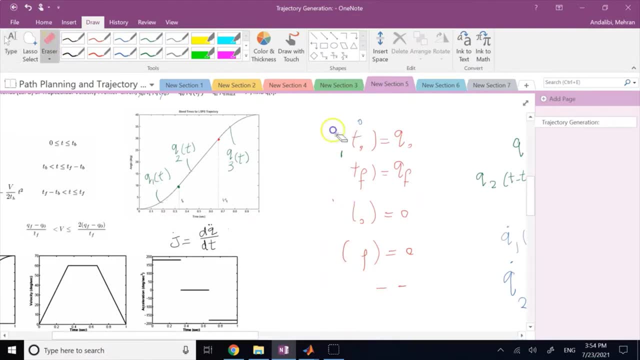 right, the joint accelerations over time. if you plot it so, um, let's say here, for example, it tends to be at any point it is going to be zero. but when you have those sudden jumps, so if this is t, this is j, you see this is going to be like zero and zero, and then zero, and then 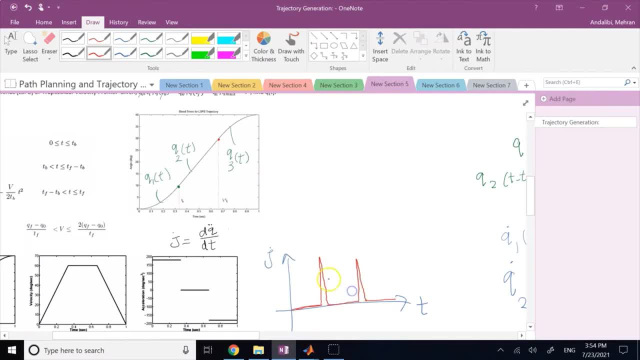 here you have a big spike and another big spike, and these are kind of like impacts that are on the links of the robot and those are going to affect the useful life of the robot and they are going to make the motion non smooth in general. you see, 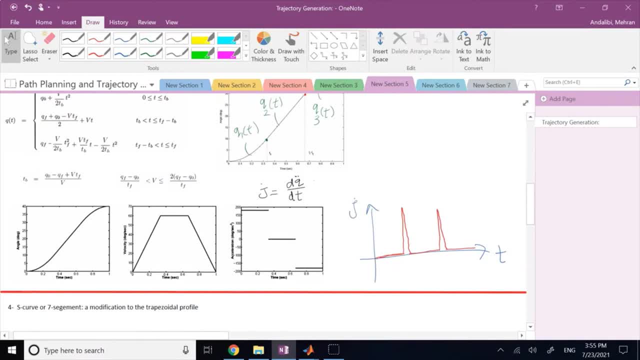 jerky kind of behavior- so large jerks- is not a good idea. that's why there is another version of this trapezoidal velocity motion that is a little bit modified. and what you do? you try to get rid of this. sharp corners in the velocity and as well here. so you go with the parabola here a line another. 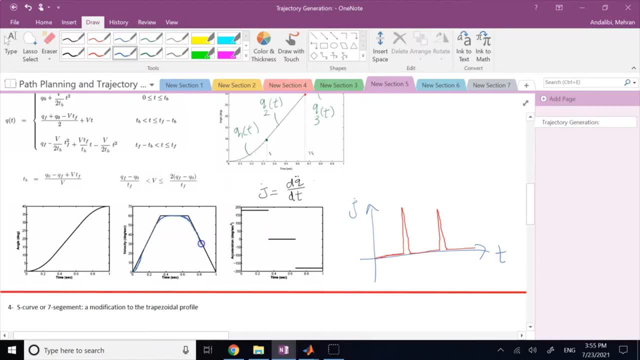 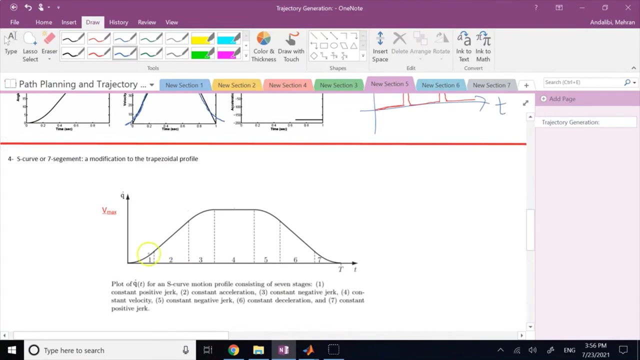 parabola, straight line parabola. then you go straight line and then again you go with what? another parabola? okay, so this kind of kind of smooth version of this trapezoid is what we call s-curve, which you can see here. so if you plot the 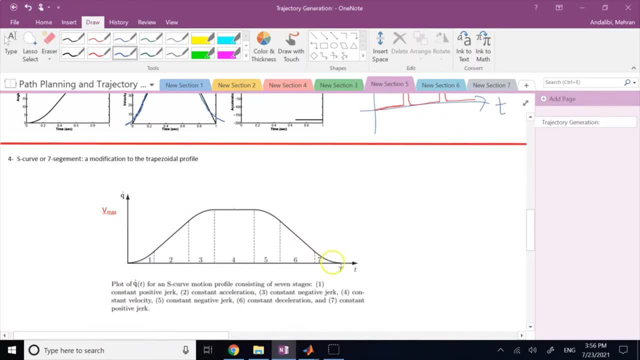 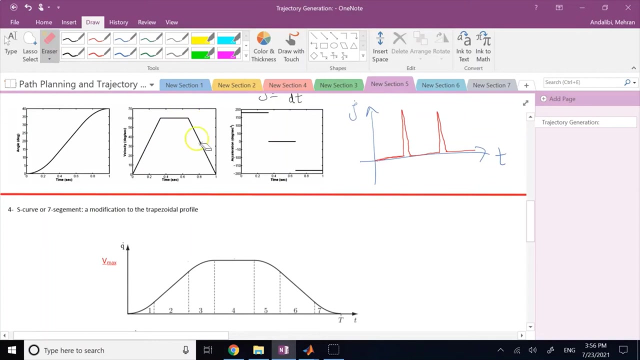 joint velocity versus time. it is a trapezoid, but at the sharp points you have what you have: a rounded feature, which means a, a. I have constant acceleration. again you have jerk, but negative jerk this time. so acceleration is decreasing. it's basically gonna go down until it goes. 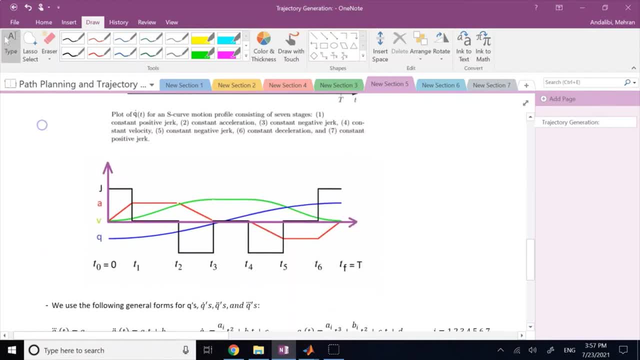 zero here and then here drops. so if you look at the profiles for velocity, acceleration and jerk- these are the four plus that you see. the green one is that modified trapezoid or s-curve that we mentioned. if you look at the acceleration, you go with the trapezoid and then you go with the acceleration and then you have. 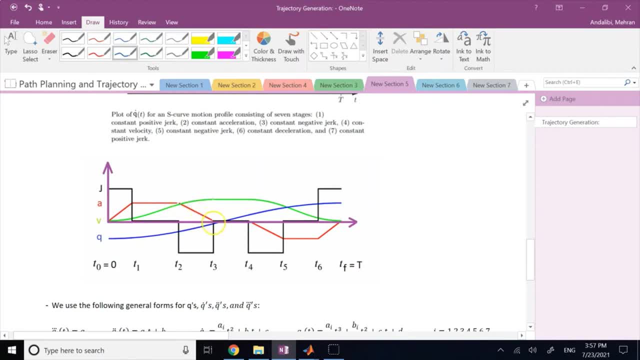 0. acceleration to zero, yes, and you start to go up linearly, then you stay constant, then you go down linearly to 0, then they stay at zero, and then exactly the opposite of that: you go negative, you go constants negative. and then what? this is where you are dropping your velocity and then you go to zero. 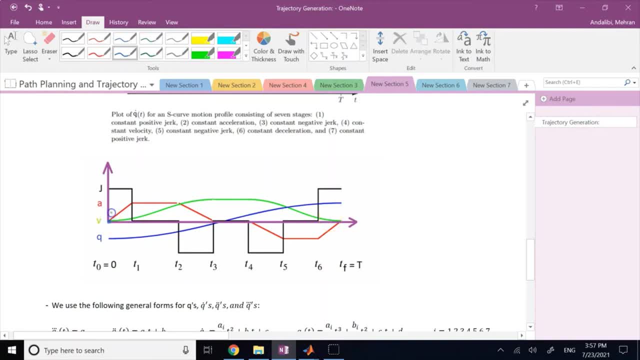 ok. so you start at zero velocity and you end up with zero velocity. the same thing: we acceleration, you start with zero acceleration, you end up with zero acceleration, Greg. so we start from 0 speed, you end up with what that velocity, rest and go to rest. basically, your start angle can be zero or non-zero and your 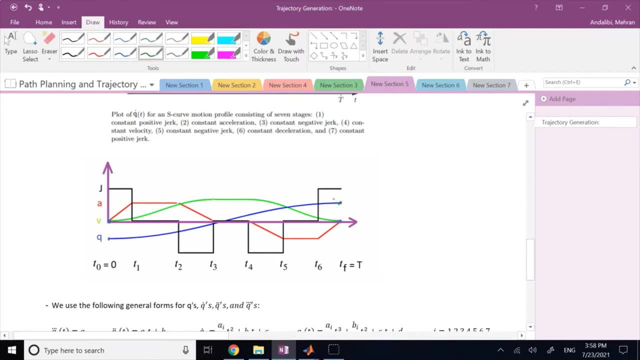 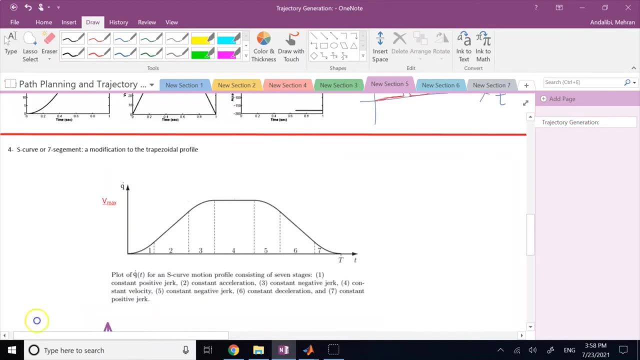 final angle is whatever you want to rotate, and if you look at the jerks now, you have some positive jerk, zero jerk, negative jerk, zero jerk, negative, zero and positive jerk. so the motion consists of seven separate parts, despite the previous one being just three parts. if you remember right, you had part one. 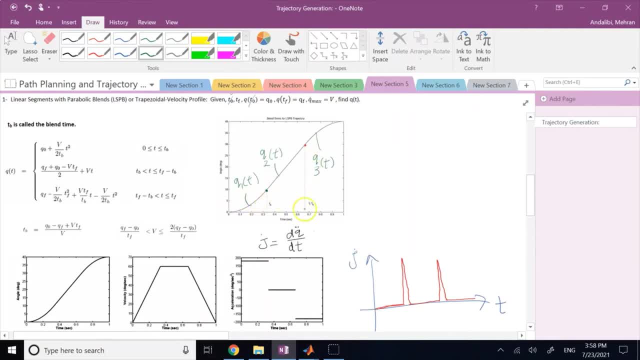 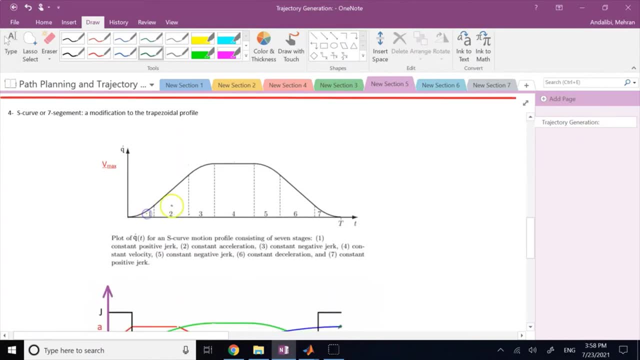 between zero to T blend, between T blend to T minus T blend, T final minus T blend and then T finest minus T blend and T final. so you only had three segments. now your motion has seven parts, so that's another name that they call. they call it a seven segment profile, okay, and here I'm gonna show you a. 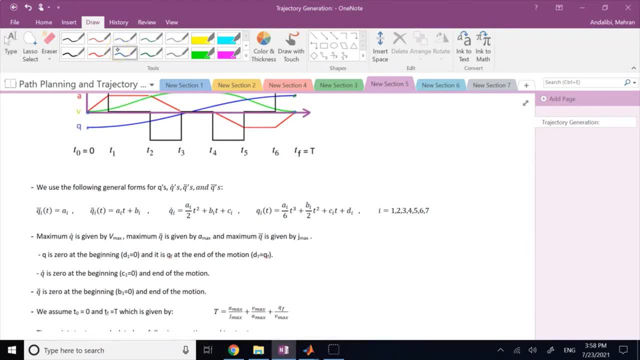 formula for that as well, which I derived. so what I will do here is, I assume, a general cubic form for the joint variable, which means a quadratic form for the joint velocity, which means a linear form for joint acceleration and which means a constant number for the jerk. okay, now, in some cases the jerk is zero, like between: 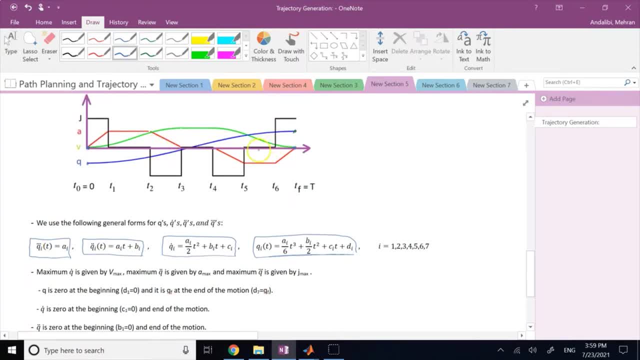 T 1 and 2, between 3 and 4 and between 5 and 6. for all of these cases jerk is 0. for some cases the acceleration is also 0, like between T 3 and T 4. okay, velocity is never 0, but in one range it is constant, and that is between T 3 and T 4. okay. so 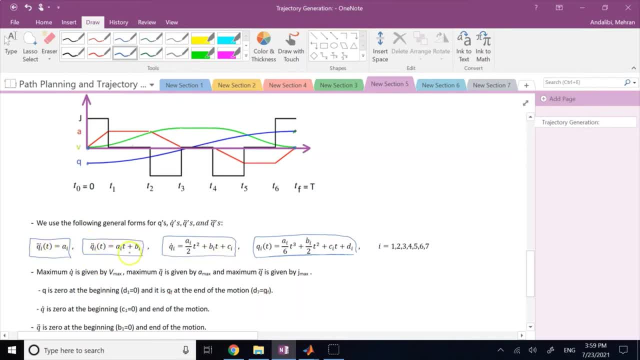 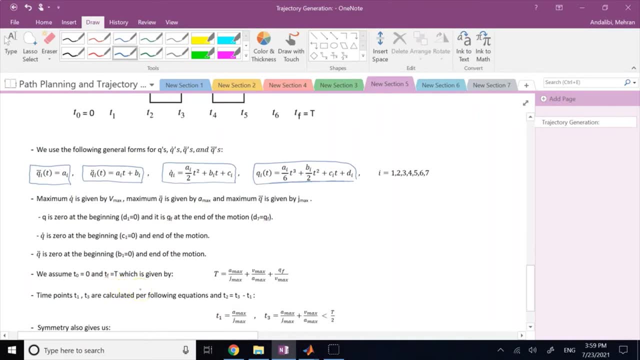 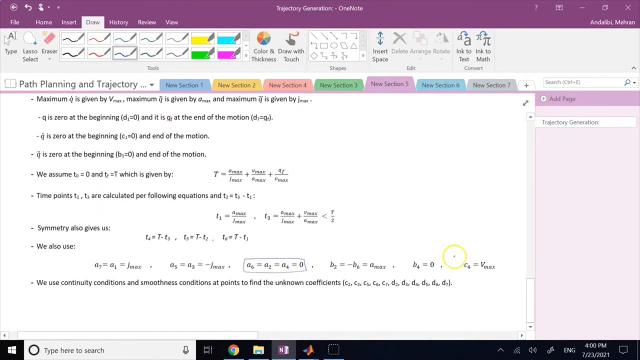 some of these A's or B's could be 0. as I said, three of the A's that I guess I mentioned them in my notation. if you look you have your a, two, four and six. all three of these are 0 and among B's is only before the middle be the B for the middle motion between three. 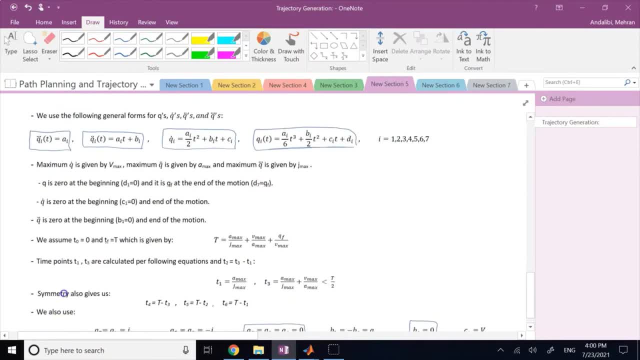 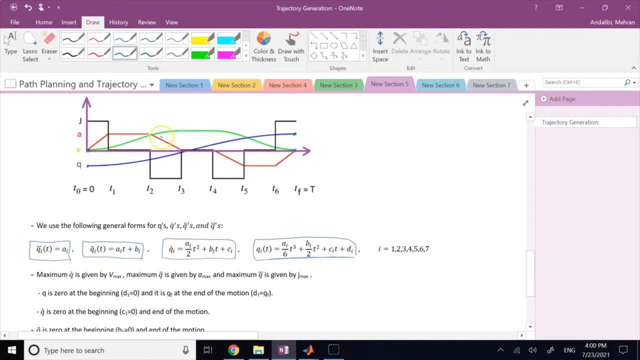 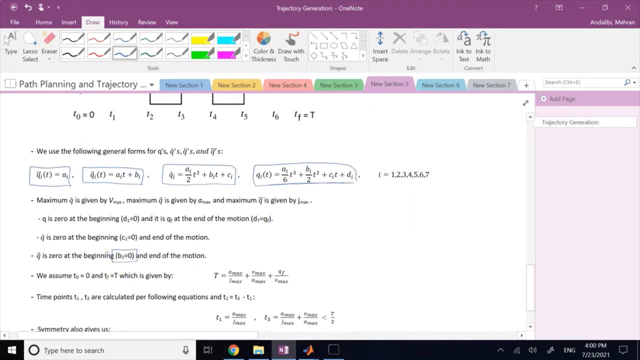 to four, that is 0. the C's are not zero. now we start from zero velocity and zero. what acceleration? what does that mean? it means B one is also zero and Right, the acceleration term for the constant of the acceleration term for the first motion. that's your initial condition. it has to be zero in addition to B4.. 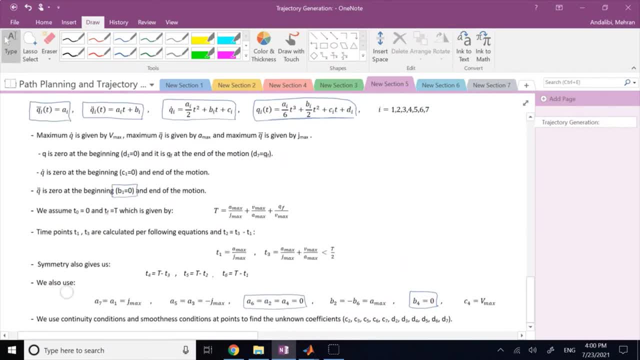 So not only B4 is zero, B1 is also zero because we chose to start with zero acceleration. Your initial velocity, we assume, is zero. that means C1 is zero and your Q initial is zero. Now you don't have to choose your initial angle to be zero, but since you can measure everything from the Q initial, you can for simplicity assume that the Q initial is also zero. 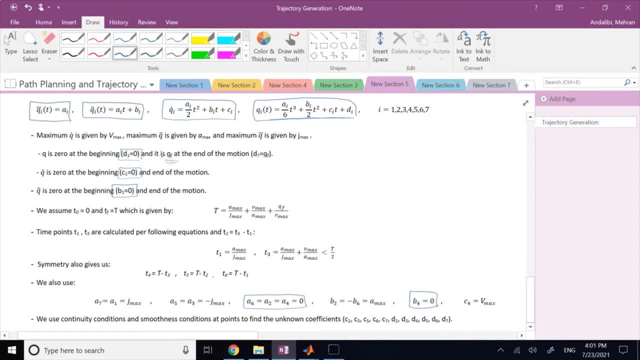 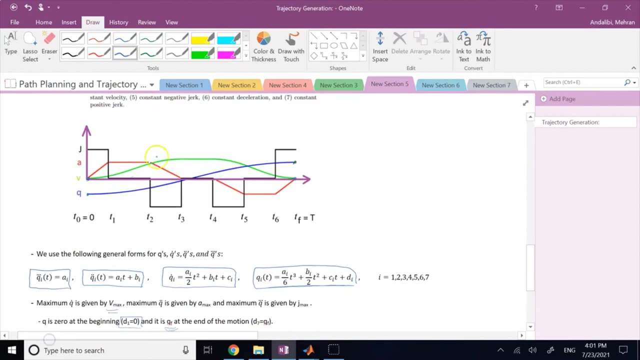 Q final is definitely not. that's the angle you want to rotate through The final time. here we show it with capital T. the initial time is zero. Now, what you can see there here is three constants. One is the maximum velocity, just like the previous case, correct? 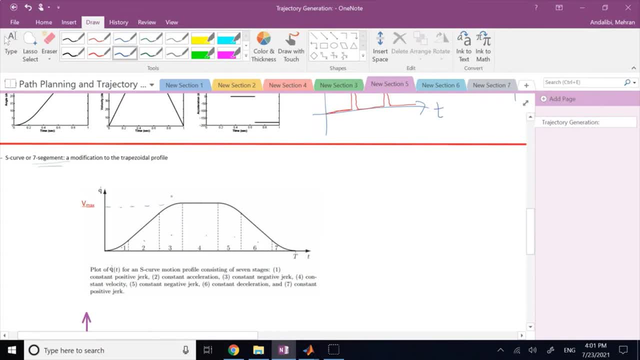 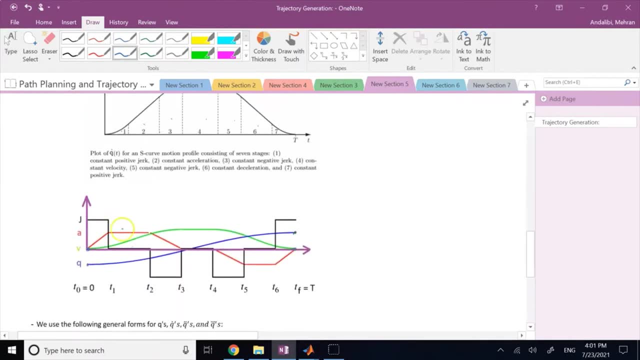 This Vmax. this is the maximum, the fastest that your motor or linear actuator can move or rotate. You also have some maximum acceleration, which you can see here. this is your Amax right, Which comes from your motors again, how much torque they can generate or how much force they can generate. 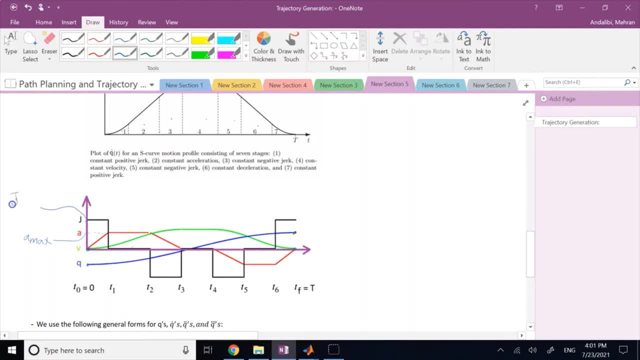 And you also have another parameter to choose, and that is maximum jerk right, How much jerk your system can tolerate, How much impact can it tolerate without mechanically failing? So Vmax and Amax comes from your actuators, Jmax comes from your physical system. really, 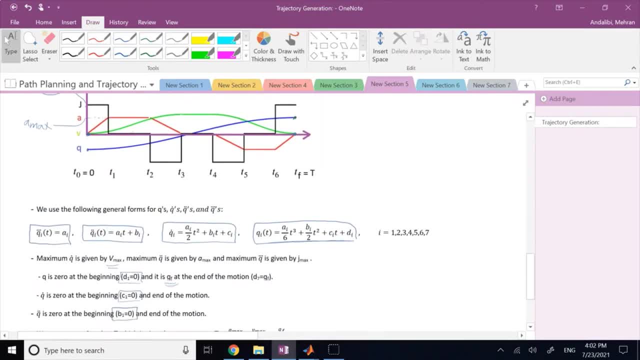 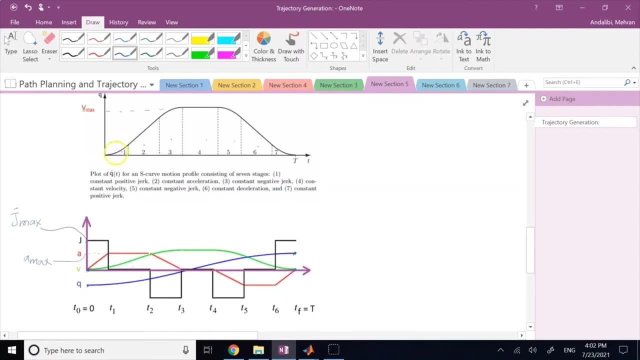 Okay, so here you choose the three parameters Amax, Jmax and Vmax, And based on that you can easily find the criteria for each one of the Qs In general. here you have seven Qs, right, You have Q1, Q2, Q3, Q4, Q5, Q6 and Q7. 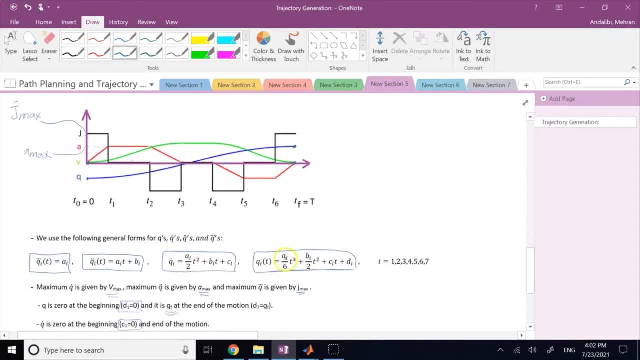 And each one of these Qs, as you can see, it has four coefficients: A, B, C and D. So you have 7 times 4, that's 28.. There are 28 coefficients to find And also you have to decide about the time: T1, T2 and T3. 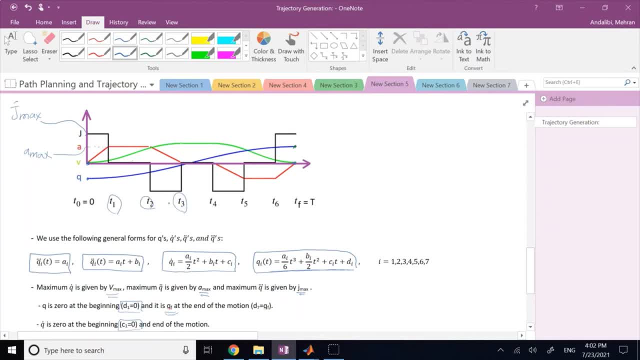 Okay, you have to find them as well, And I'll show you not only that, you actually need to also find your final time as well. So there are, in general, 32 unknowns here, But don't worry, I've gone through all of them and I solved this. 32 unknown, 32 coefficients. 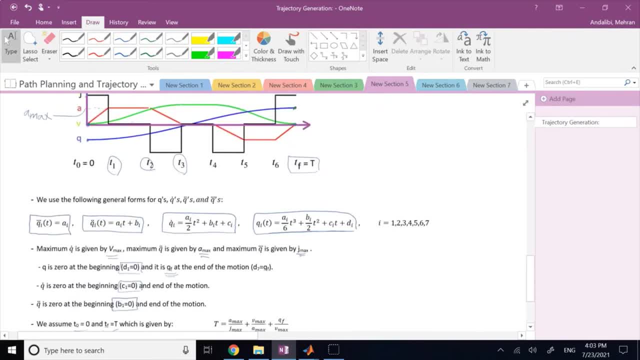 It wasn't easy but I did it And here I can show you, If you choose your Vmax, Amax and Jmax, as I said, and your Qfinal. these are the four parameters that you have to choose, As I said, based on the motor, these two. this is based on the mechanical properties of the robot. link: 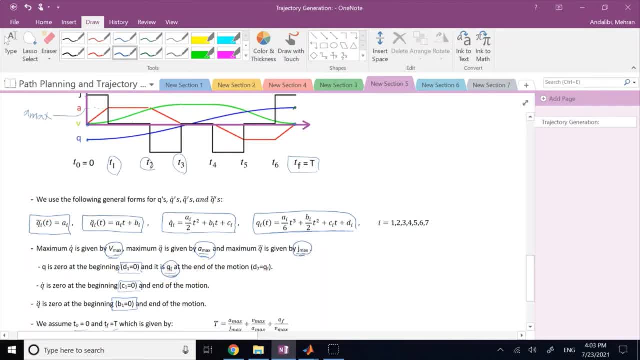 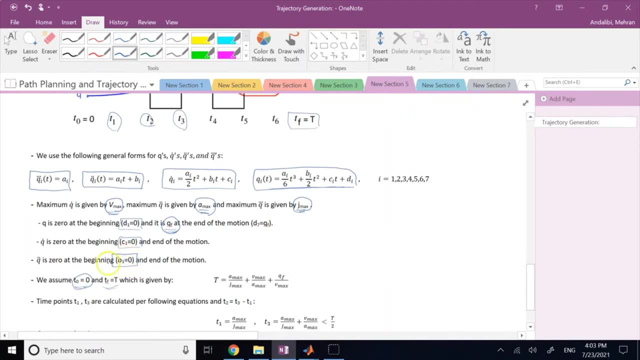 and Qf is the angle you want to rotate to. Okay, so you have four given numbers. Your initial time is zero. of course, in this case You assume the initial velocity and acceleration to also be zero And the initial angle. 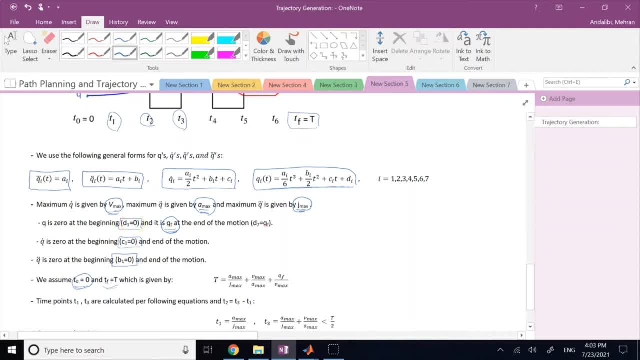 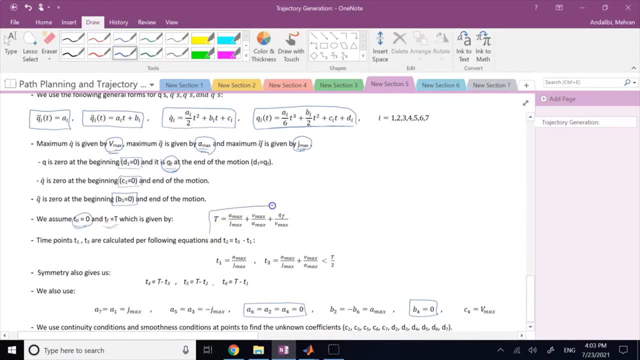 And then what you can do is you can determine your final time. Your final time can be given by this formula: Amax over Jmax plus Vmax over Amax, plus Qf over Vmax. Your T1 time comes from Amax over Jmax. 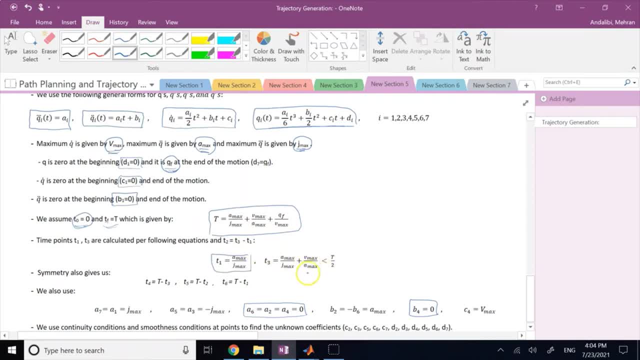 Your T3 is going to be Amax over Jmax, plus Vmax over Amax, And it has to be less than T over 2.. So if you choose this- Amax, Jmax, Vmax, such that this T3 that you get from this formula is equal, 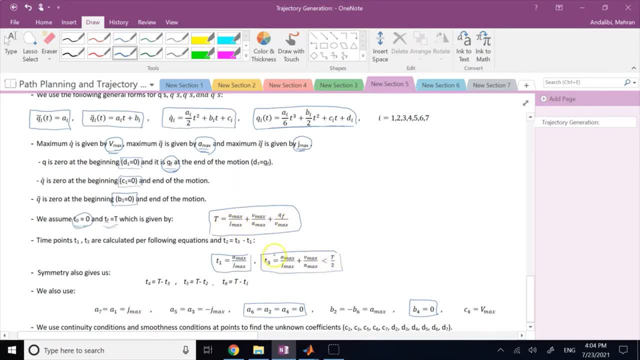 or bigger than half of this T that you found from the top one. you cannot achieve such motion Then the rest of the times you can easily find. So T2 is T3 minus T1.. T4 is T minus T3.. 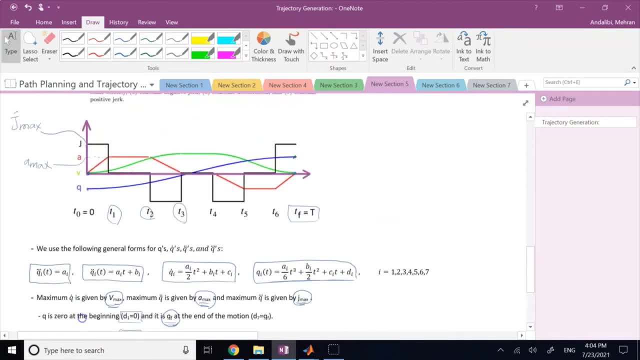 T5 is T minus T2.. T6 is T minus T1.. And that's all coming from symmetry here. So if you look All of this motion, except for Q, the rest of the parameters V, A and J. 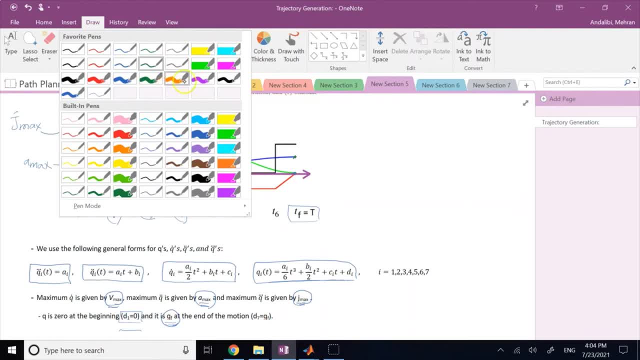 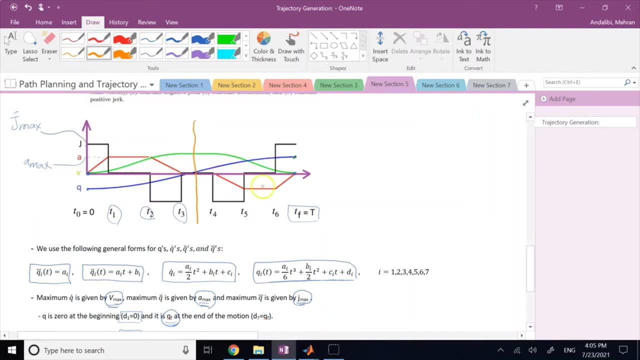 they are all symmetric about the middle point. So if you can draw the middle point here, a line like this- The V profile, the A profile and the J profile, The A profile- is not symmetric about the line, It's symmetric about the middle point. 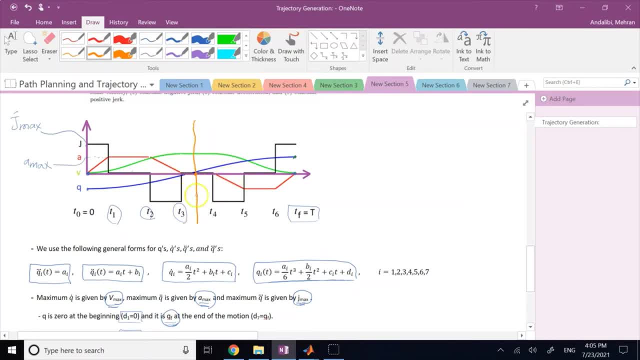 V profile and J profile. they are symmetric about what, They are symmetric about the line, but the A profile is symmetric about the point. So when you reverse it, when you mirror that from the left side to the right side, you have to also negate it. 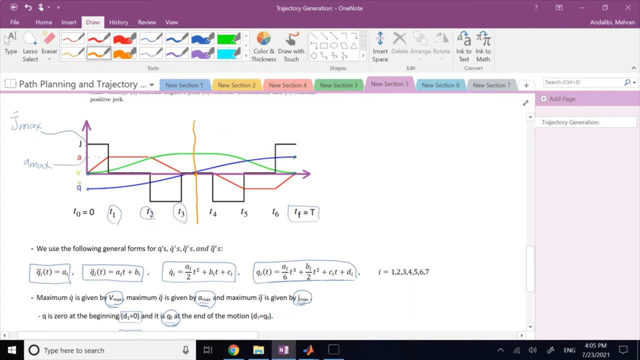 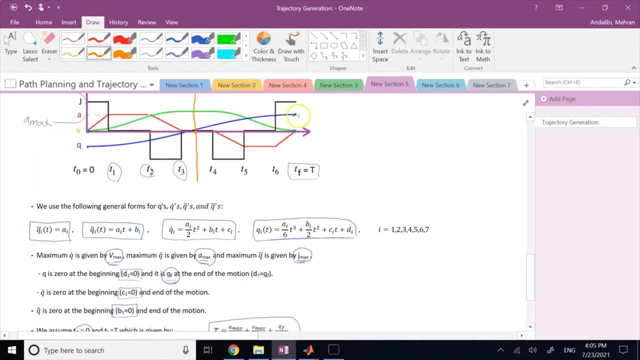 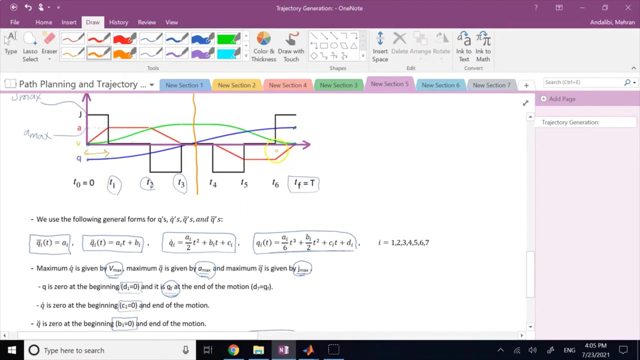 Q is not perfectly symmetric, okay, Unless you have your initial Q to be the negative of the final Q, then yes, you might get that also symmetric. Again, about the point, About the middle point. So using that you can say, for example, whatever distance I have here, I also have here. 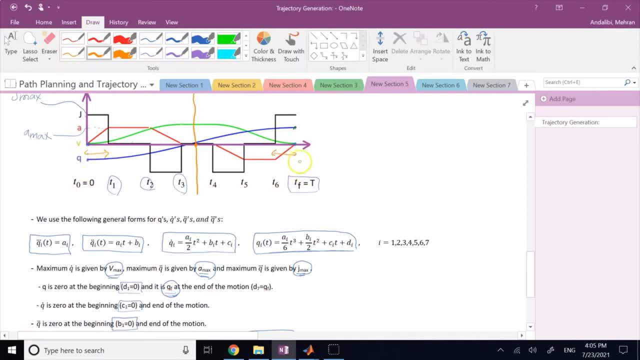 That's why if this is T1, from T1 to 0, then the last one should also be T1.. So it means T6 plus T1 is T final or cap T. So T6 is what T minus T1, right. 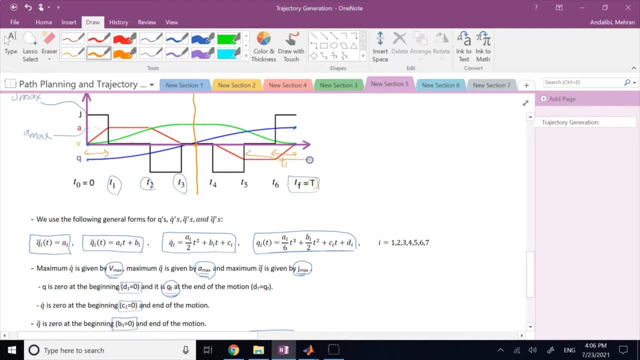 Or if this is like: from here to here all the way. Okay, So T2 is T2, which is the same as this one. So it means T5 plus T2 is again cap T. So T5 is cap T minus T2.. 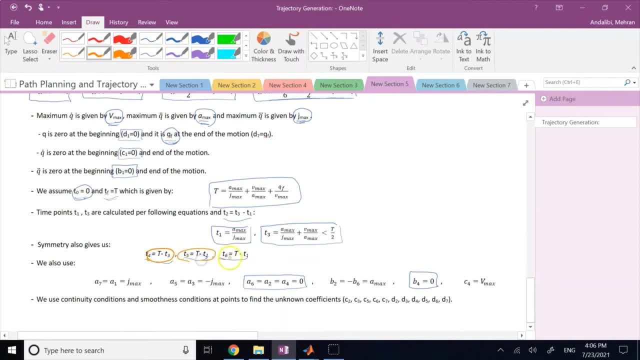 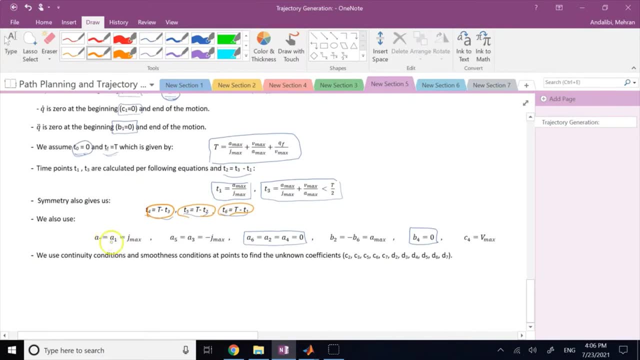 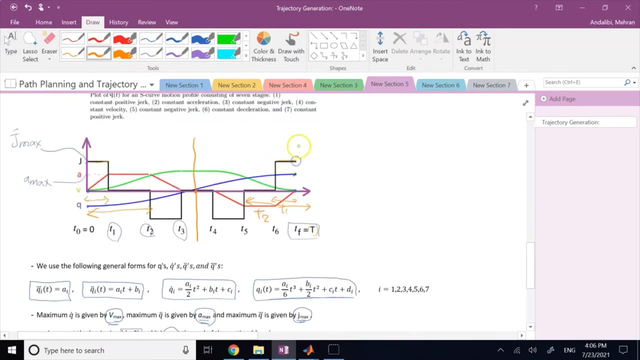 So that's where these formulas are coming from. Okay, And now your coefficients. the A's can all be given based on the J values, because you see, the J's are all constant. So J in the first motion and the last part of the motion are positive, J max. 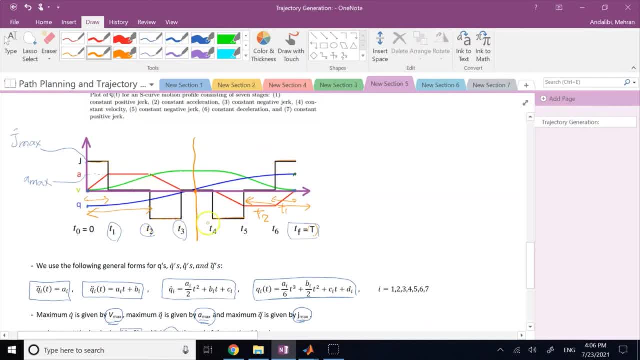 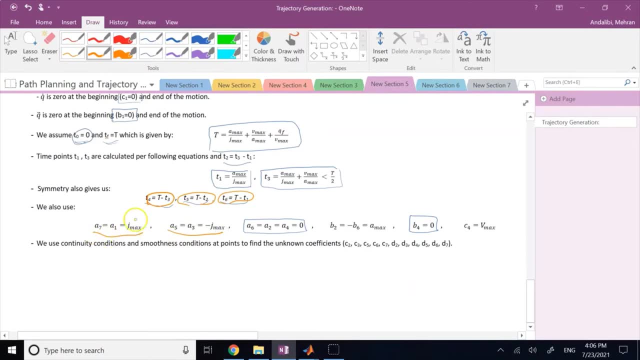 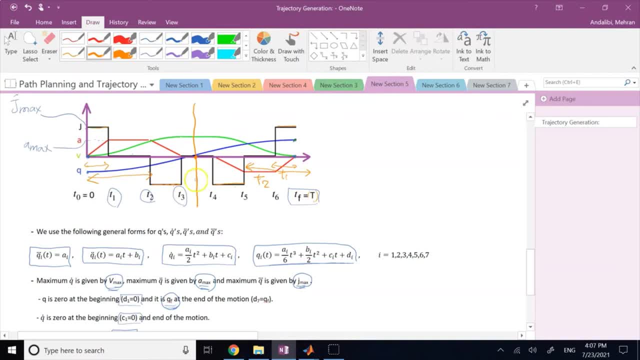 One of them can be less than the max in terms of magnitude. But here, to make it as symmetric as possible and make the calculations as simple as possible, we choose to go with max jerk in parts 1,, 3,, 5, and 7.. 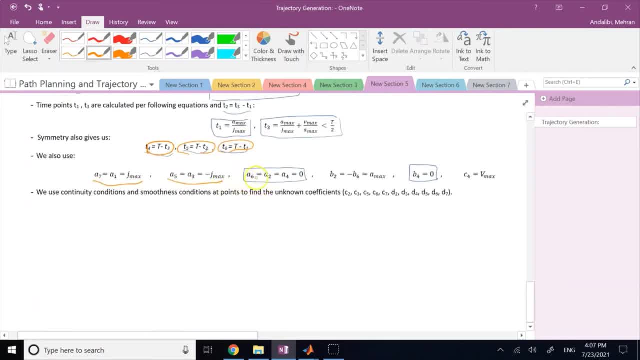 as i said, then a624 are all zero and these are all of your a's. so if you see, here i have given you all of your a's. you can start with these a's out of your b's. b4 is zero. that's given to you. 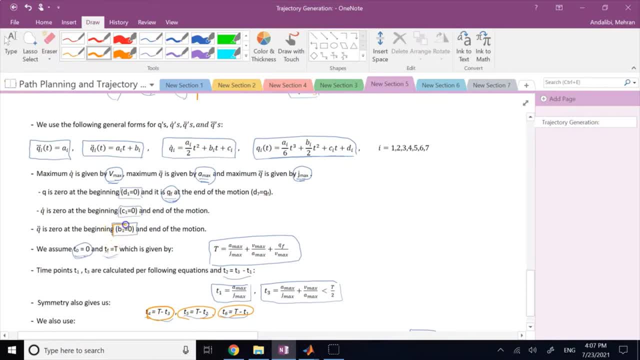 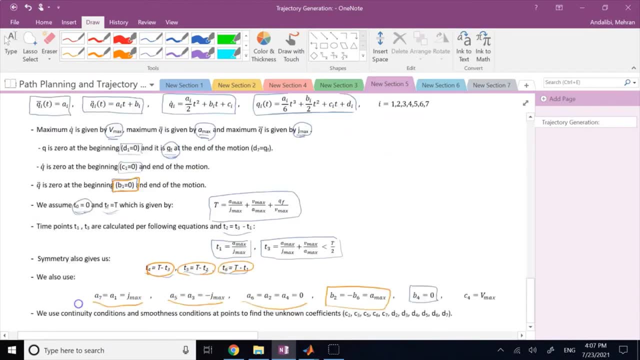 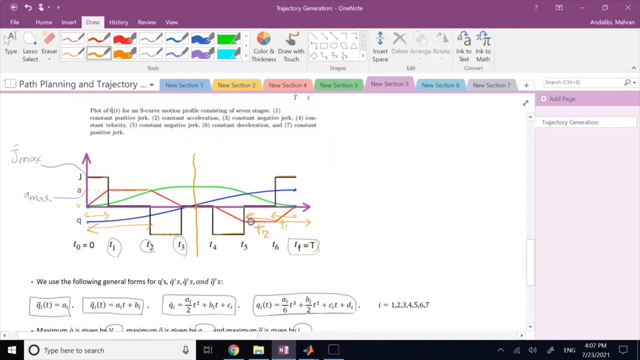 b1 is also zero because your initial acceleration is zero and your b2 and b6 are equal to a max and negative a max. and that comes from this plot here. this is the b2 value and this is the b6 value, the accelerations in second and sixth part- and they are equal to a max, as you can see here. and 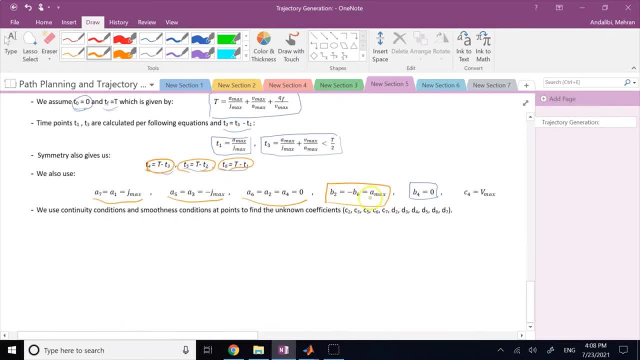 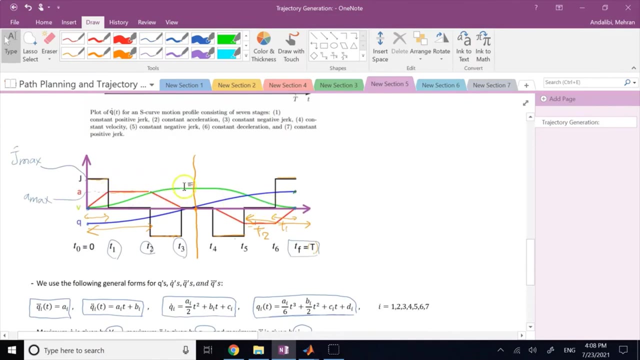 here. this is negative a max which you can see. so you have um. if you can see, you have four of your b's, correct. you have four of your b's. your c4 is also um, the velocity in the center part, and that is your v max, correct? so we know that one as well. 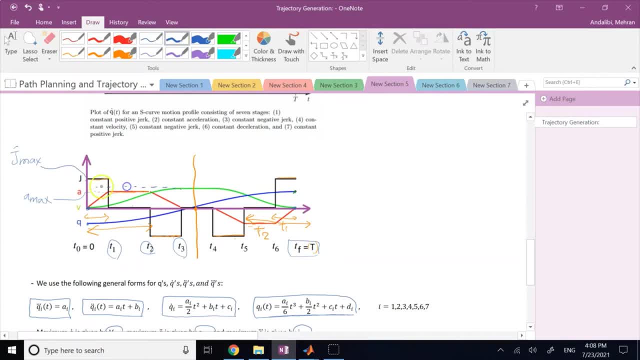 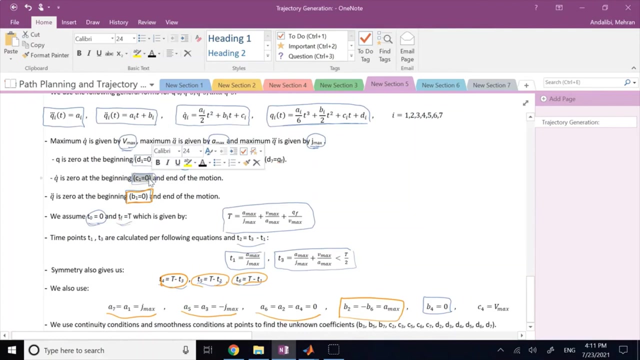 so if we project that here, this guy is also v max, right. so the velocity also for the center portion is v max. so that is equal to uh c number, uh four. okay, so your c number four is given. also c number one is given because that's the initial velocity and since the initial angle is zero, it means d1 is given. 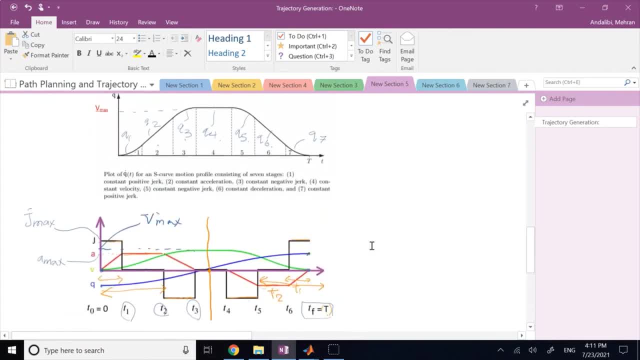 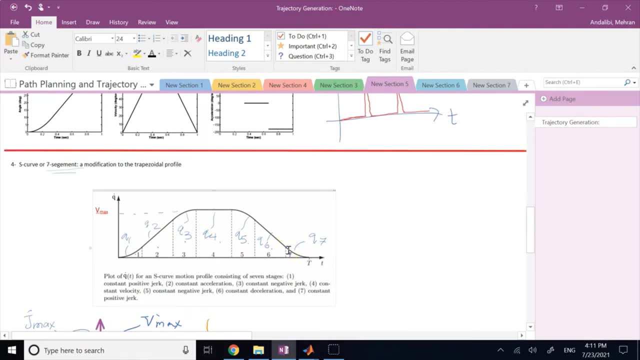 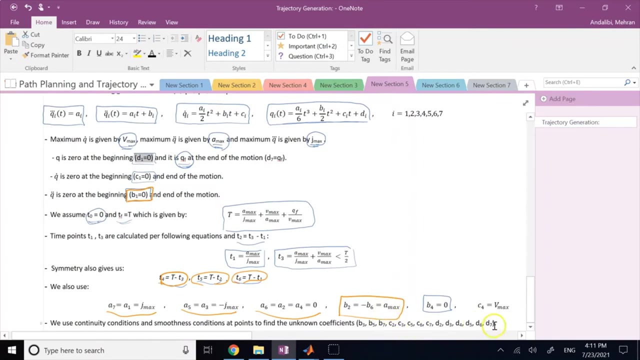 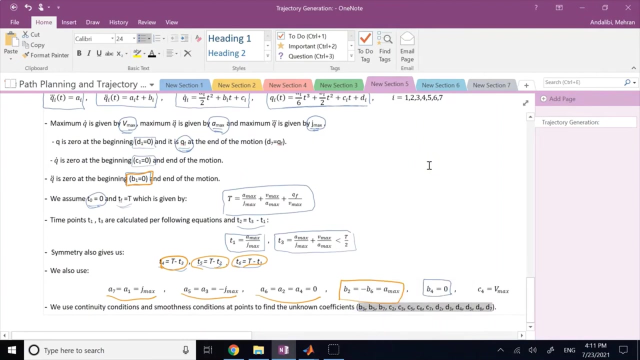 so, out of these, uh, seven times four out of the um 28 coefficients that we have, several of them are given here and the rest of them which you can see over here, these guys you have to find, which are about 14 of them. okay, so 14 coefficients you have to find, but it's not at all hard, i'll show you. 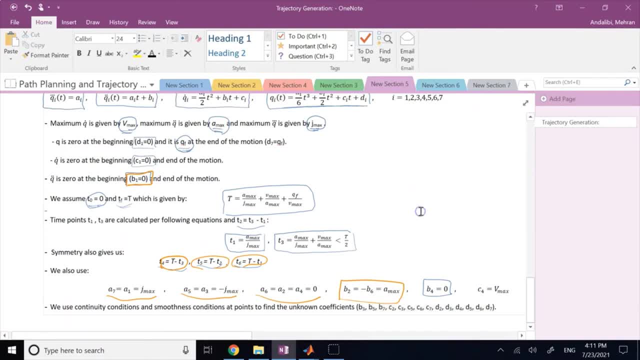 uh, first of all, 14 left. why 14? and do i have enough equation to get it? well, a's are all gone and some b's and some d's and bcds are gone, so 14 are left. but do i have enough equation? well, the matter of fact is yes, i do. 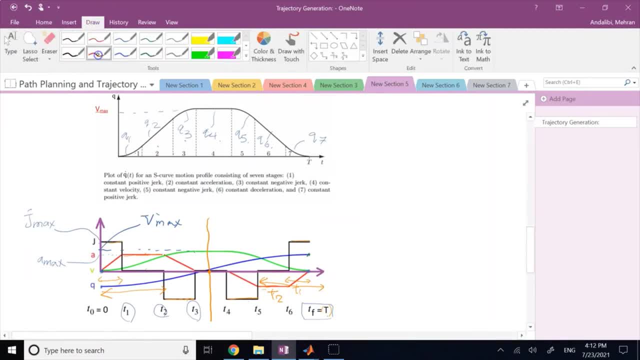 at each one of these intersection points, which is t1, t2, t3, t4, t5 and t6. not only the q's should have the same number, the q dots should have the same number, as you can see, because your q dot is a smooth function, and your q double dots or a's should have the same number because you see it's. 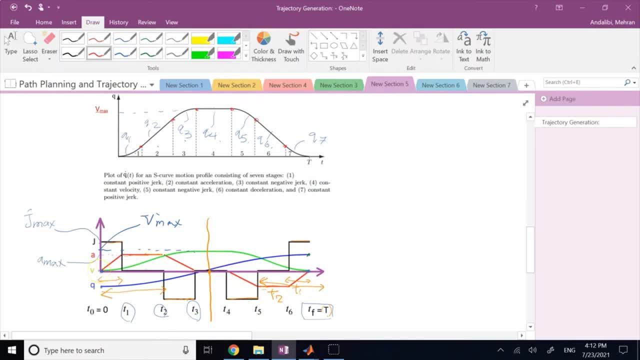 a continuous function. Okay, so at t equal ti where i is, from 1 all the way to 6.. Okay, it's not the first one, it's not the last one. At each t equal ti, I should have three conditions. 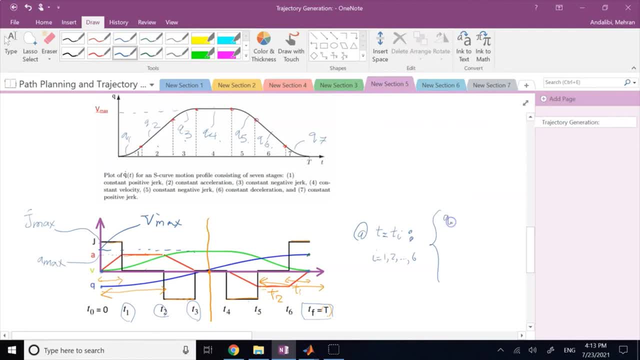 Q i at that ti should be the same as Q i plus 1 at that ti. It's the continuity in Q, And then for smoothness at that point I should have: Q i dot at ti is equal to Q i plus 1 dot at ti. 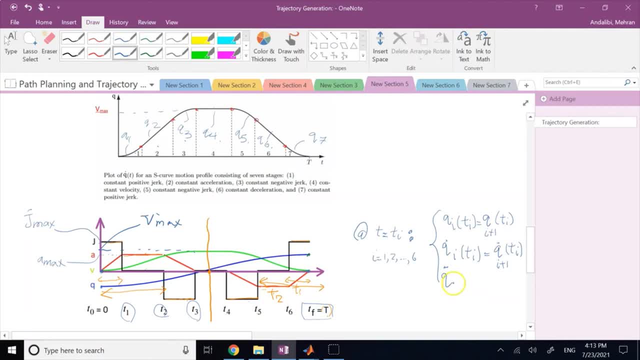 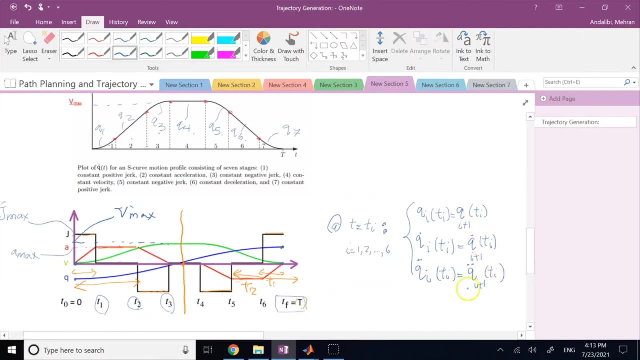 And then Q double dot I at ti should be the same as Q double dot i plus 1 at that ti. Okay, and you might say: well, how many conditions are these? Well, there are three of them, and there are six points. 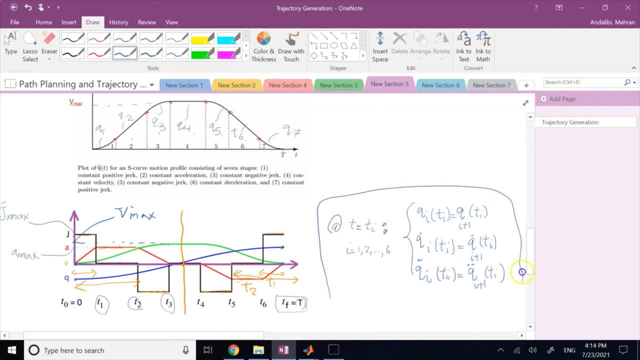 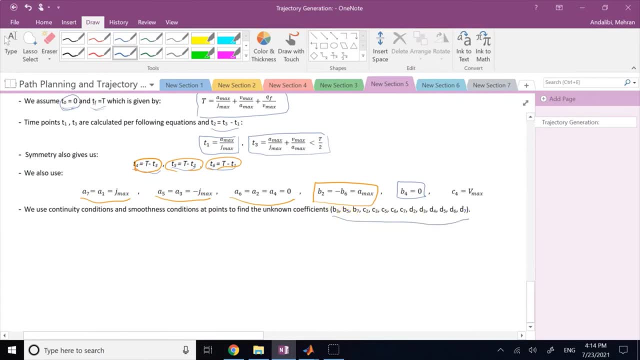 So it's 18 conditions. These are 18 conditions, But you might say: well, I only have 14 parameters. If I have 14 parameters to find here and I have 18 conditions, will I somewhere get into problem, because I have more equations than unknowns. 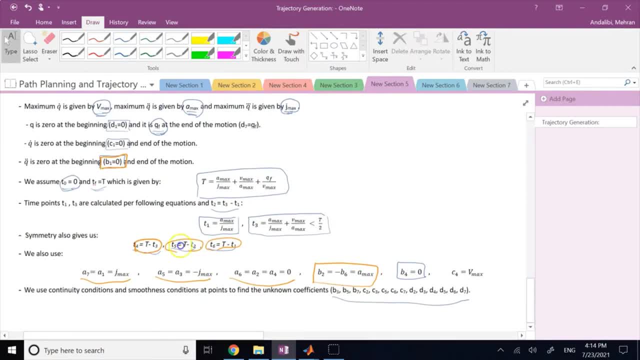 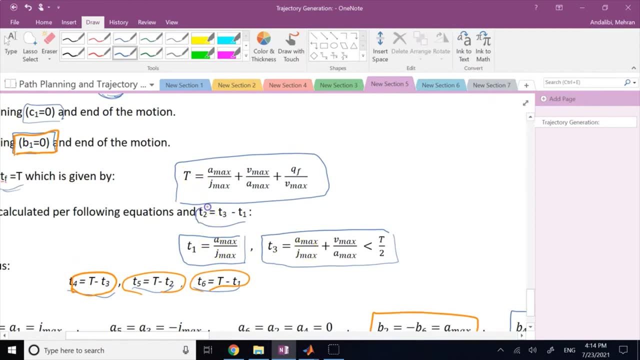 And the answer is no. If you here take a look, I have four formulas for you for capital T, T1,, T2, and T3, which you can see here, these four guys in blue, These four formulas come from. these four formulas come from those four extra. 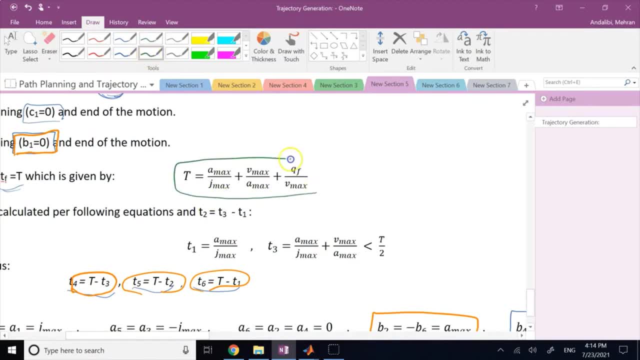 um equations that you have. Okay, So the fact that I could calculate these formulas, they are from the continuity conditions. So, as a matter of fact, you have 18 unknowns, 14 coefficients plus four time values: T1, T2, T3, and cap T. 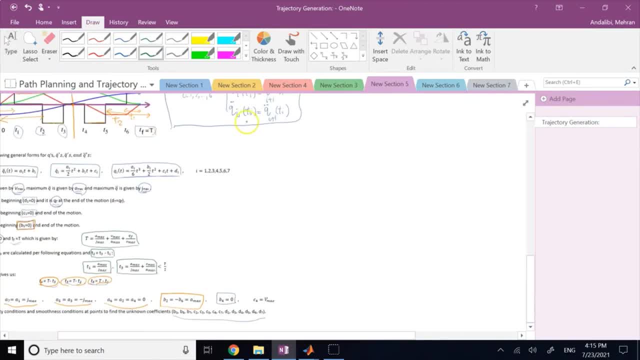 And now you have 18 conditions. from these 18 conditions, You should be able to find all of these. Okay, So you might say: well, how? let me show you, for example, where I got some of these. for example: 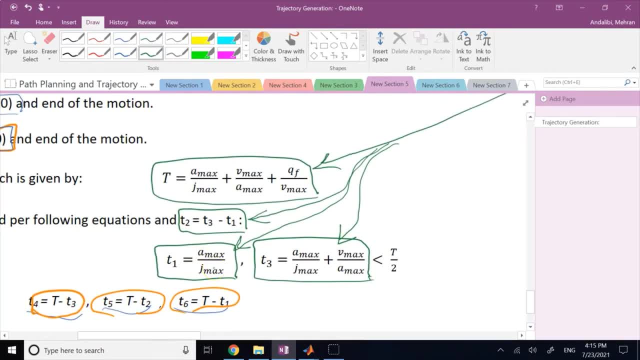 where did I get T1 equal A max over J max? Because I don't want to just give you formula, I want to show you how you can handle this by yourself. So A max over J max, A max over J max is T1.. 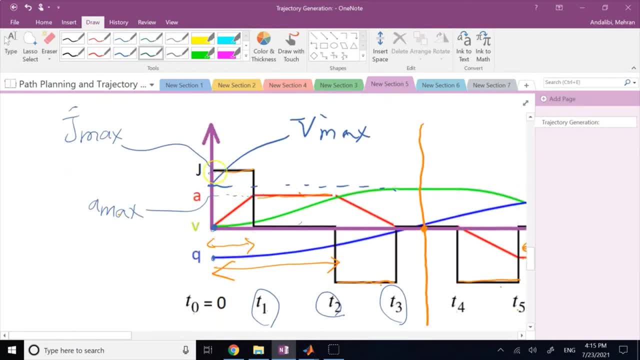 Well, that comes from the first part of the graph. If you see, time goes from zero to T1.. Let me get rid of these. Your time goes from zero to T1 in the first part of the motion, Correct, And then with the constant jerk of J max. 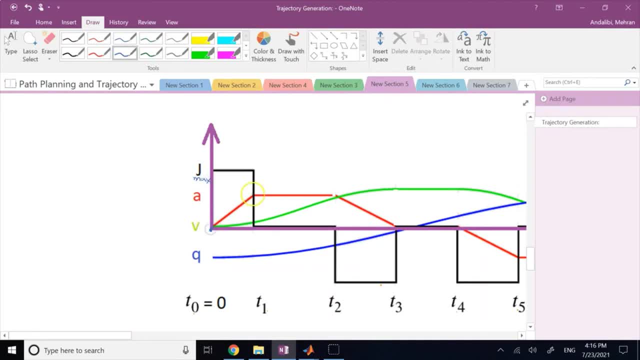 you go from acceleration zero to acceleration A max And since the relation for the acceleration is linear, clearly this A max, the height, is equal to the slope. This J max here is the slope of the line times the time that you had, which is T1.. 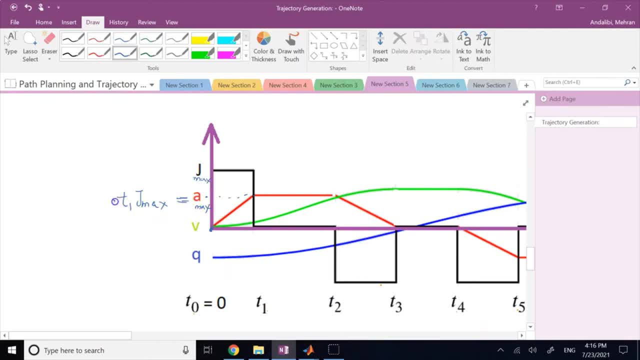 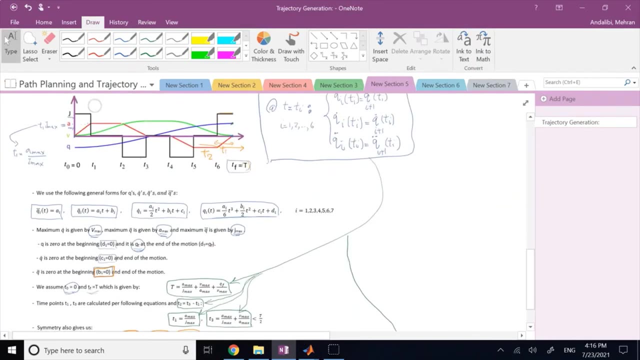 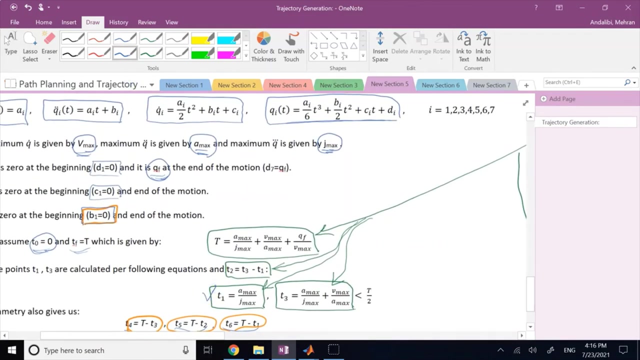 So you see, T1, J max is equal to A max. So from here, T1 is what It is: A max divided by J max, Correct, Which you can see over here, Right. Where does the other formula come from? 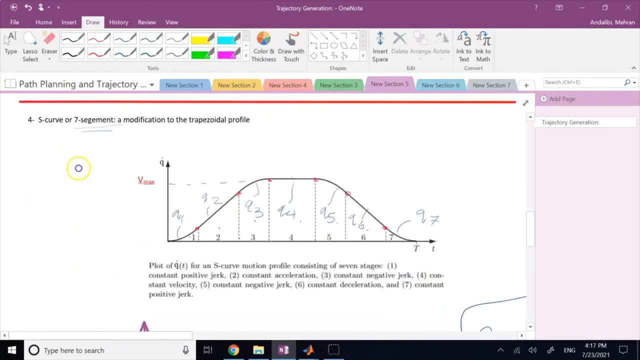 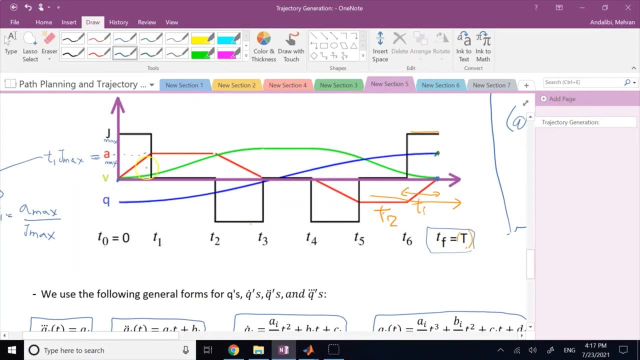 T3,, for example. T3 comes from what? Well, for T3,. let's go take a look. T3 is the end of the third, The third part, which is you go through one full trapezoid of acceleration, as you can see. 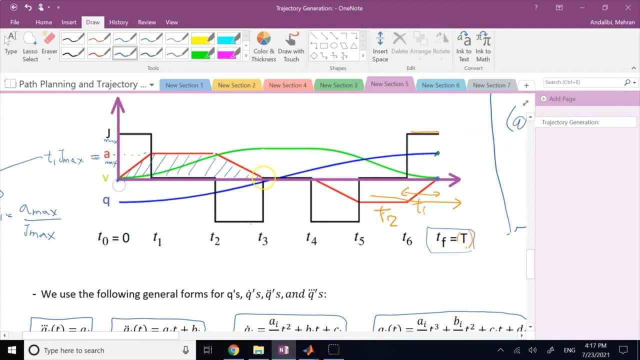 Where, during this full trapezoid which goes from zero to T3, you go from zero speed to what? To the V max speed. Correct, This is what V max. So your speed changes from zero to V max And that's because of this profile trapezoid. 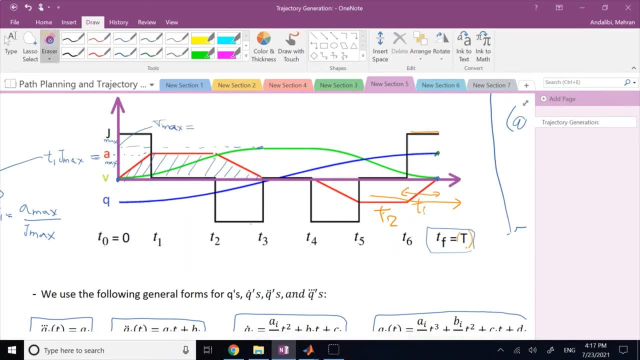 This is the trapezoid of acceleration And you know the change in delta V in general, which is V max minus zero. Delta V is equal to what Integral of ADT? The integral of ADT means the area under the curve of A versus time. 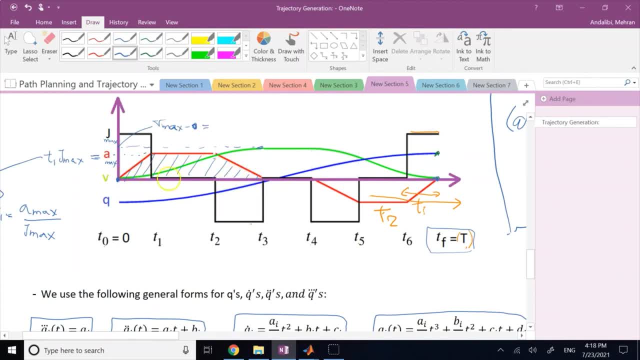 So it's the area of this trapezoid. And how much is it? You know, the area of a trapezoid is the average of the two base times height. Well, the bottom base is T3.. The top base is T2 minus T1.. 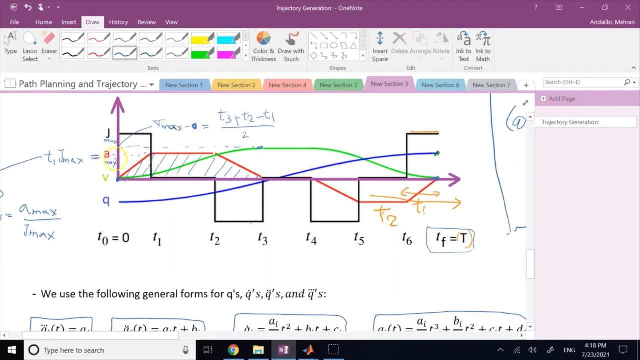 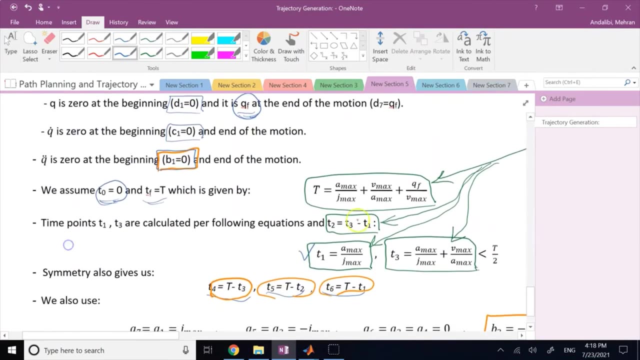 The average of these two then times the height, which is what A max Correct. So this is the formula you have. Now, before I can solve this for T3, I need another relation which I have over here, And that is: T2 is equal to T3 minus T1. 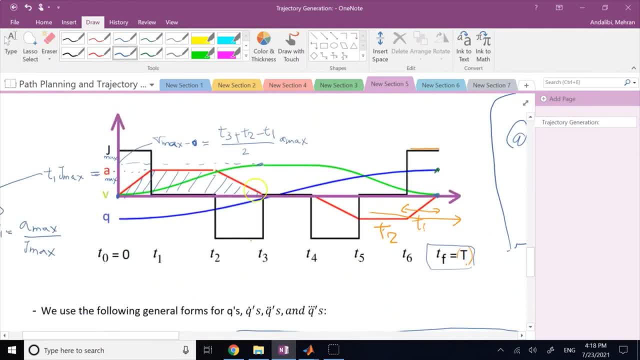 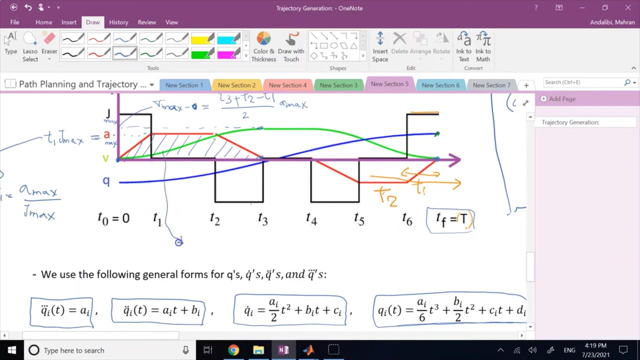 Where do I get this one from? Well, that comes from the fact that your acceleration goes from what? Zero to zero during this trapezoidal motion, And you know the change in acceleration during the very same time, between zero to T3, the change in acceleration, as you know. 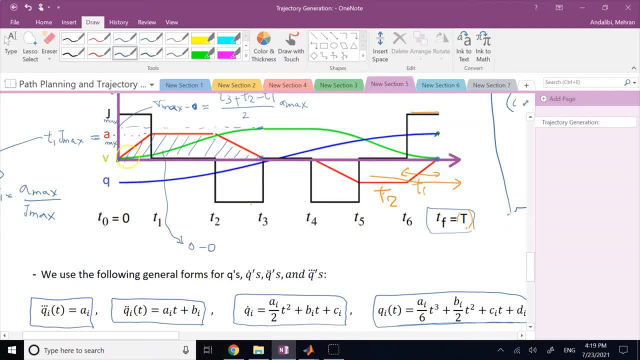 which is zero minus zero correct final value minus initial value. So it comes from the integral under the area of the jerk, which is this area here in green. And what is this area? Well, it is T1 times Jmax. 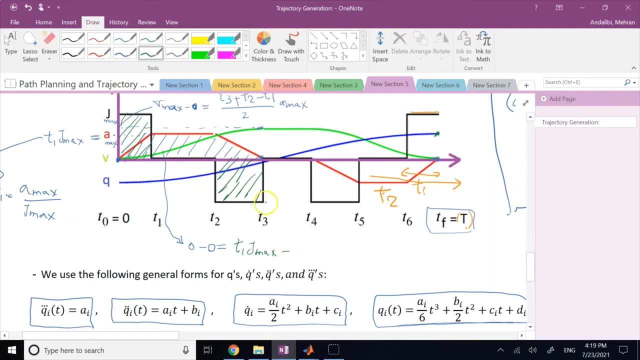 And plus what Or minus? actually, Minus T3, minus T2 times Jmax, correct? Because if you remember, if this is positive Jmax, I said this value here is what Negative Jmax. I don't have to choose it that way. 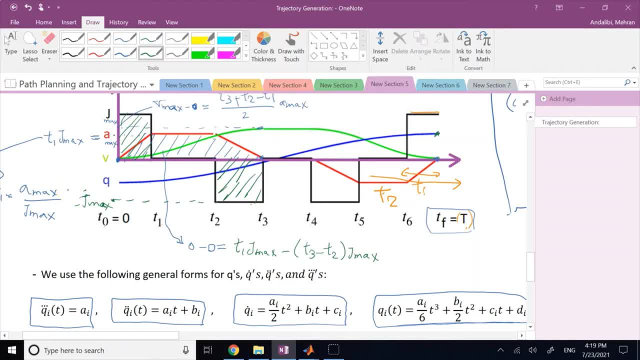 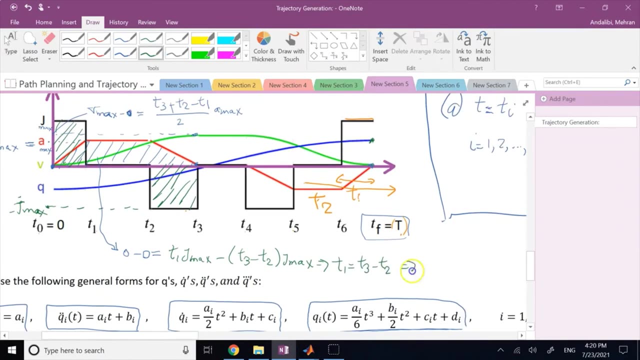 but if you do, it makes life a lot easier, makes your formulas a lot better. So clearly, from here, you see what, Since it's zero, from here your T1 has to be the same as T3 minus T2.. And from here, clearly, your T2 is what? 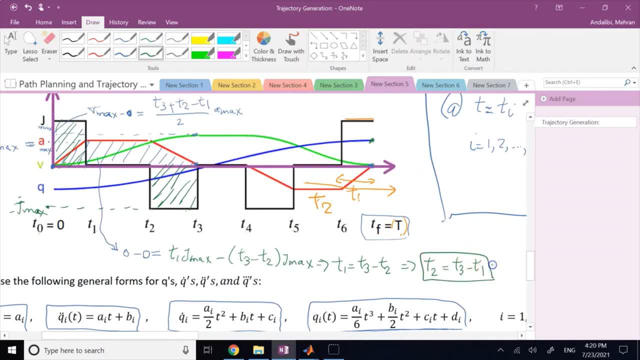 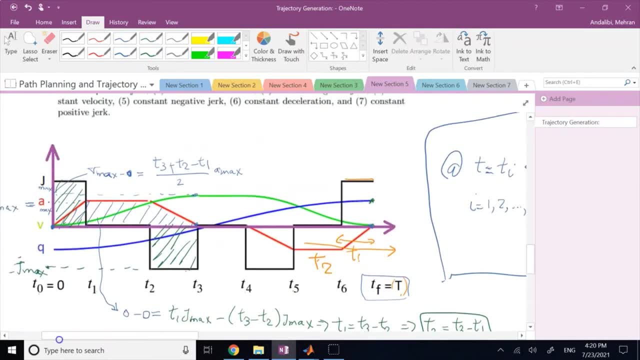 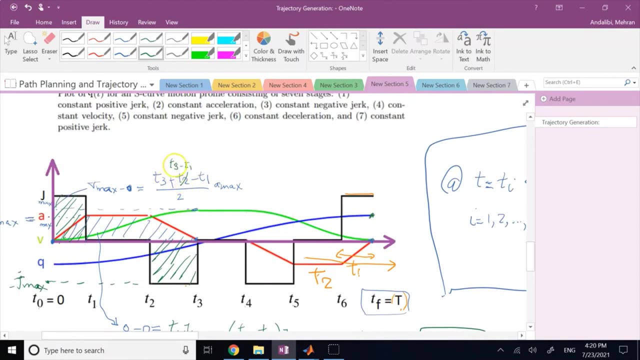 T3 minus T1.. So that's where I got this formula from. Now that I know T2, I plug it into this bottom top formula. So T2 is T3 minus T1.. So now, if you look, you have two T3s negative, two T1s divided by two. 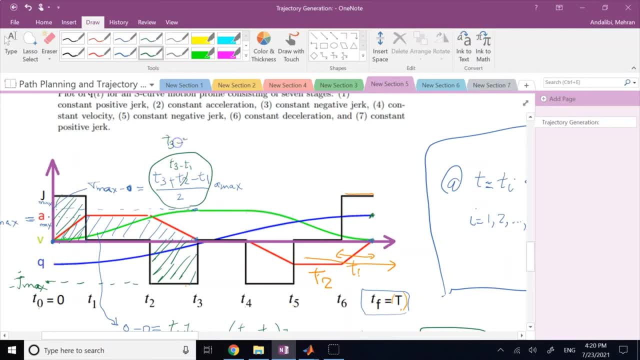 So this whole thing can be simply simplified. as T3 minus T1 times Amax is Vmax, Therefore your T3 is going to be Vmax divided by Amax. And then what Plus T1,? take T1 to the other side. 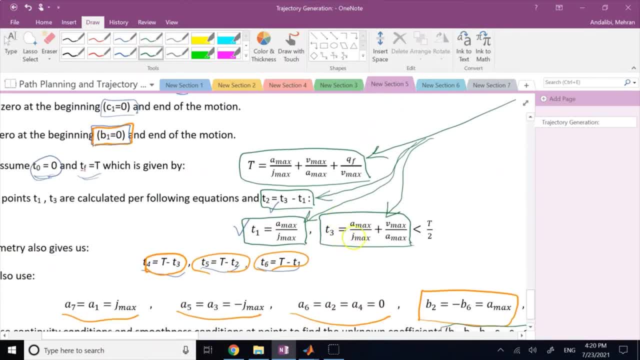 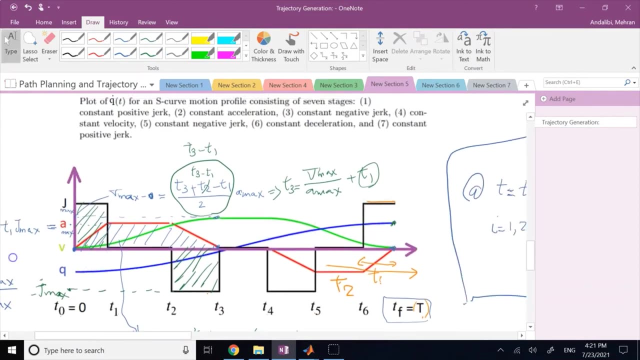 Right, And that is this formula here. Well, let's see, I said Amax divided by Vmax, divided by Amax plus T1.. But T1 itself, if you remember, T1 is what? Amax over Jmax. 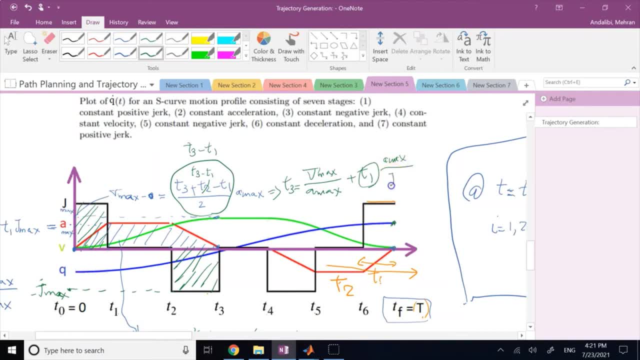 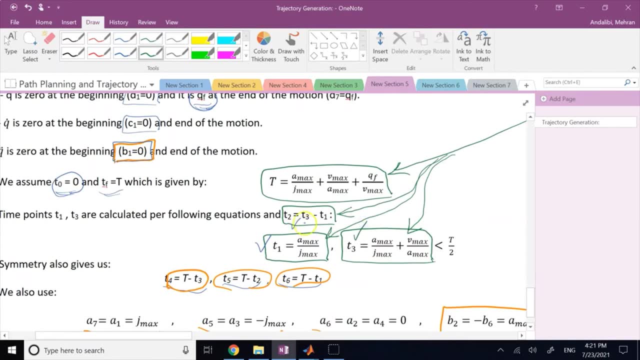 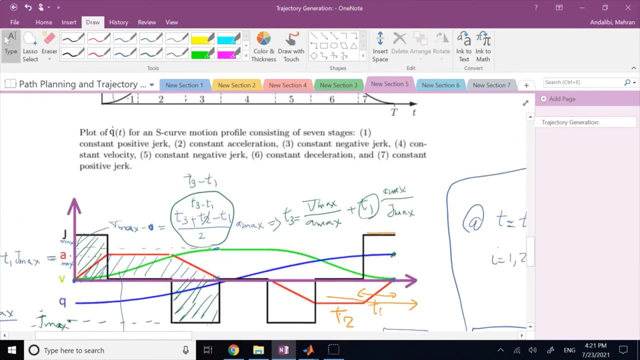 So I just replaced it. That's this formula. So you see how I got these three formulas for T1, T2 and T3? Yes, So I'm using continuity conditions and the fact that I should go from one area to another. 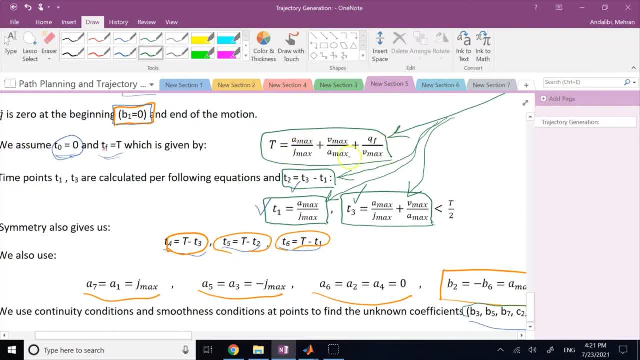 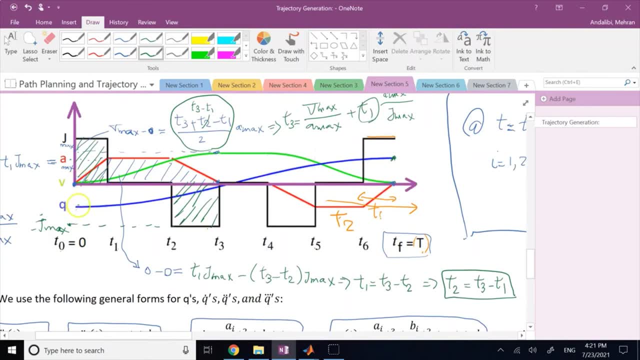 Now, what is the last one? this formula for capital T. Where does that come from? Well, that comes from the change in the angle. You go from initial angle that we chose to be zero, unlike this case where it starts from a negative Q. 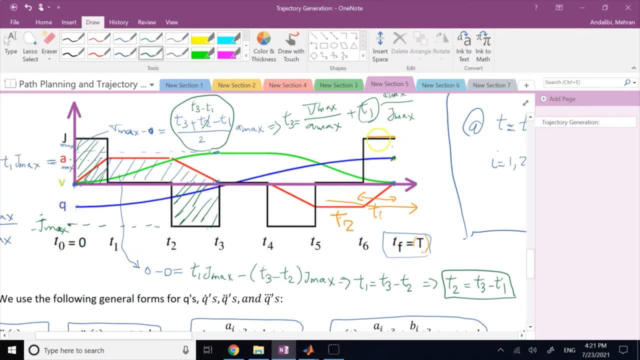 We start from zero Q and go all the way to some Q final And the change in the angle is area under the curve of what? Under the curve of velocity Right. So if I can find the area under the velocity curve, that is Q final minus Q initial. 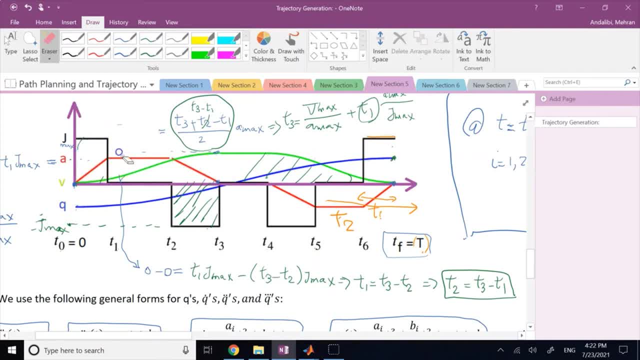 Now how can I do that? So to do that, I need to do a little bit of clean up, if you don't mind, because it's just too crazy here. So I will do just very fast cleaning here so you can see when I'm plotting something for you. 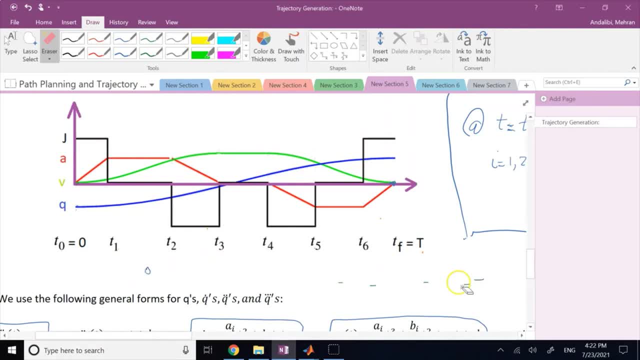 OK, good, Now what? Now, what's the area under the green curve? So it is actually a trapezoid, but you have to pay attention. So what I will do? I will connect this point where the linear velocity, the constant velocity, starts, to the beginning. 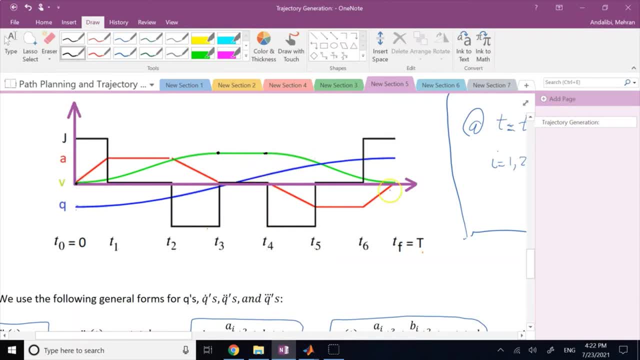 And I also connect the end of the point T4 to T7.. If I connect them with two lines, let me see if I can connect them for you. OK, there we go. This is one and this is the other one. OK, because of the symmetry. 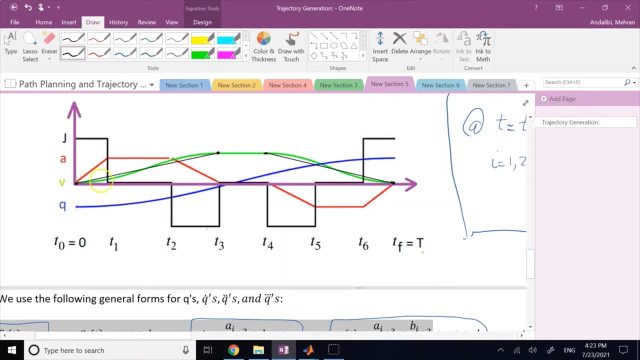 the area of this between the green line and the black, the green curve and the black line, which is this area here. So this area is where the line is bigger than the green curve. This area here is a different color. This area here in red is where the green curve is bigger. 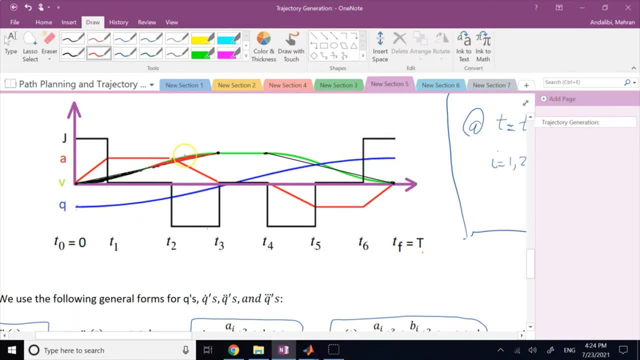 Than the light. But because of symmetry, the green area is exactly the same as the black area And similarly here. if I do the same thing here in the blue area again, the velocity is bigger than the actual velocity curve is bigger than the black. 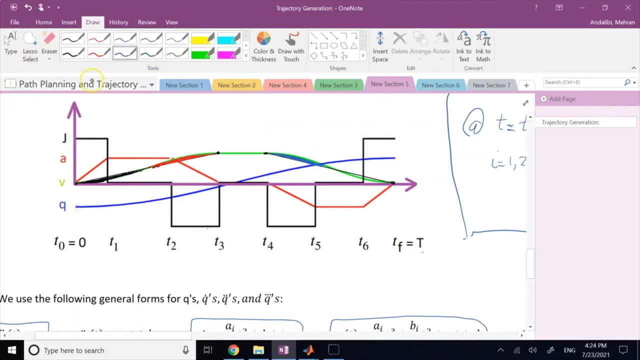 lines, and here in the T5 to T7. You have the line to be bigger than The actual velocity profile. but again, the blue and the green areas are the same. So the area under the trapezoid, really the area under this trapezoid, 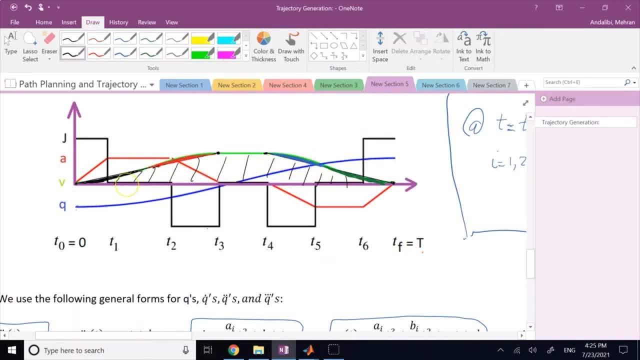 is the exact same thing as the area under the actual velocity V. And what is this area? Well, the area here which is, as I said, area under velocity and is equal to Q final minus Q initial, By the way, your Q initial here. 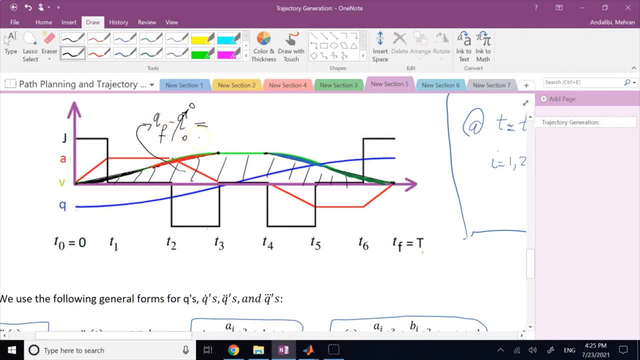 I assume zero, but you can choose it to be nonzero. This is equal to what The area of a trapezoid which is the big base, which is capital T, plus the middle one, which is T4 minus T3.. 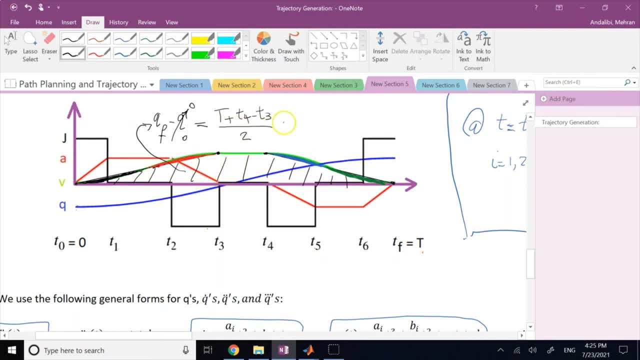 Divided by two and then times the height, The height is Vmax, Right, You know, this area here is: This is Vmax, But if you remember, T4 is T minus T3, right, Or is it here? 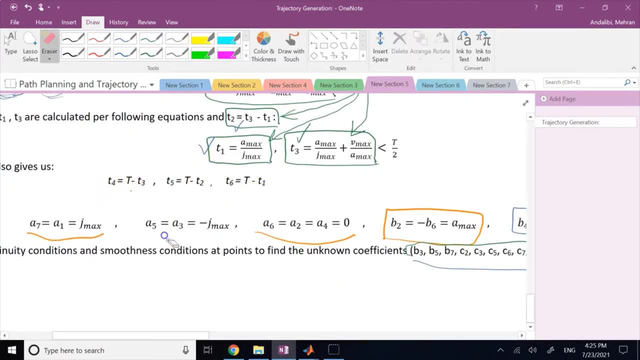 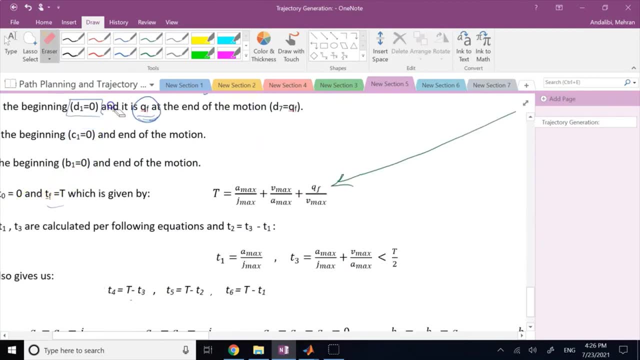 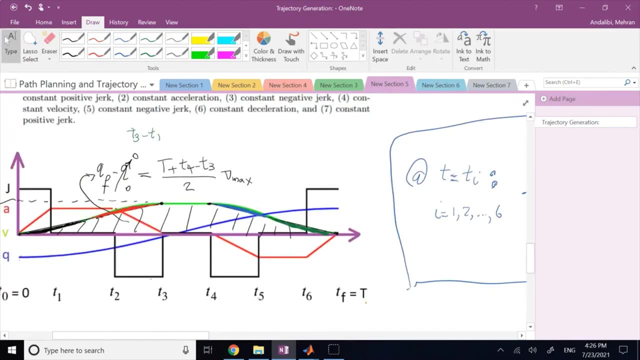 T4 is T minus T3. Therefore, I can replace it up there, so let's go ahead and replace it. Just trying to do a little bit of cleanup. I just made it too busy here, So if I replace it, this is going to be T minus T3. 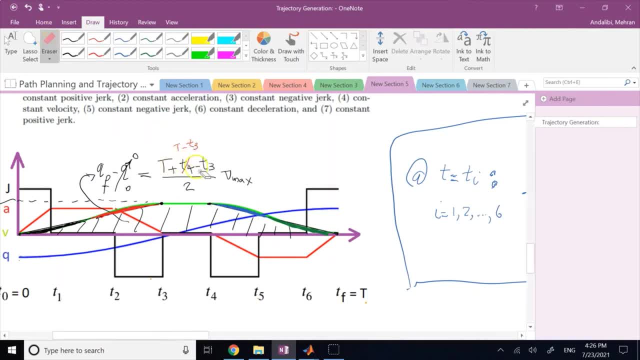 And now, if you look again, you have two cap T's minus two T3's divided by two. So this whole thing can be written simply as T minus T3.. Right, And from here you see your T is going to be. 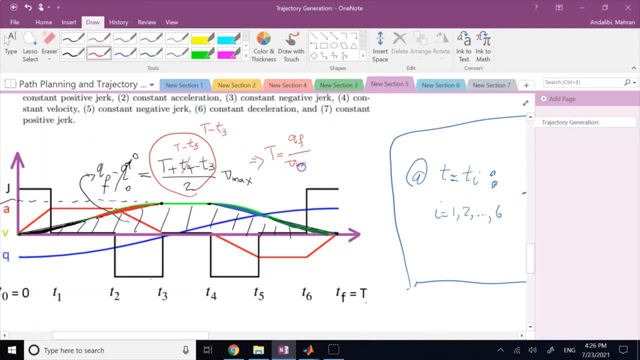 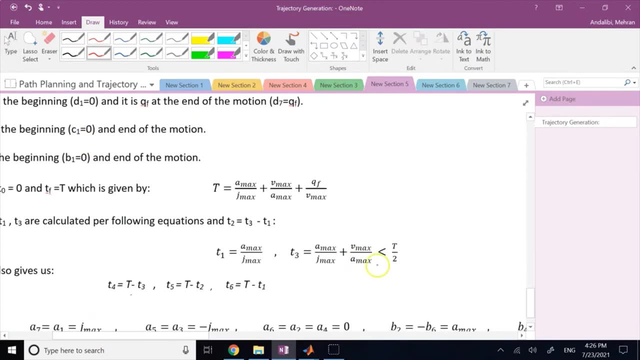 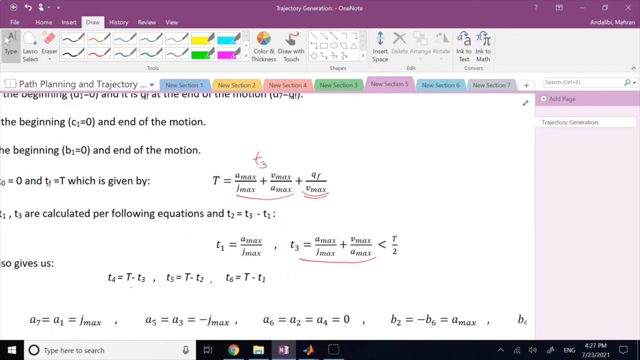 Q final over Vmax, and then plus T3.. And T3, if you replace it from what we had in the past, This is T3. And this is that Q final over Vmax which you found here Correct, So it exactly gives you what you wanted. 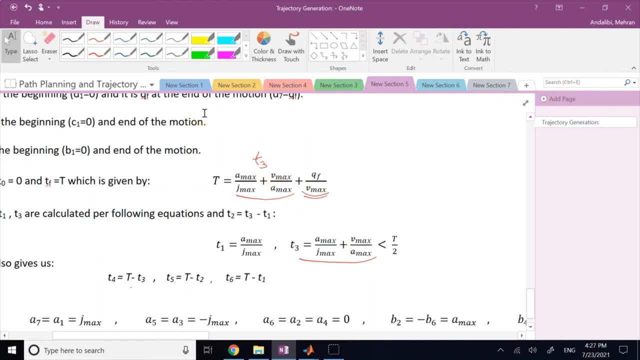 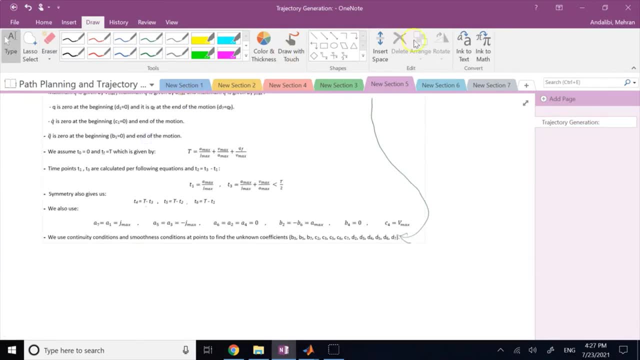 Right. So you see, I'm using these continuity conditions and that gives me the value for this four time points. Now that I got my four time points out, of those 18 equations that I had up here, four of them are gone. I'm down to 14.. 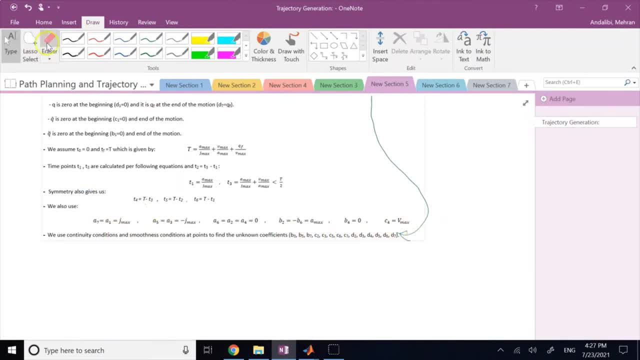 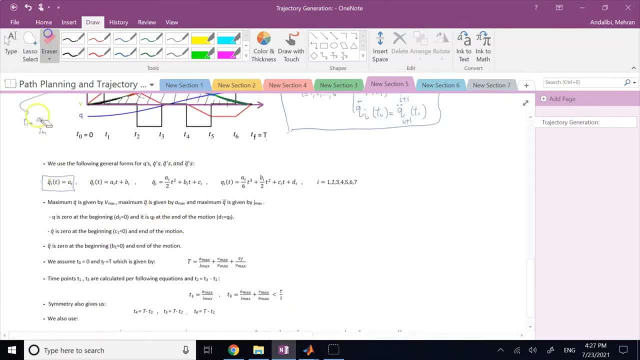 And guess what? I have 14 coefficients here to find. And it's just coming from those equality conditions. right, The Q's are the same, Q dots are the same, Q double dots are the same at the share points. intersection points. 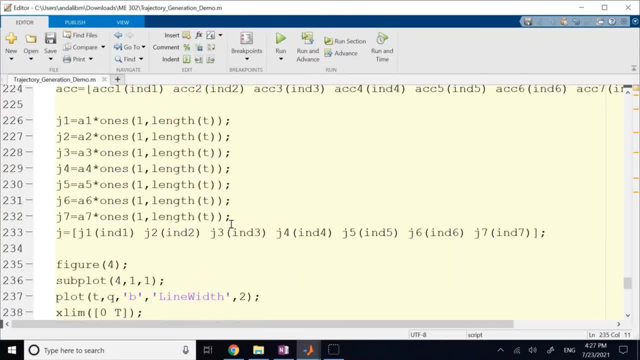 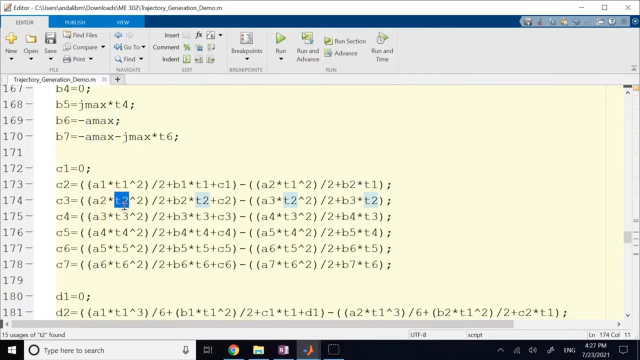 And here, if you go and look at my math lab code, I'm using the same thing here. So when I have my A's and my B's, when I want to calculate my C's, let's say, or D's, I'm just calculating the value of QI at the TI subtracted from QI plus one. 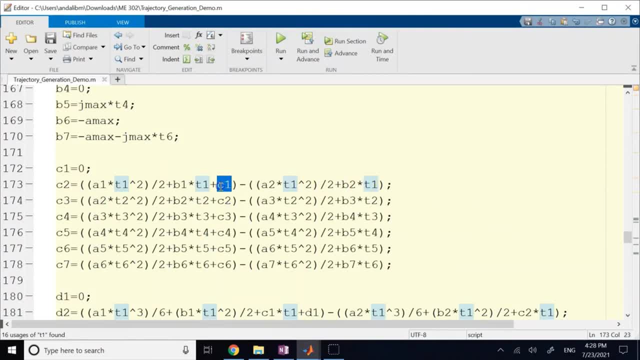 at the TI, except for the parameter that I'm trying to choose, And then that gives me the unknown. So if you bring this whole thing, for example, if you bring this whole thing to this side and add it to C2, it means exactly what. 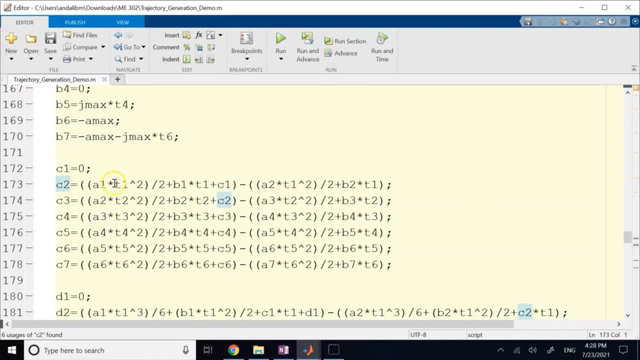 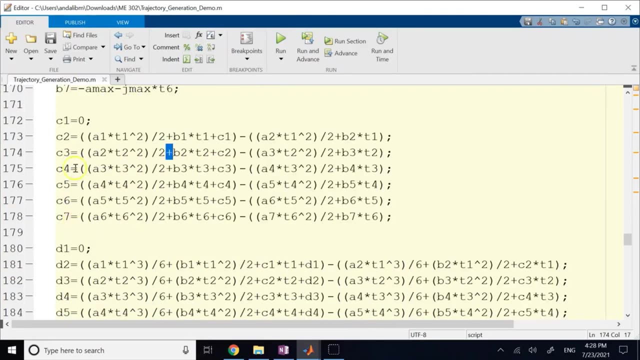 It means that Q1 dot at T1 is the same as Q2 dot at T1.. If you look at this, this is going to be: Q3 dot at T2 is the same as Q2 dot at T2.. And since everything here is known, through these recursive equations I can get: 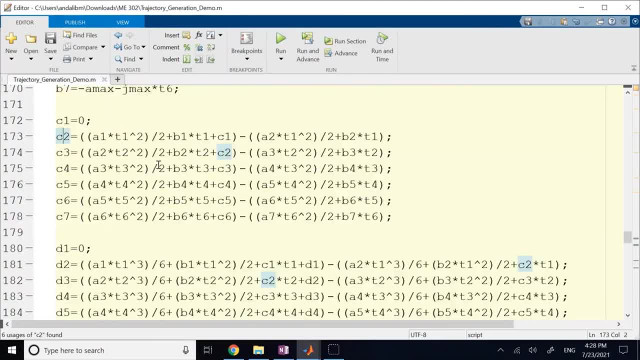 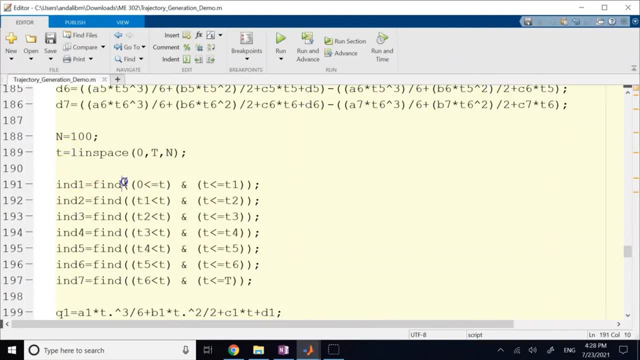 all of my C's, all of my B's that are missing. My A's and B's are good And here I have seven parts of the segment, So I need to divide my whole time point into seven areas, which falls within one of the ranges. 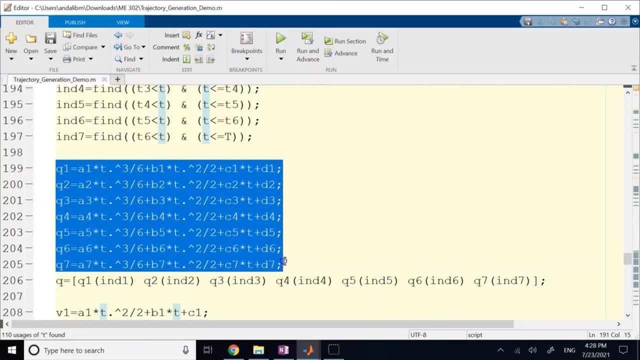 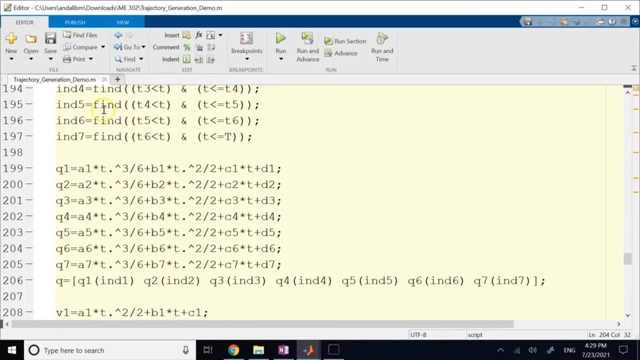 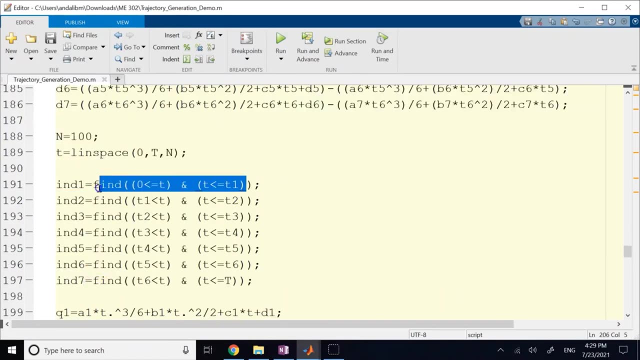 And then when I form my Q's based on those cubic formulas where some of the coefficients are zero, then because I have those indexes, I can limit the data in Q1 to only the Q1 where T falls in this region. So I say Q1 of index one. 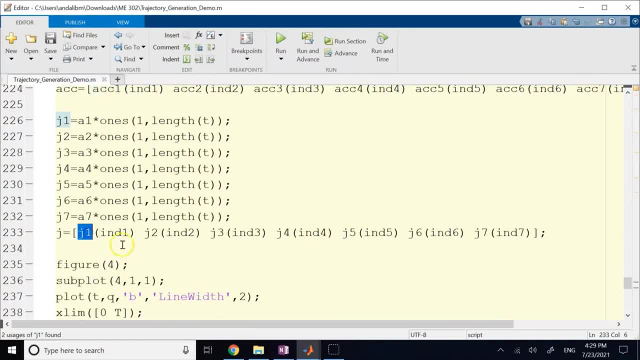 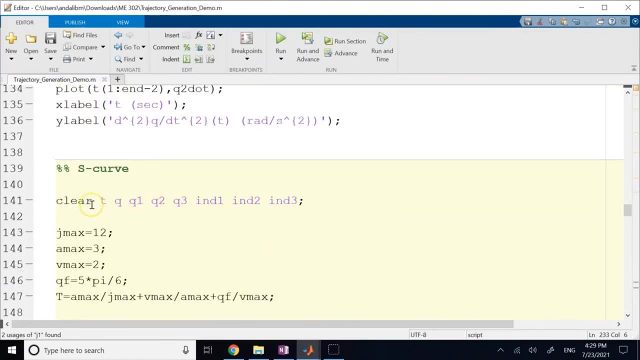 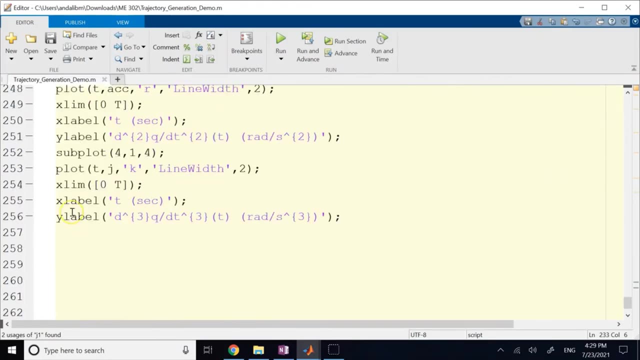 The same thing I do for velocity, for acceleration and for jerk, And here if I run this for you. So here you see, I wrote a bunch of code. I started from, you see line 141, and it went to 256. 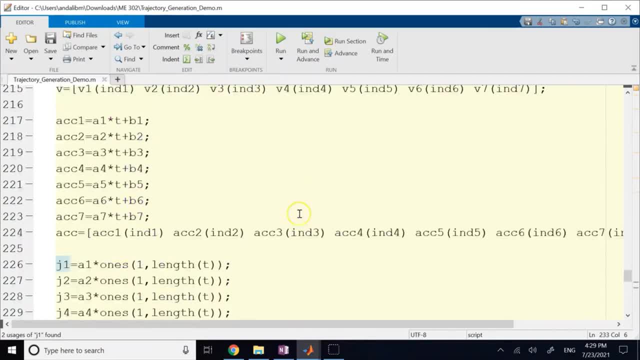 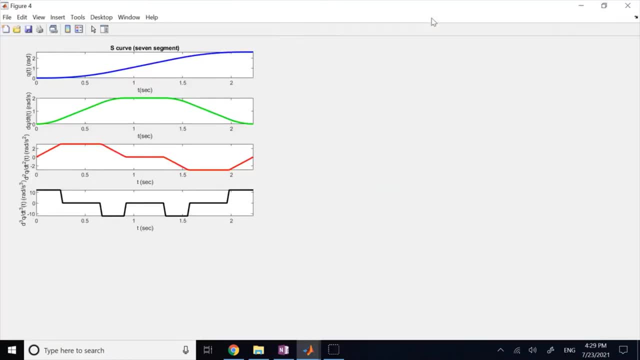 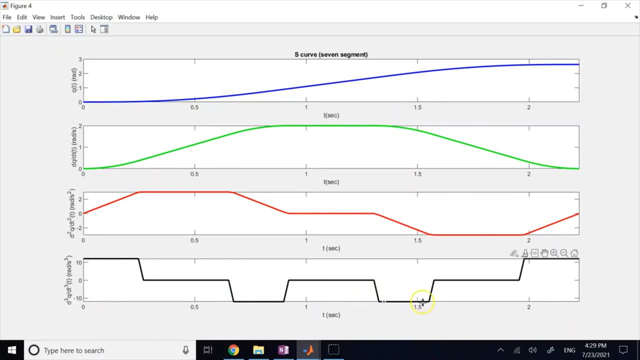 With the spaces, it's probably around 120 lines of code, But here, if I run it for you, you can see the result Right. so you see: constant jerk, zero, jerk, constant jerk, zero, jerk, constant jerk zero, jerk positive jerk max. 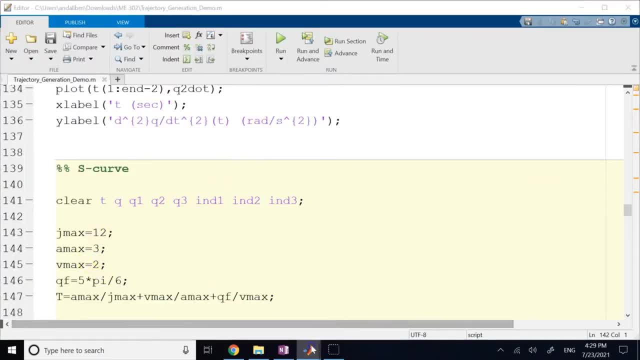 Here your jerk max is 12 and you can see the number here is 12 also. Then your max velocity is three and your max acceleration is three. max velocity is two. So you see, your max velocity is two, your max acceleration is three. 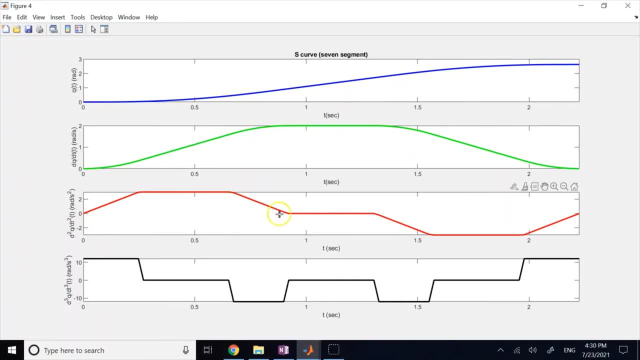 You see linear increase, constant linear decrease, constant linear decrease, constant linear increase. go back to zero. This is your nice S curve for velocity. And finally, this is your Q, going from Q initial, which is zero, all the way to Q final, which is, in this case. 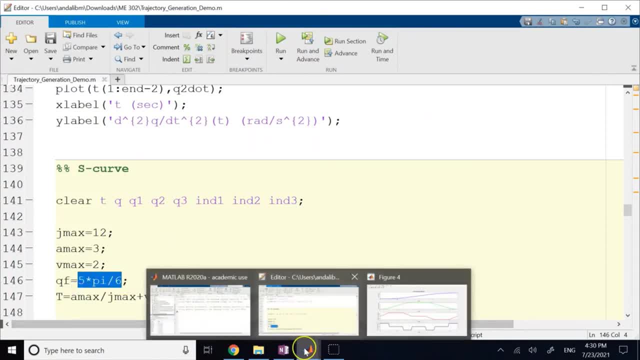 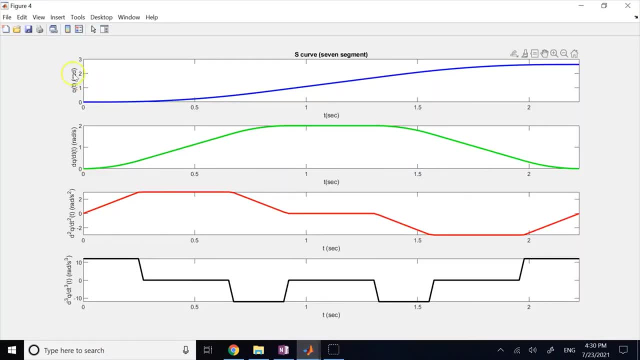 150 degrees right Q final. And if I calculate my Q final here, this 2.61, and that is the number that you see, that this one converged to 2.61.. OK, so it is working perfectly fine. 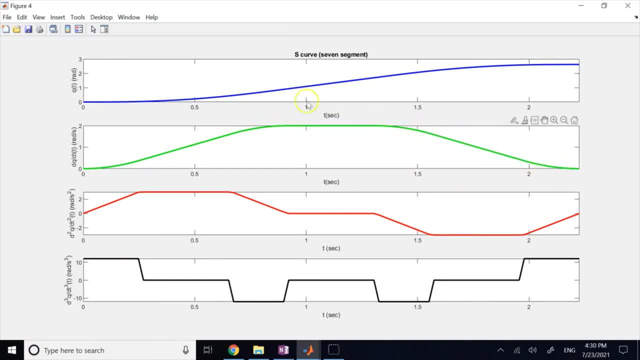 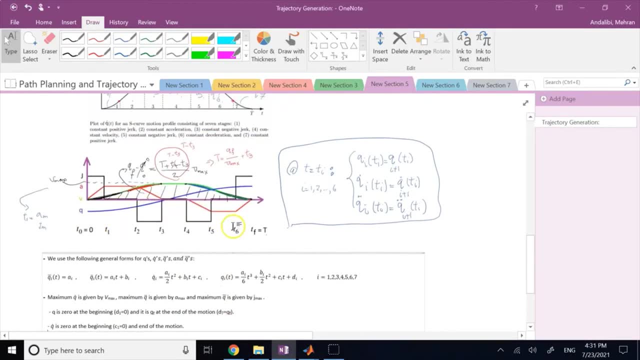 Again, we call this S curve because of the shape of the velocity, or we call it seven segment because it has seven parts, going from T0 to T1 all the way to T6 to T7. There are seven parts of the motion, OK. 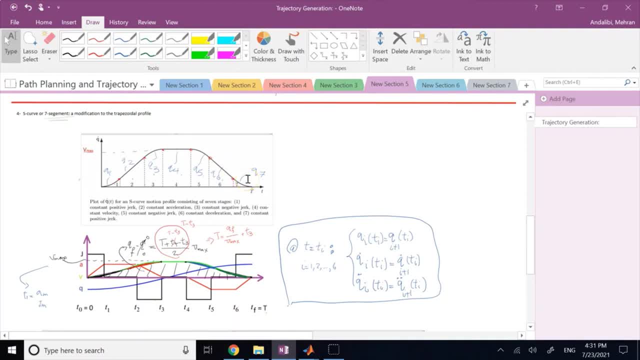 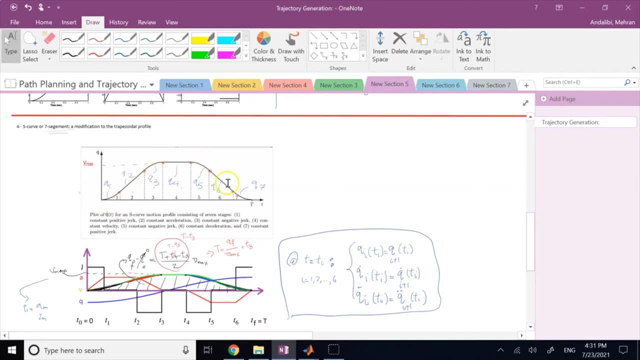 So this is a good choice for robotics applications, Right Where you can start from zero, go to some constant velocity, stay there and then smoothly go back to zero and travel from initial angle to final angle without you exceeding the maximum RPM that your joint can rotate, without you exceeding the maximum.